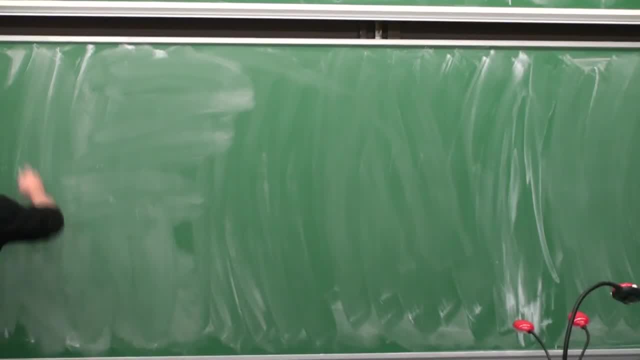 All right, we'll start with the, the sysoid problem, where we defined sysoid in terms of a circle and a line. Maybe our coordinates are like this- x and y with one up there, and then the idea is that we're going to take a line like this: see where it intersects the circle. 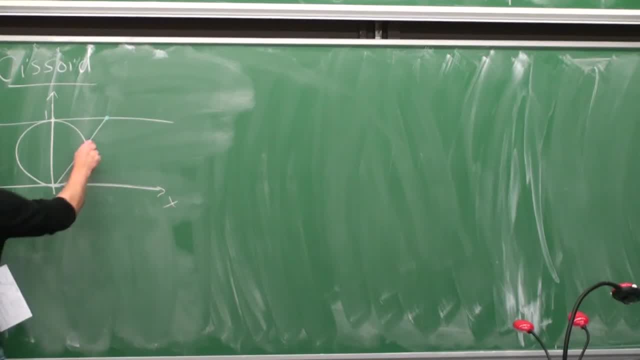 and this other line, and then we're going to translate this vector down here, back to the origin, and see what the locus of this point is, then getting something that looks like this: And the problem is to find a rational parameterization of this sysoid. 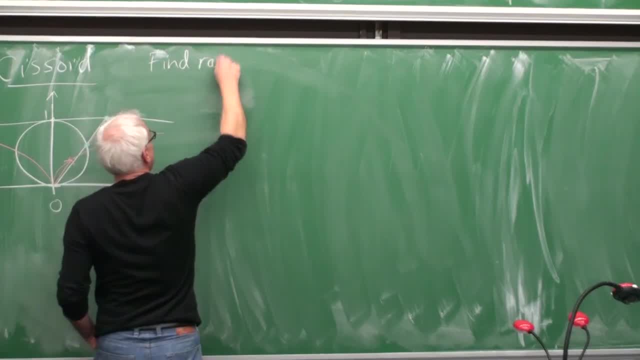 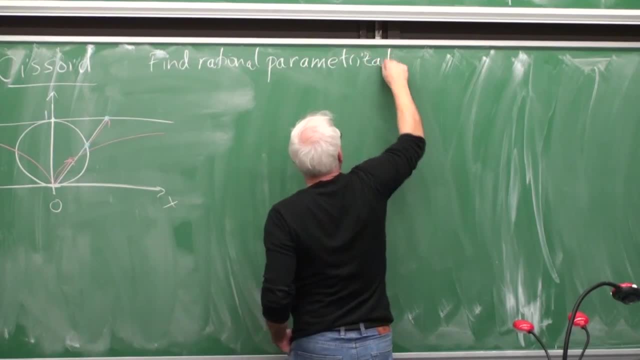 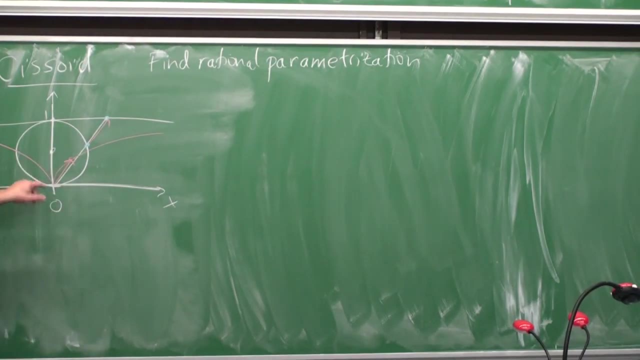 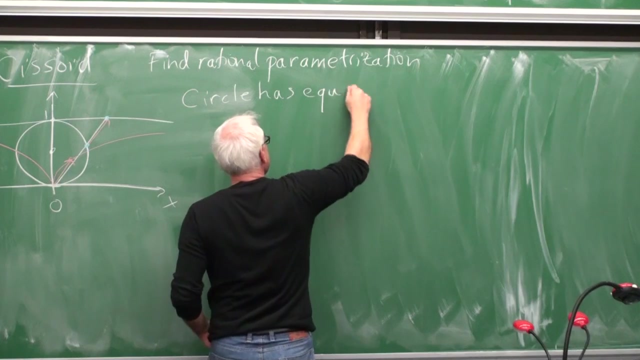 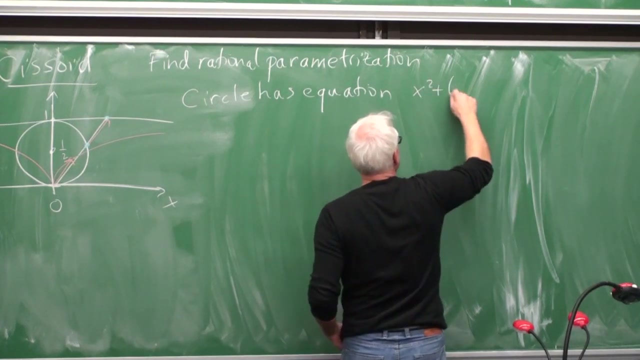 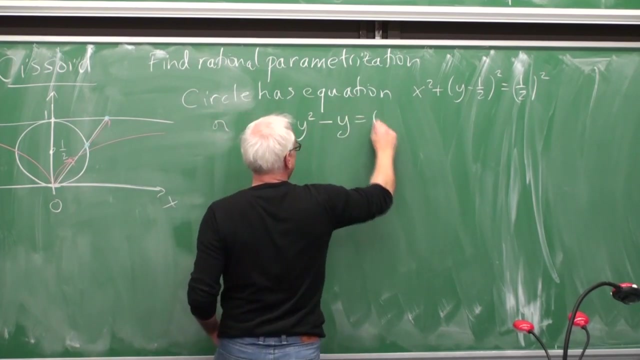 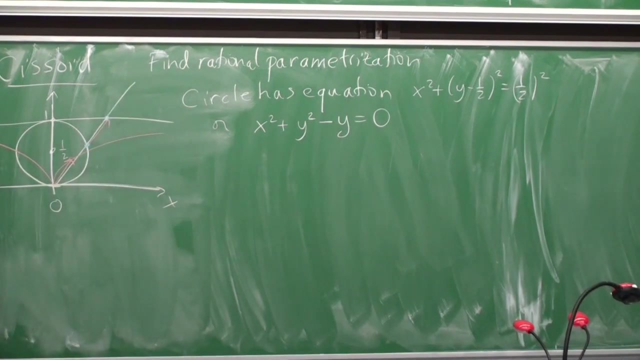 OK, so let's have a look. how might we proceed? Well, first of all, this equation of the circle x squared plus y minus a half squared equals one half squared, or x squared plus y. squared minus y equals zero. And let's have a look at this line that we're using to define the sysoid itself. 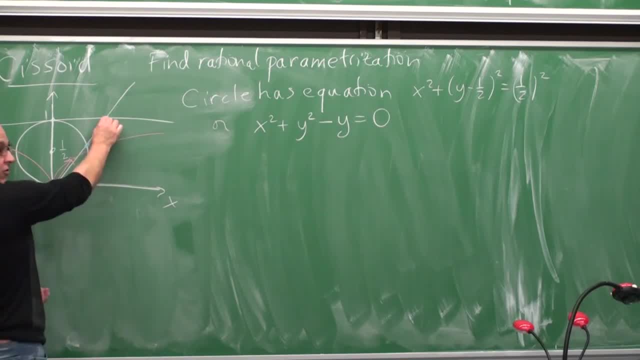 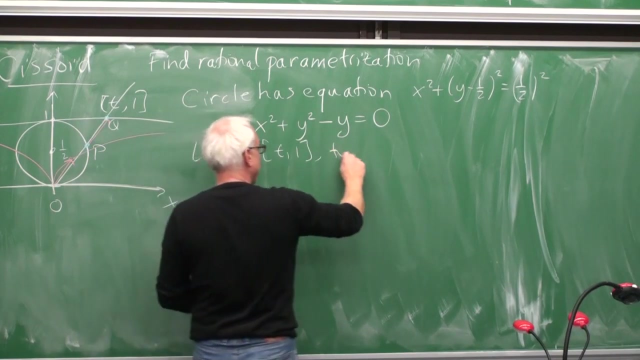 So let's sort of get some control over that line, maybe by thinking about this parameter here. that's the point. say, whose x-coordinate is t and whose y-coordinate is one. So let's call this point p and this point q, so let's let q be the point t1, and to: 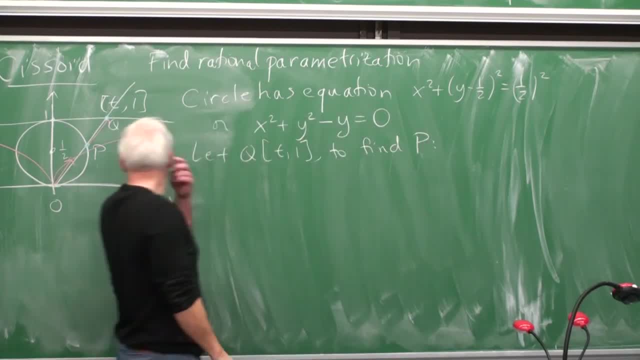 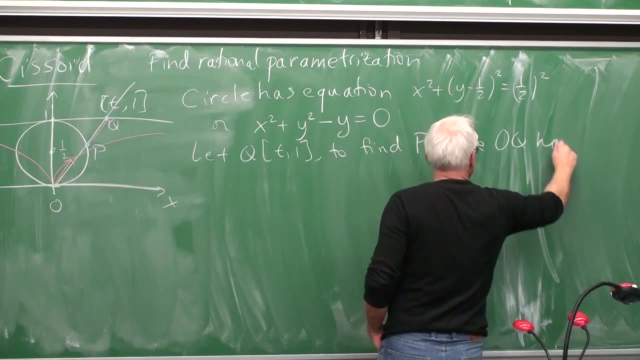 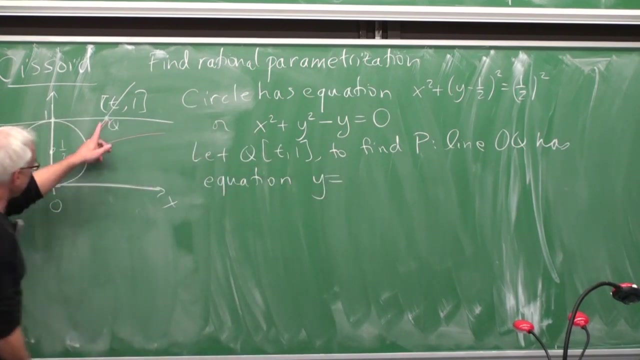 find p. what are we going to do? Well, we want to write down the equation of this line and then see where it meets the circle. So the line oq has equation y equals. well, it's got a slope of t, because that's no. 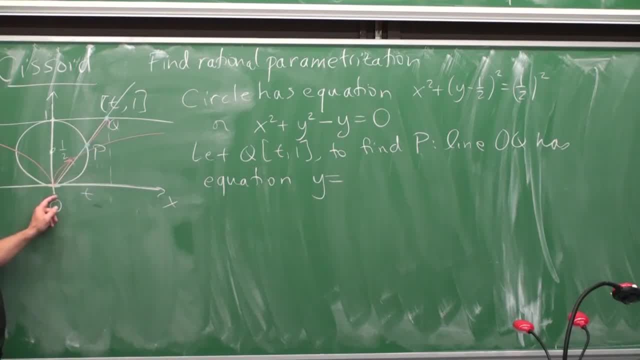 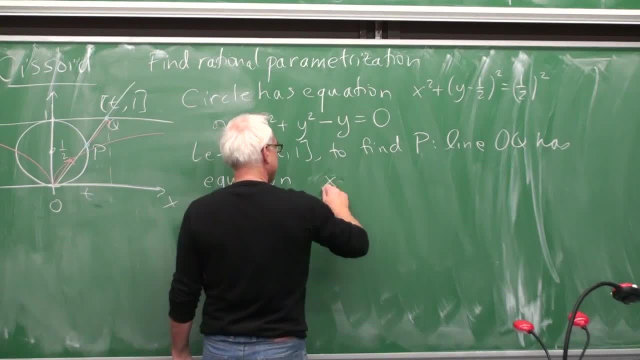 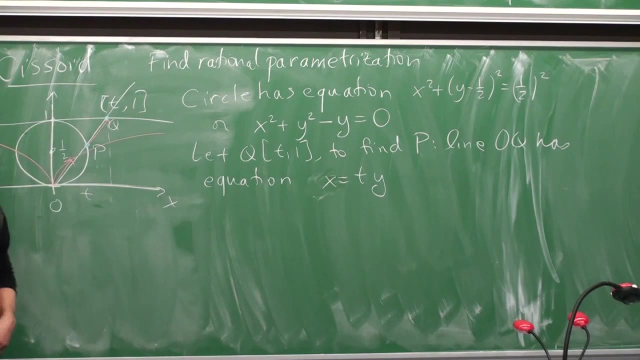 it doesn't. it has a slope of one over t, So the equation maybe we should write it as t, x equals ty. So when y is one, x is t, We don't always have to write an equation of a line in the form y equals mx plus b. 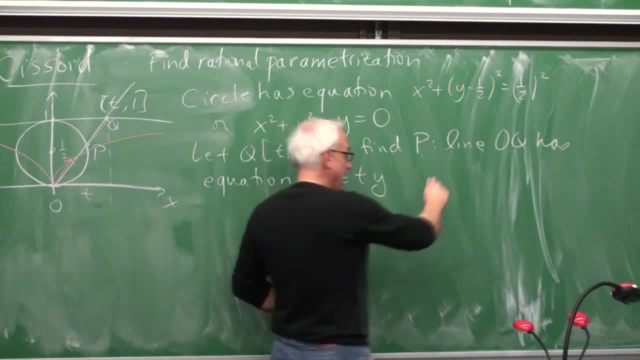 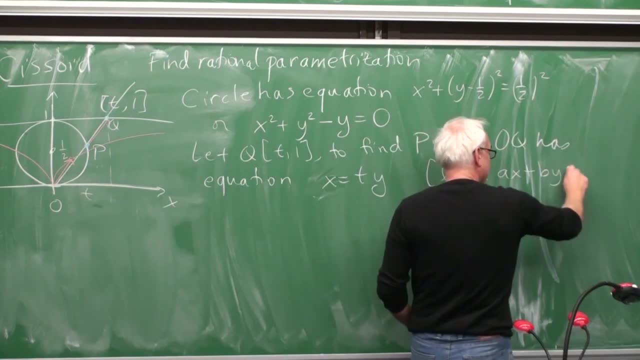 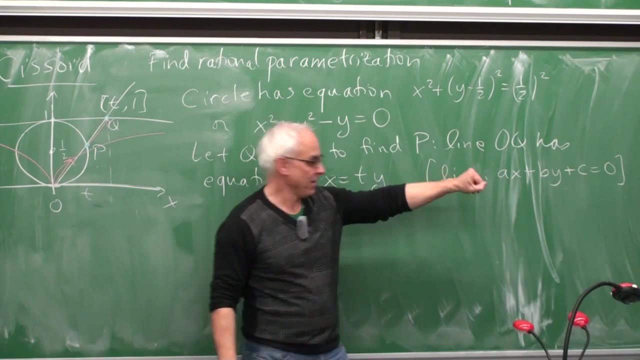 and in fact, generally speaking, the best approach to thinking about a line is to think of it in terms of the form: ax plus by plus c equals zero. That's a symmetrical form for a line, So it's a good idea, generally speaking, if you're working with lines to think about. 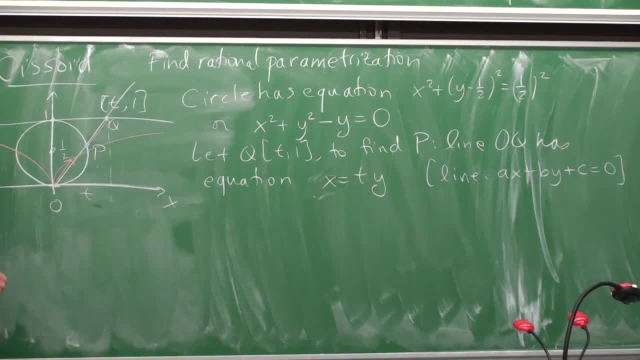 them with that general form, rather than: y equals mx plus b, because this is more general, in particular When b is zero, this will still make sense, but the other one won't. All right, we've got that line then, so it meets. so the line has this equation, and: 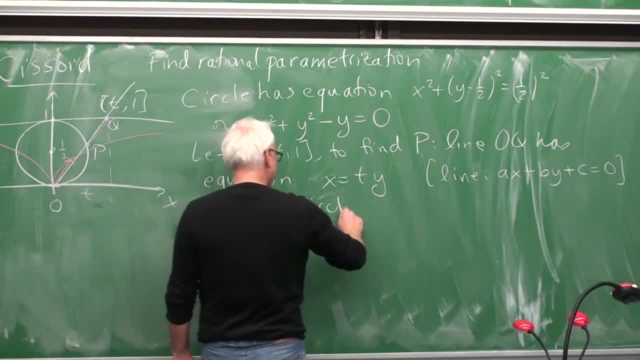 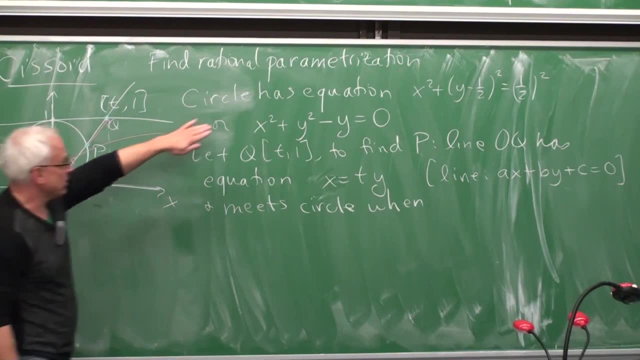 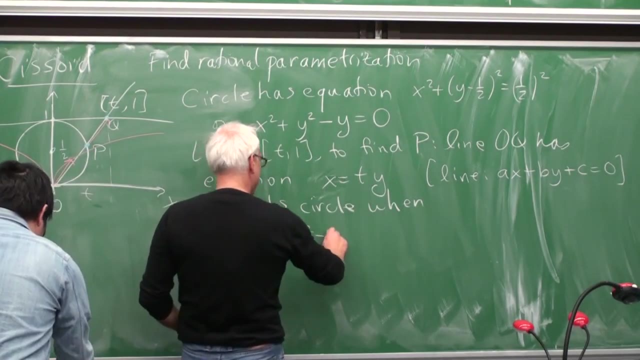 it meets the circle Where, when? okay, what's the equation that we need? We need to plug this into the equation of the circle. Here's the equation of the circle. so we'll replace x with ty. So getting t squared, y squared plus y squared minus y, equals zero. 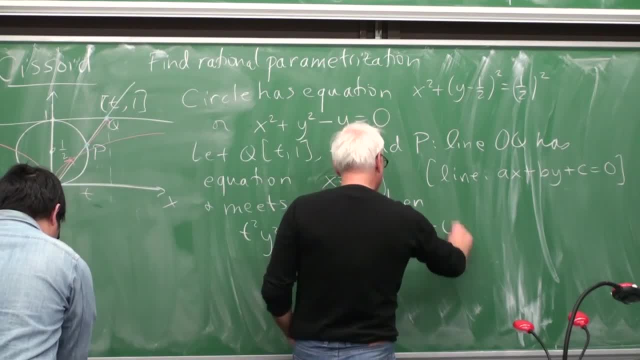 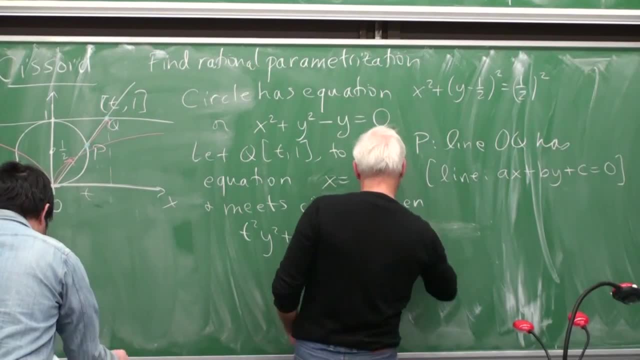 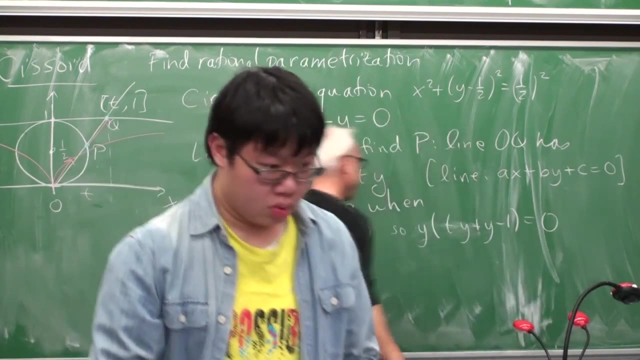 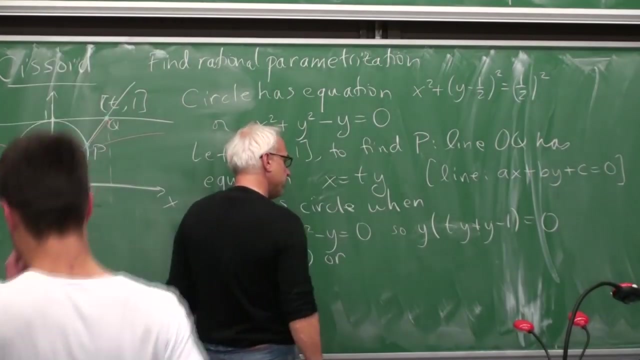 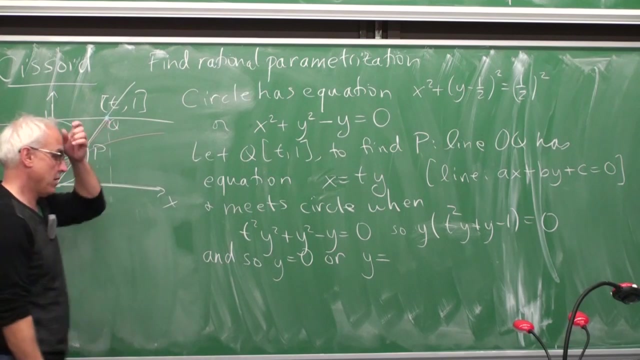 So y equals zero, or well, maybe I'll just factor it, That's the honest thing to do. So y equals zero. So y times ty plus y minus one equals zero, and therefore we get two possibilities. and so y is equal to zero or y equals there's a t squared here, or y equals one over one. 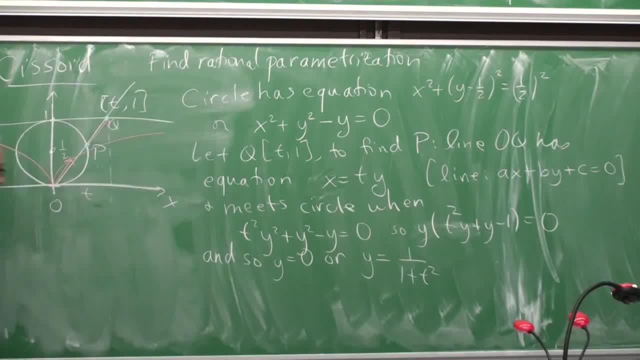 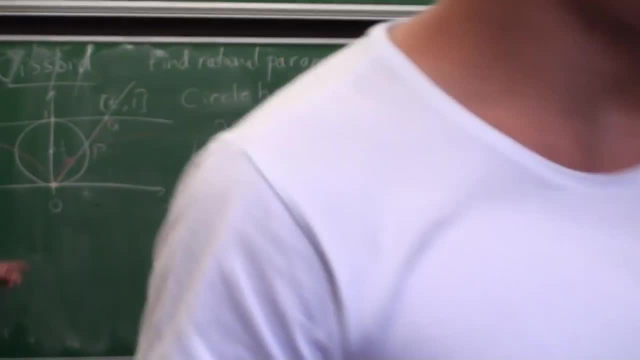 plus t squared. All right. if y equals zero, then we're talking. If we're talking about this point here, we already know about that point. This is the point that we're interested in. so its y-coordinate is one over one plus t. 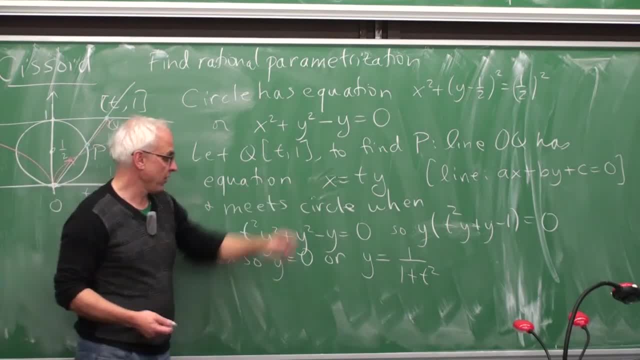 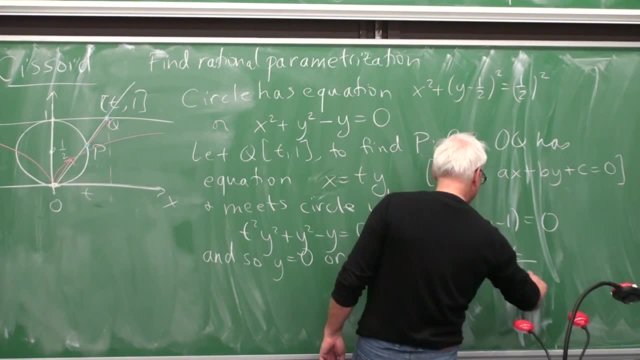 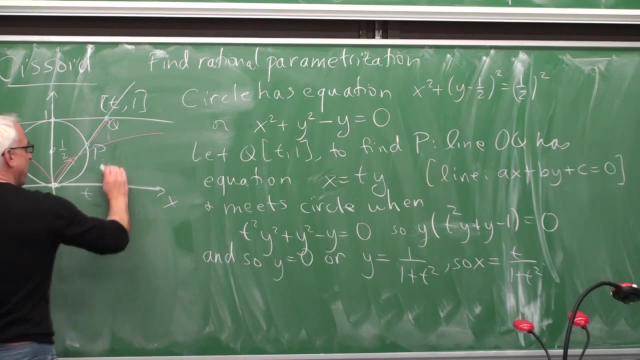 squared. and what is its x-coordinate? Well, it has to be given by this. so x equals t over one plus t squared. So that's the point p. Maybe we'll write it down here. So x-coordinate is t over one plus t squared. 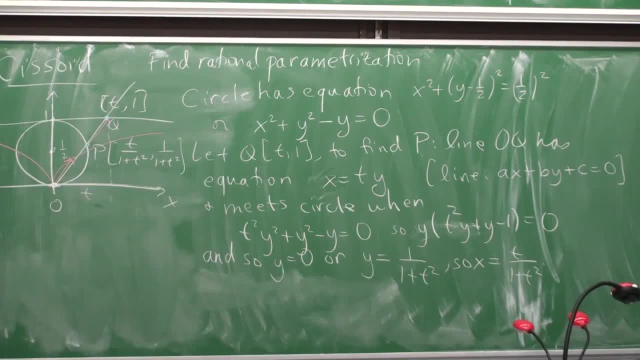 And the y-coordinate is one over one plus t squared. All right, so we have the point p. There's the point p with the coordinates we found. So what do we have to do now to get the sysoid? We have to find this vector pq and translate it to the origin. 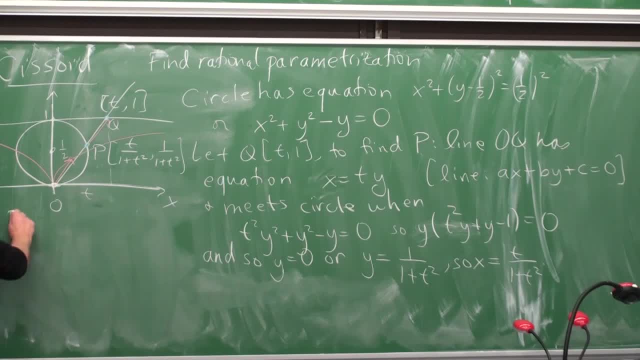 Basically we have to find the vector pq. So let's say, going over here, the vector pq will be the difference between the q-coordinate and the p-coordinate, So t comma one minus t over one plus t squared. And then we have to get this over a common denominator. 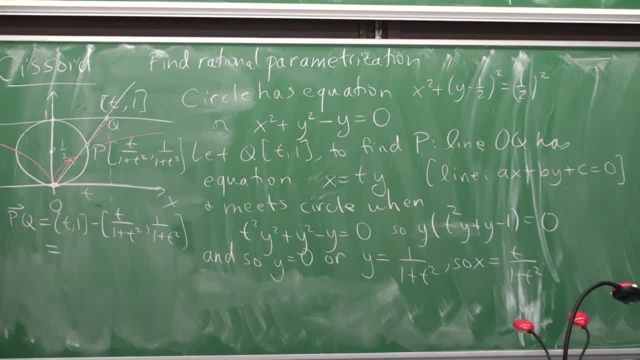 So t minus t over one plus t squared, I guess that will be t cubed over one plus t squared And one minus one over one plus t squared. that's going to be t squared over one plus t squared, And that's in fact then, if we translate it down. well, that will actually be the coordinates. 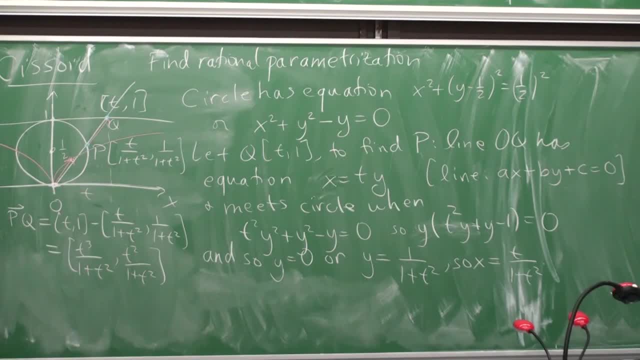 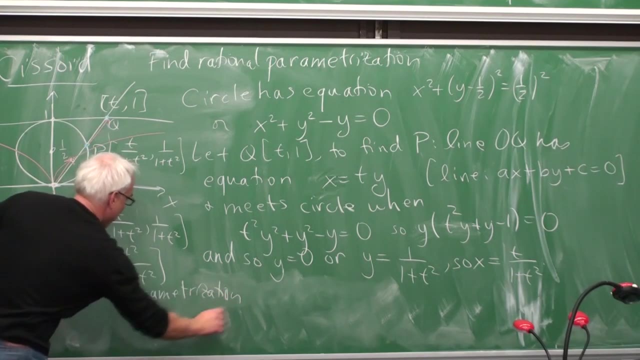 of this point right here. So that is a rational parameterization of the sysoid. This is a rational parameterization of the sysoid x, x is this and y is this. t is a parameter. Alright, there's one more thing that we'd like to do here, which is to find an algebraic. 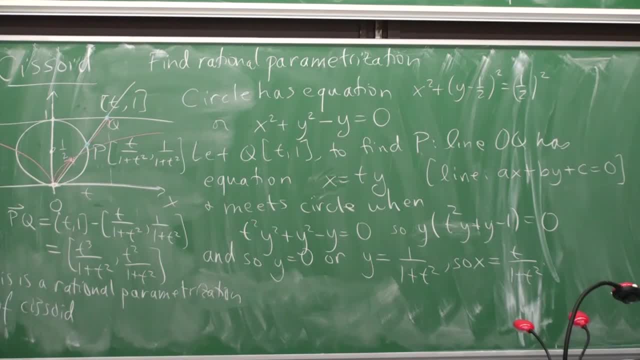 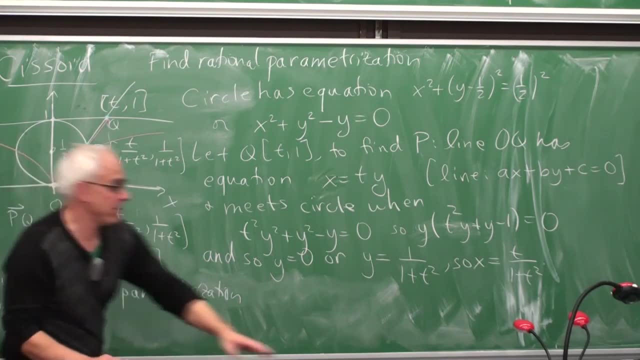 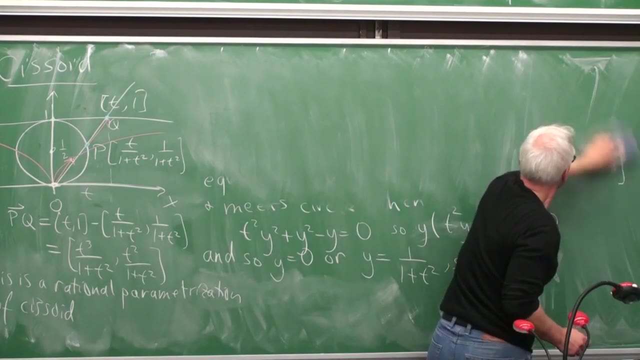 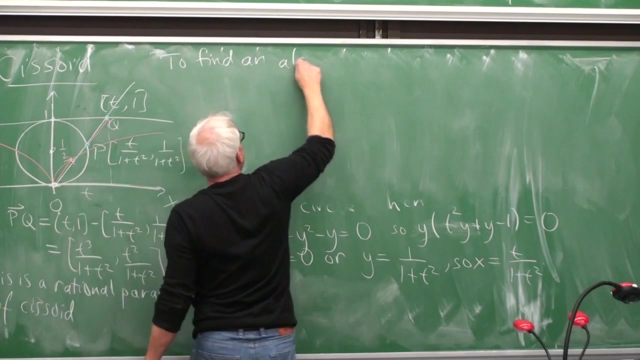 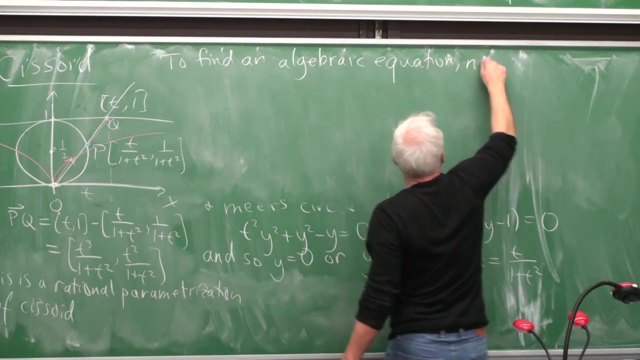 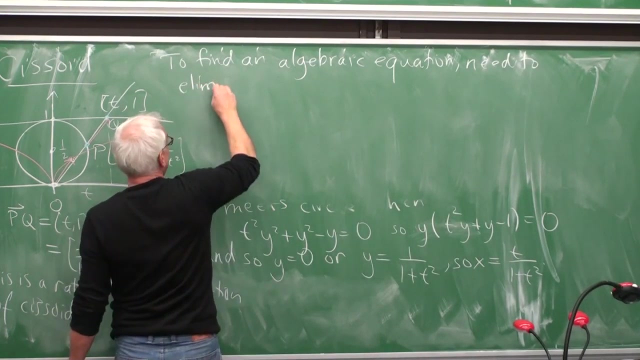 equation for the sysoid. So to get that, we want to essentially eliminate the parameter and just get a relation between x and y. So let's do that here too. So to find an algebraic equation, we need to eliminate the sysoid. 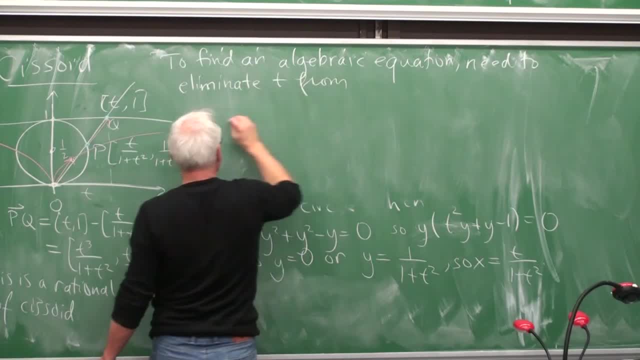 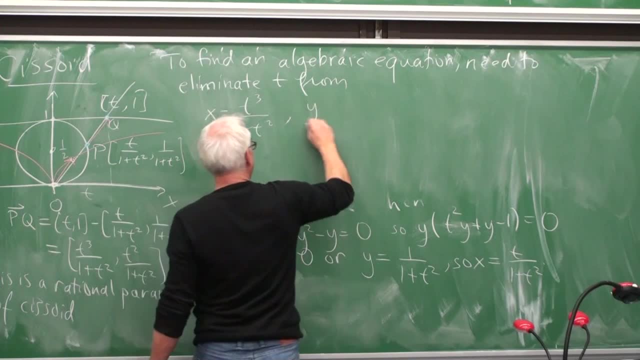 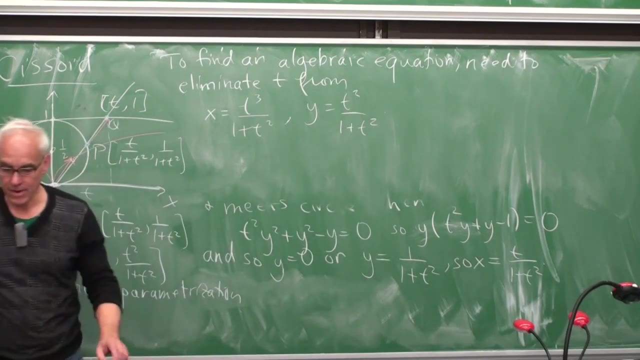 Alright, Eliminate t from the two equations: x equals t cubed over 1 plus t squared, and y equals t squared over 1 plus t squared. Now, this kind of problem is sometimes quite tricky. in this case it's pretty easy because 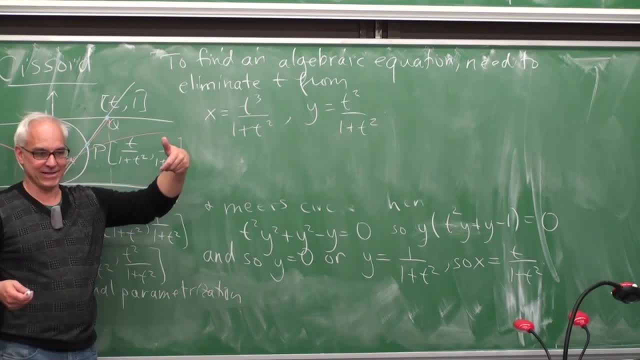 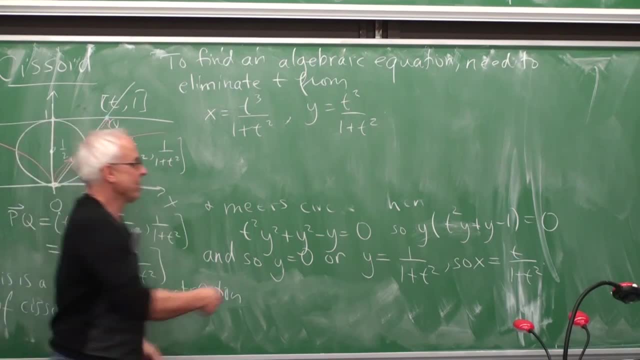 we actually know that the relationship between x and y is. we know that t can be directly expressed in terms of x and y because that's how we set things up. So we recall that the way we set things up was that t was actually just the ratio of 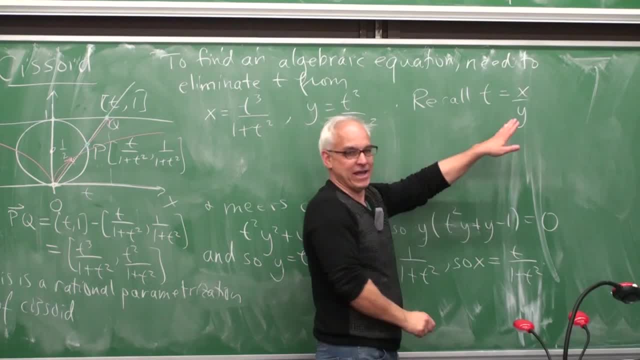 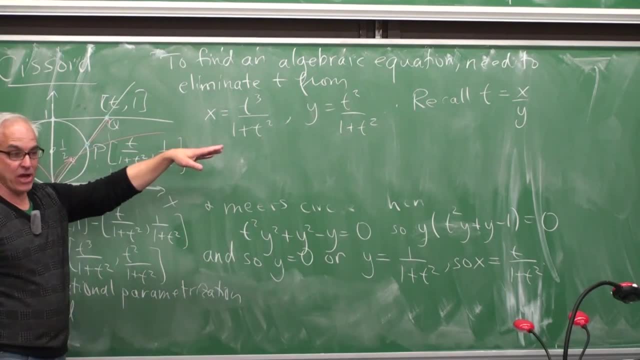 x and y. So that's already t in terms of x and y, which means we can then substitute it into either one of these equations and get an equation that doesn't have any t's anymore. This one's slightly simpler, So sub into t. 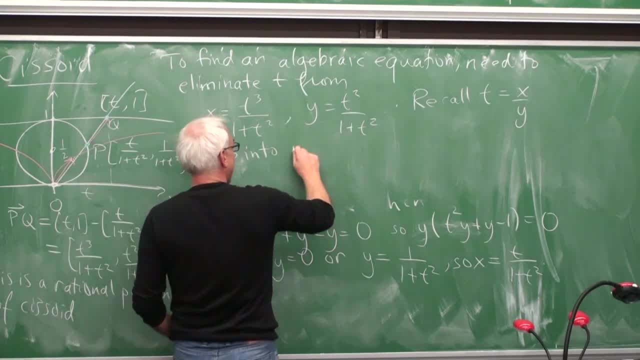 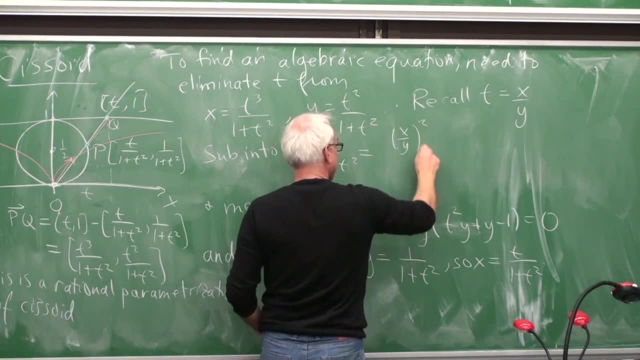 Sub into t, Sub into t And then we get the equation, for y equals t squared, 1 plus t squared. so if I replace t with x over y, I get x squared over y squared, 1 plus x over y squared, for a total of x. 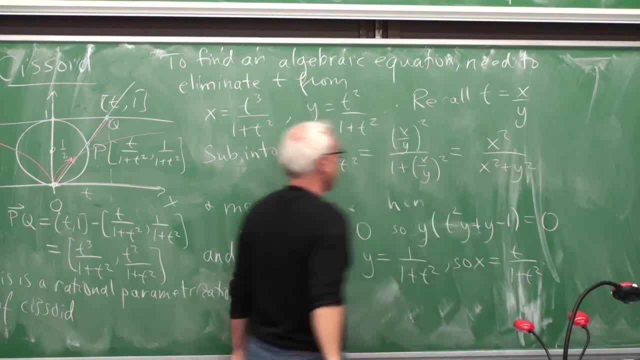 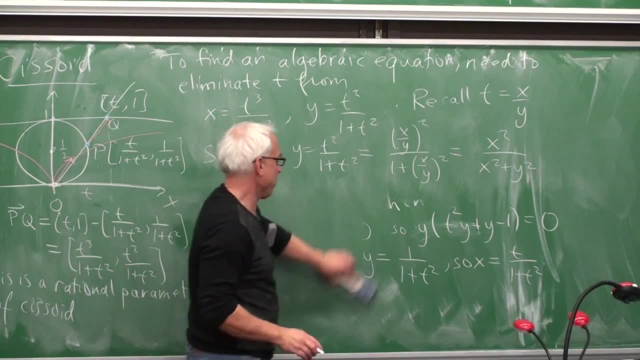 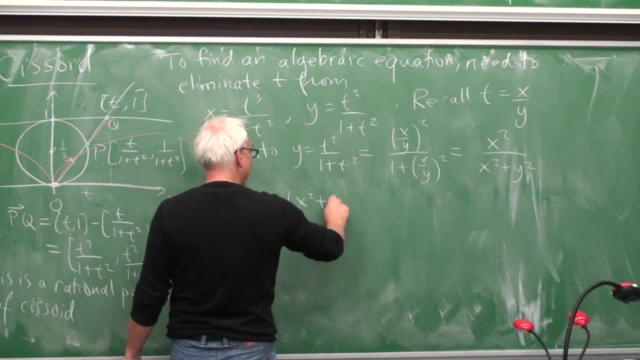 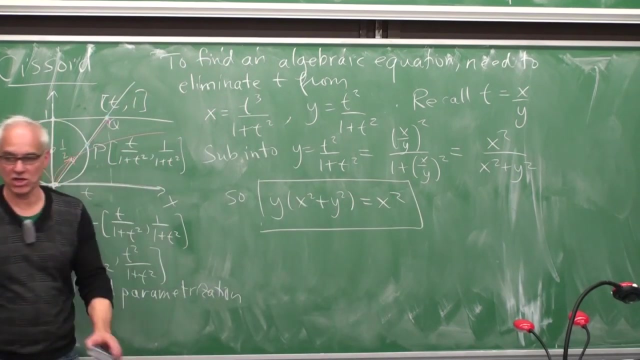 squared over x squared plus y squared, And then that if we equate that to y, we get an algebraic equation for the sysoid. So altogether, y times x squared plus y squared equals x squared. That's now an equation just relating x and y. 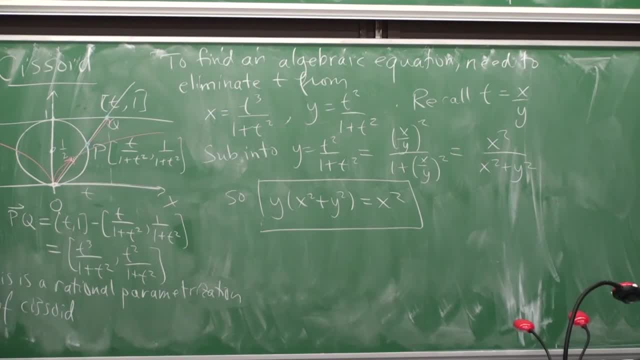 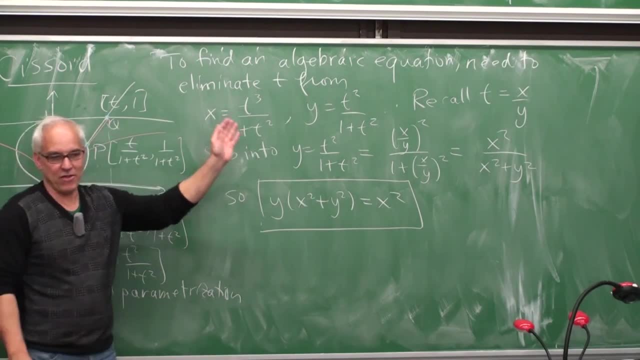 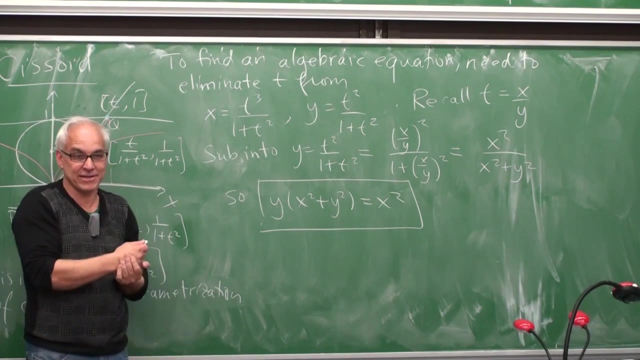 We've eliminated t. Okay, notice the way I've written things out. I've been rather verbose, but maybe not too verbose. I've tried to tell a story. I've tried to write more or less English sentences, Maybe not completely, but I'm sort of aiming to do that. 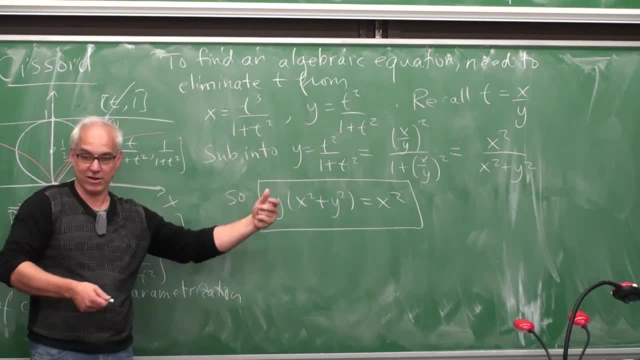 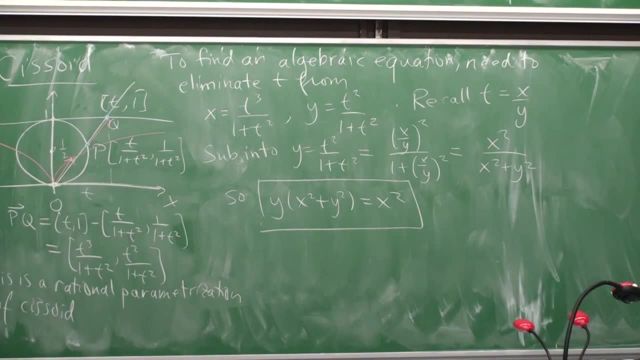 And if I was actually doing this on an assignment for lots of marks, I would make sure that I would try to write English sentences, So I might even have a period, for example, at the end of statements like this, making it look like a work of literature as well as a work of mathematics. 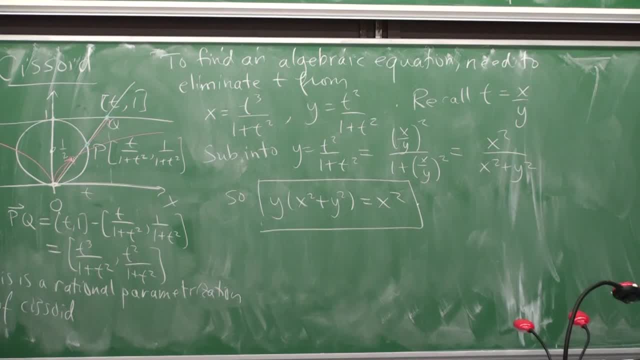 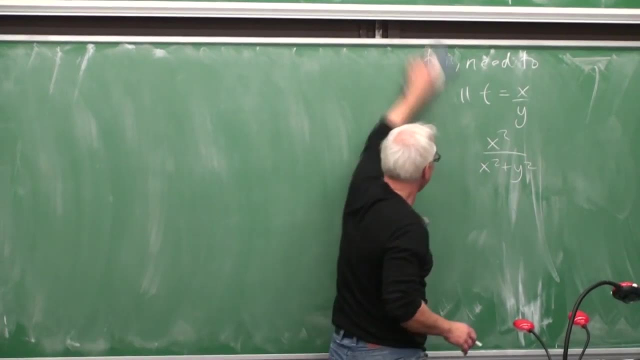 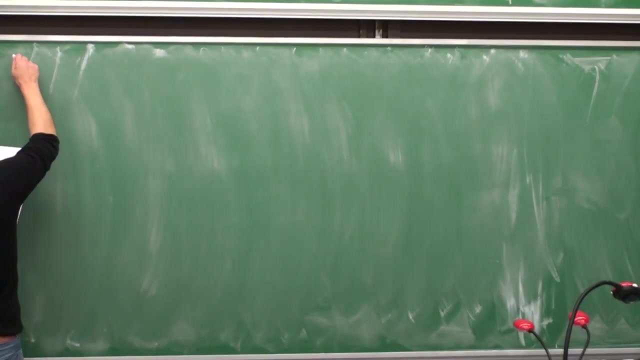 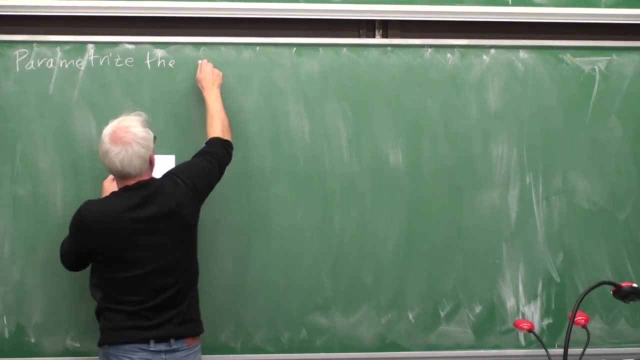 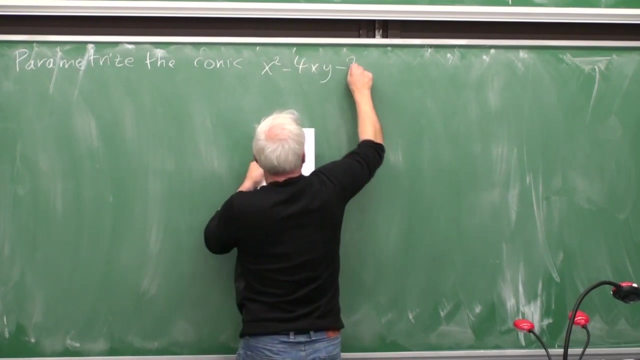 All right, good, So that's the first. That's the first question. The next one I want to look at is a parameterization question. So the next question I want to look at is the question: can parameterize the iconic x squared minus 4xy minus 2y squared equals 3.. 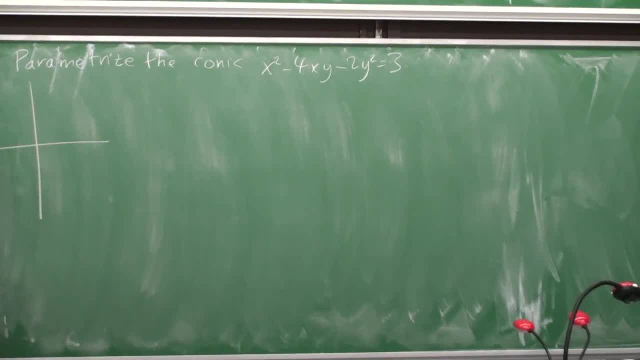 It's not necessary, but if you have a computer algebra program around, it's probably not a bad idea to quickly graph this thing and see what it looks like, just out of curiosity. And it's a hyperbola that does something like this roughly. 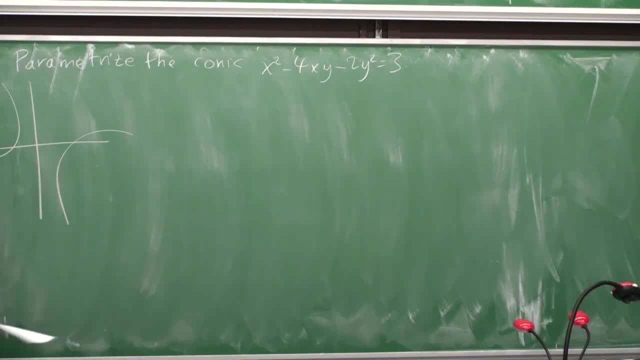 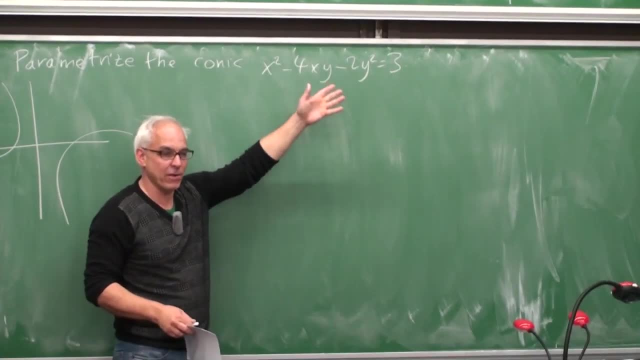 Okay, And we need. We need a point on the hyperbola to start with. So we have to actually just hunt around for some small values of x and y that will satisfy this And fortunately, in this case it's not that hard to do that. 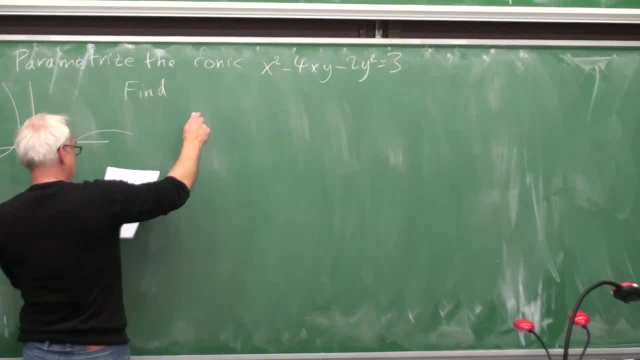 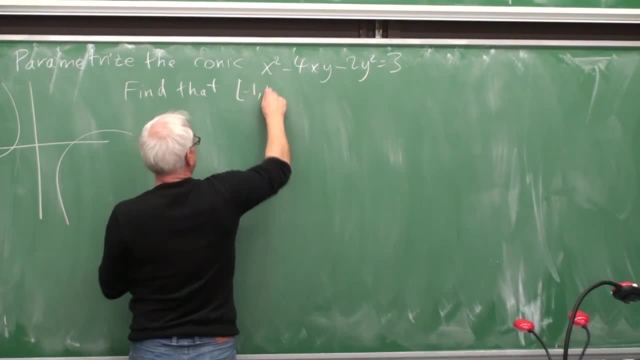 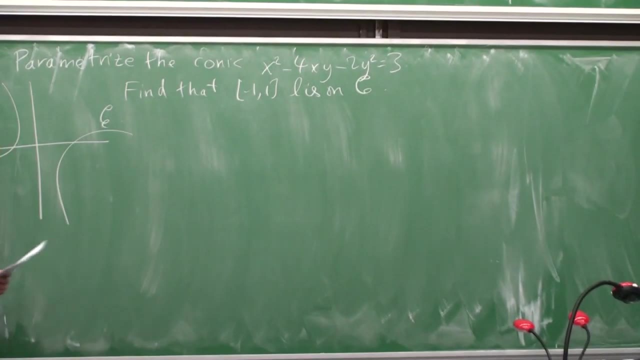 So we find by trial and error that the point minus 1, 1 lies on c. Let's call the thing c, All right. So we're going to use that as our base point for a parameterization And most of you got this fine. 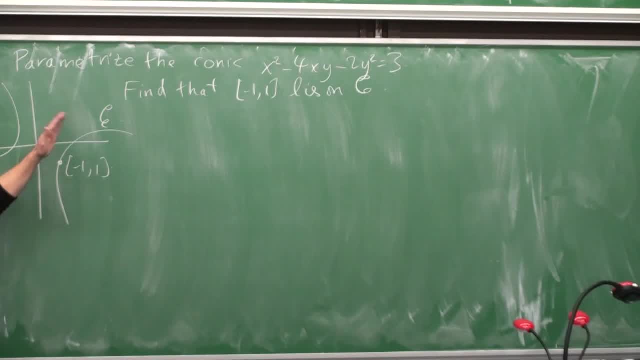 There are many possible answers, because there's lots of ways of choosing an auxiliary line to set up your parameters. So I'm going to do something just a little bit different, which a few people did So, just to give you an alternate view which is sort of in keeping with our approach. 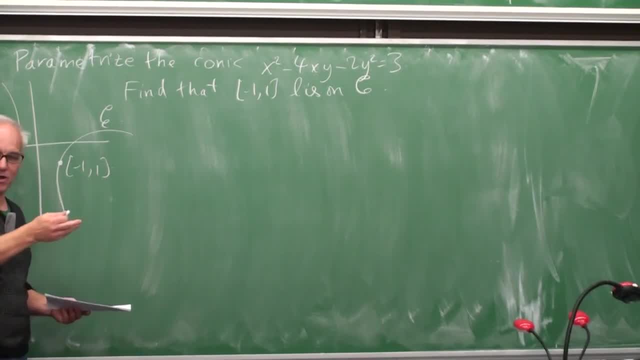 to things, that if you have a problem involving a point and a conic or a curve, if you translate the point to the origin, maybe things are simpler in general. Okay, So let's do that. So let's translate c so that the point 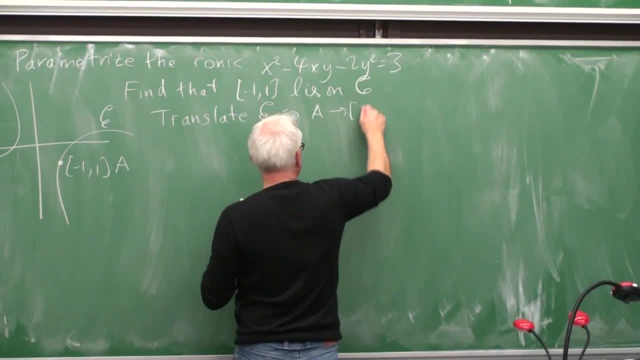 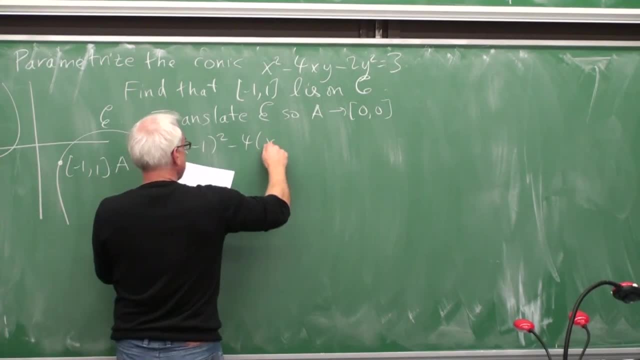 let's call it a. here goes to the origin. Okay, So we get a new equation: x minus 1 squared minus 4x minus 1y plus 1.. Minus 2y plus 1 squared equals 3.. 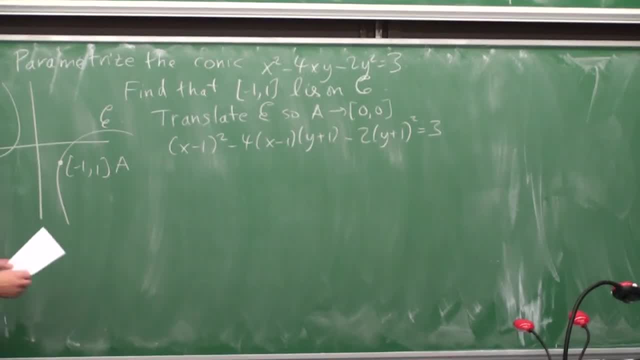 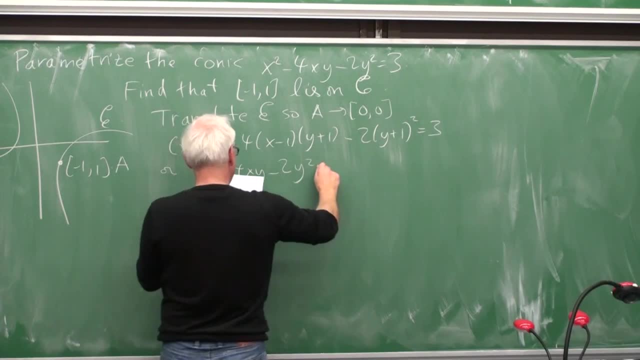 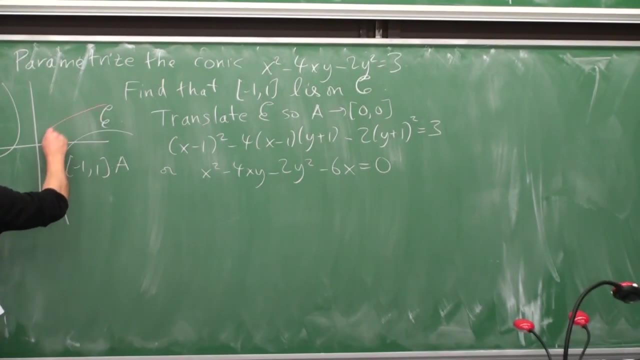 And admittedly you have to do a little bit of algebra here. So we simplify this to get x squared minus 4xy minus 2y squared minus 6x equals 0.. So we've really actually translated the conic. I might just sort of try to draw it like this: 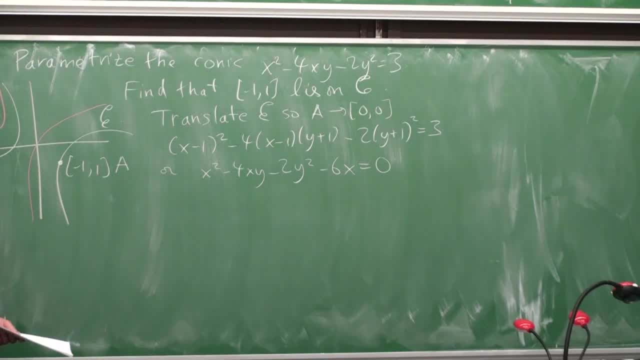 Yes, Shouldn't the other way around? should be x Plus 1, 1, minus 1?. Well, if you think about, if you think what happens if you replace in this, if you replace x with and y with 0, 0,. 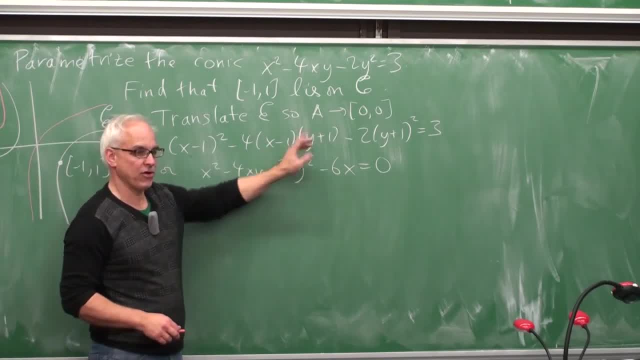 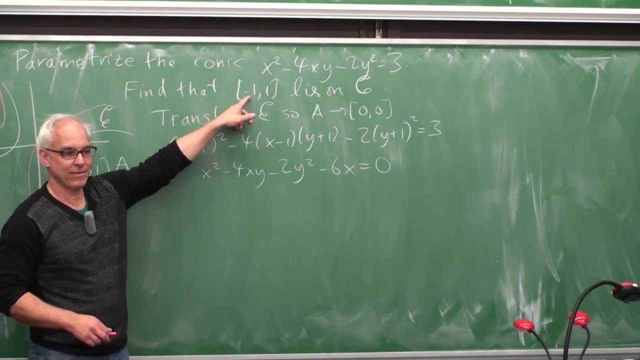 you're going to get minus 1 squared minus 4, this point, this point, You're going to get the original points. There's a minus sign here because this is a minus sign Generally, it's x plus the x coordinate. 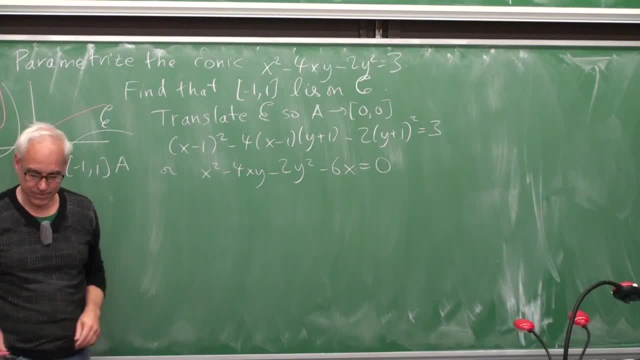 y plus the y coordinate to translate it down. Okay, So now that the thing is at the origin, our point it's the point 0, 0, so the parameterization of the line can be relatively simple. Now we set: 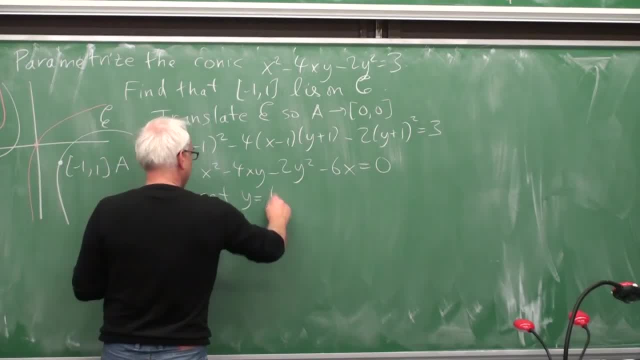 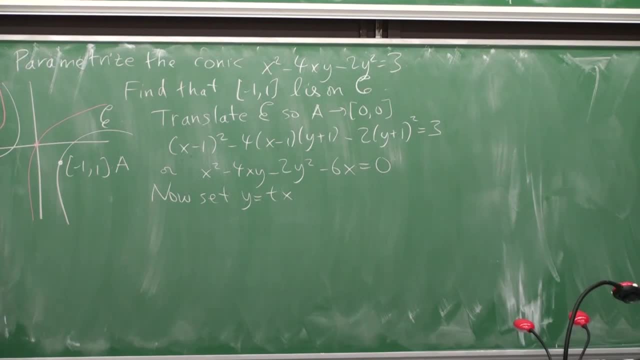 y equals t times x. In terms of a parameterization, I guess what we can think about that being well. well, that's kind of a slope. There's the line y equals t, x is: this is 1, and that's t. 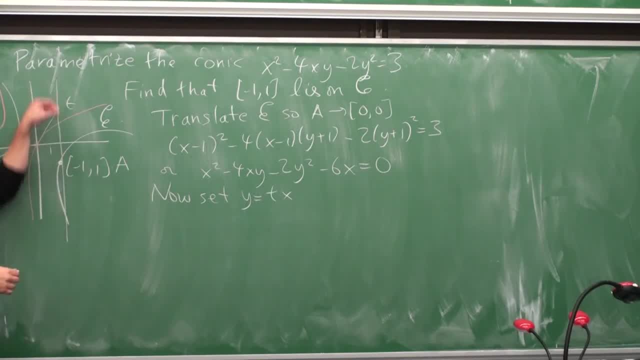 So what we're really doing is we're using this line x equals 1 and the natural parameter on it to make lines. All right, We set y equals t, x and we sub in, So we get x squared minus 4,. 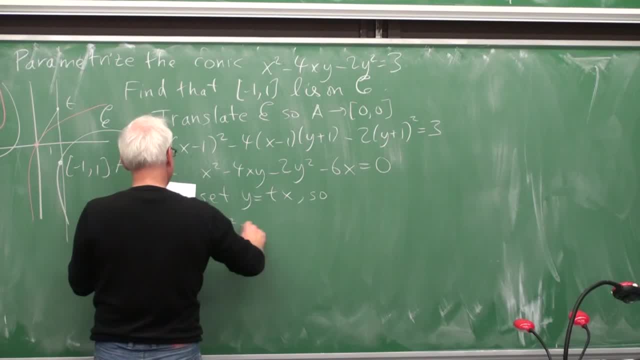 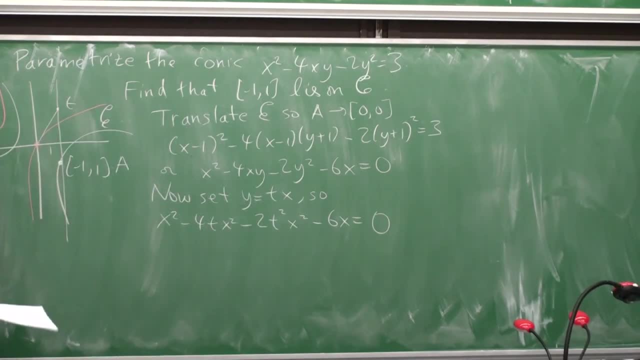 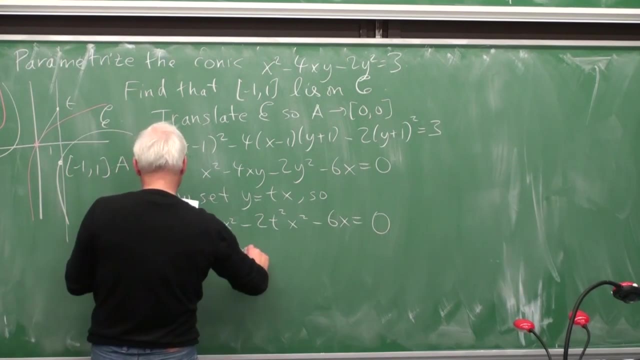 plug in. y equals t x, so t x squared minus 2, t squared x squared minus 6x equals 0.. There is a a common factor of x, which we'll pull out, and x minus 4t, x minus 2t squared x minus 6 equals 0.. 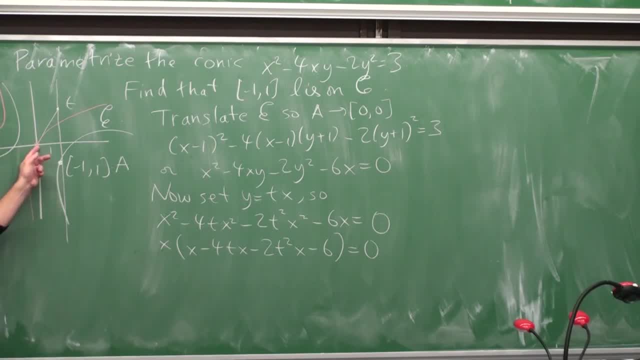 And this x equals 0 corresponds to the point that we already know, which is on this conic. There's already one point on the conic that we know. There's one solution already that we know, So there's no need to use a quadratic equation. 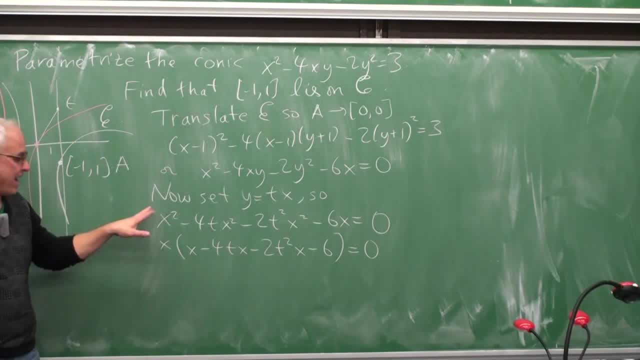 There's no need to use a quadratic equation. Okay, Quite a few people had some equation, but it's going to be quadratic. and then they said: well, we're going to use the quadratic equation. You don't want to do that? 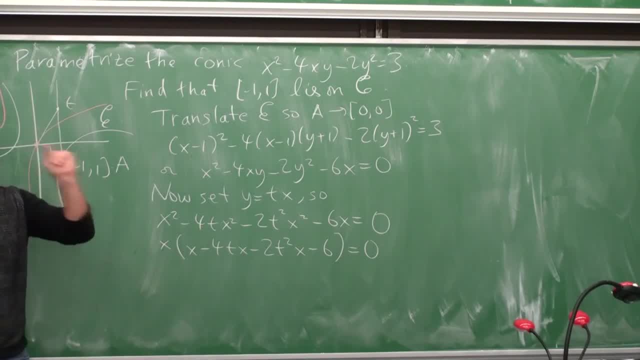 You want to observe that there are two solutions and you know one of them already. So, in particular, if you have a quadratic equation and you know one solution, then you know what the sum of the two roots are, because of the coefficient of x. 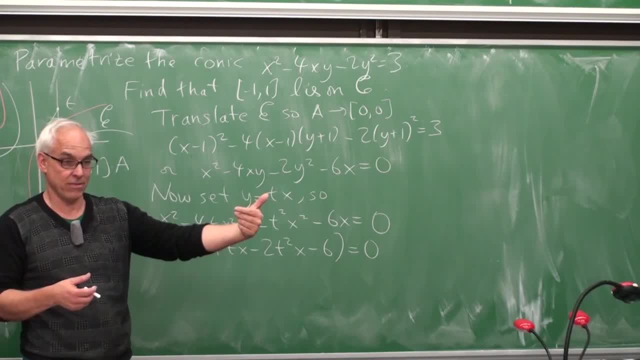 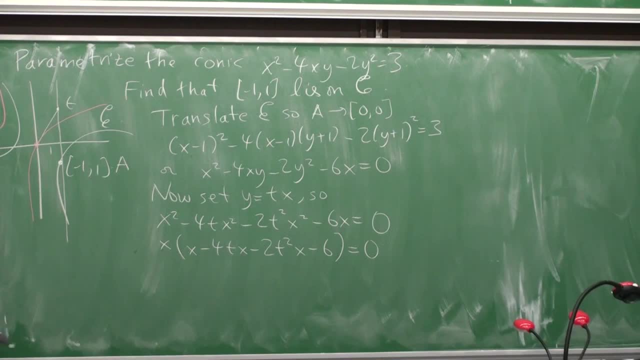 or you know what the product of the two roots are because of the constant term, All right. so you don't have to use the quadratic equation, You don't have to invoke the square root, All right. so now we've got the condition x equals 0,. 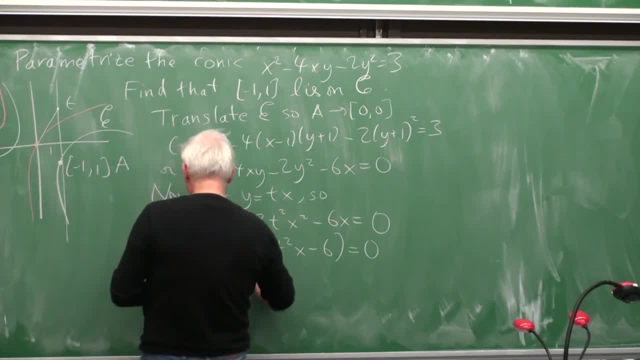 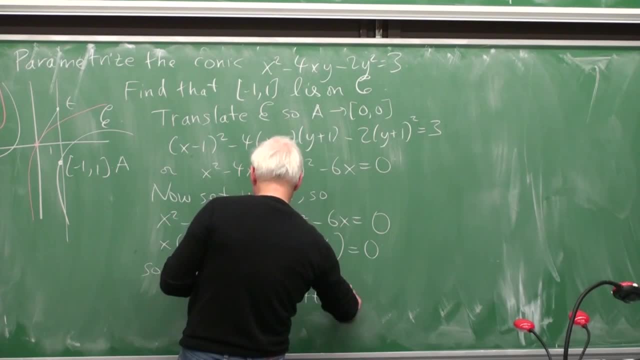 or we can solve for x here, or x equals 6 over 1 minus 4t, minus 2t squared, in which case y is then given by t times x. so that's relatively simple. So 1 minus 4t. 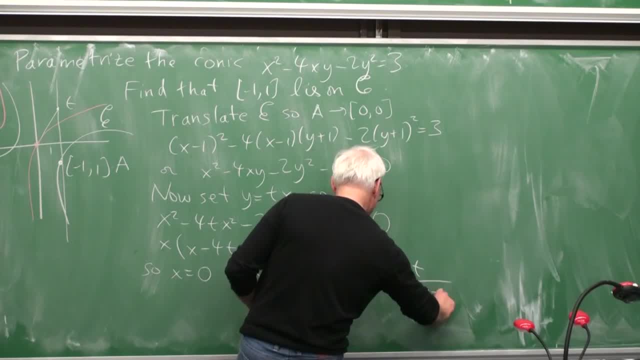 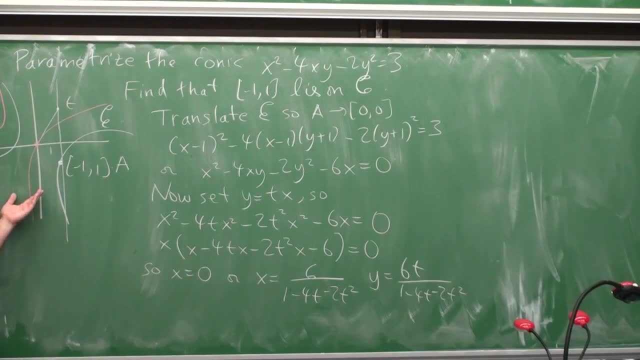 and y equals 6t over 1 minus 4t minus 2t squared. That, then, is a parameterization of this translated red conic, And to get a parameterization of the original one, well, we have to translate that back. 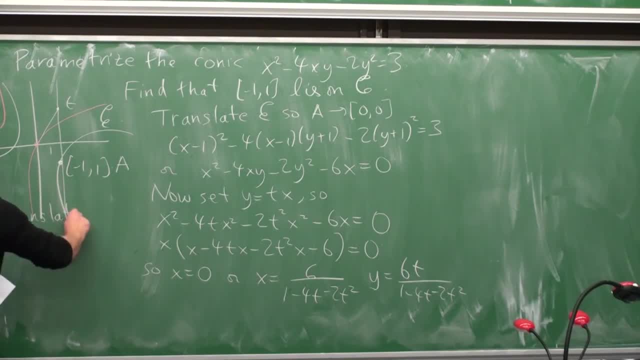 So translate back to get to get a parameterization of c, And that will be x and y is equal to well. in this case, what we do is we just we can just write 6 over 1 minus 4t, minus 2t, squared minus 1.. 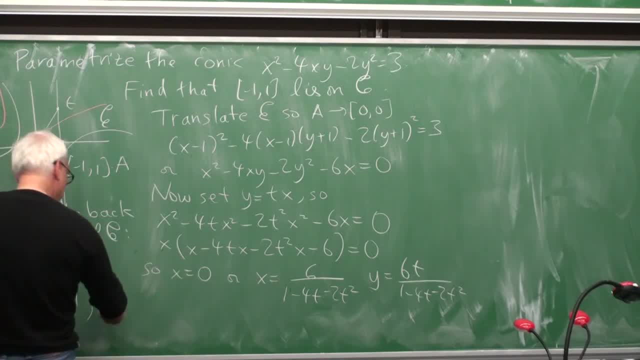 And the other one is the y coordinate. and the other one is the y coordinate and the other one is the y coordinate: 6t over 1 minus 4t minus 2t squared plus 1.. Question: I'll just like the domain of t in that parameterization. 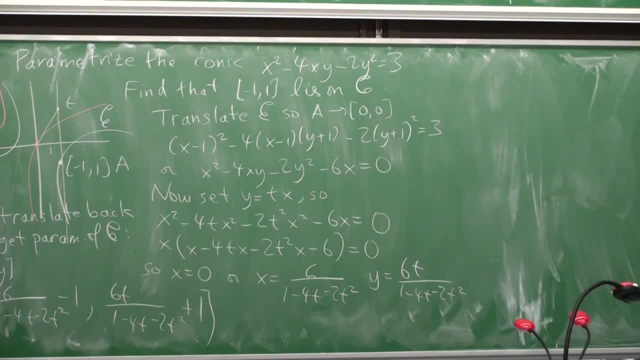 All right, so this is a good question. What's the domain of t here? And this is a little bit, seemingly a little bit tricky, because it looks like there's two branches to this hyperbola that maybe you need to think about. 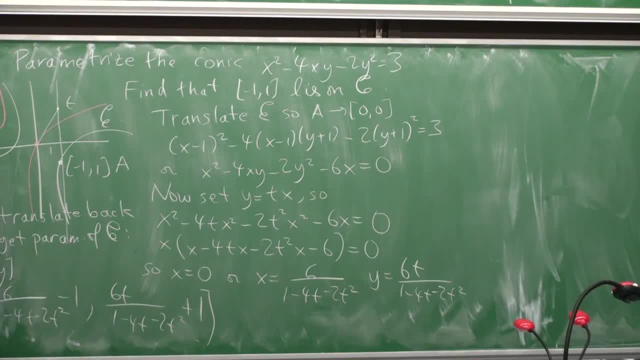 Both branches separately. In fact, that's not the case. The algebra takes care of the whole story. There's a slight complication, though, in that you really, to fully understand this parameterization, you really need a projective view. So it's a full parameterization. 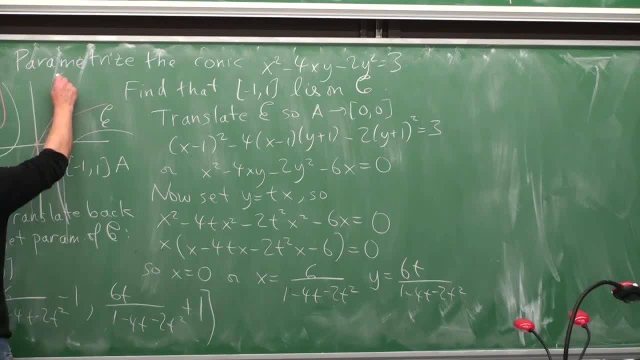 only when you go to the projective view, which allows a point at infinity in this direction. So in the projective view, this line has a point at infinity, as we've learned, And you should really think of that point at infinity as being an extra point. 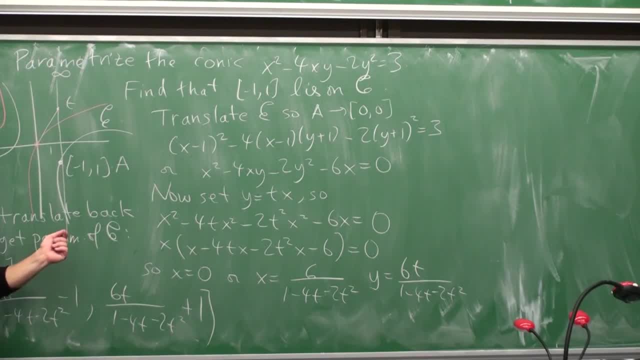 which you need to complete the parameterization. Why do you need that extra point at infinity? Well, because there will be a certain direction to these lines that we're drawing. We're drawing lines through here, or let's say, through here, So most of the lines that we draw through this point. 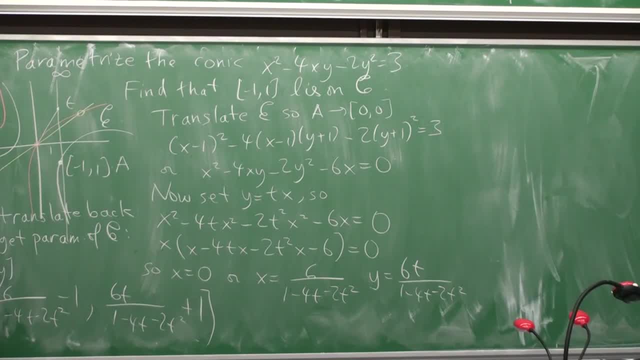 will actually meet the conic at some point. Okay. Okay, There's some other point, but there's this sort of: there's this one here which will meet it at this point here, Yeah. And then there's also the line: 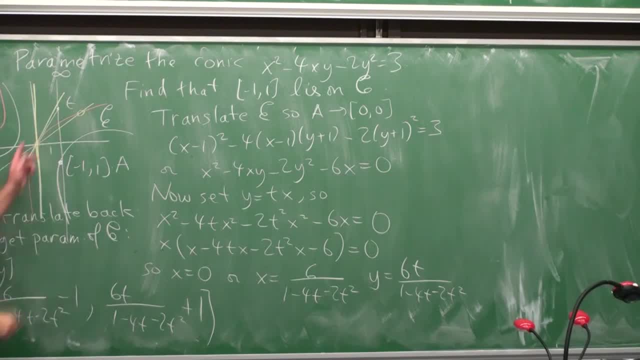 that's parallel to the line that we're using, which will also probably meet the conic somewhere. So this line that's vertical, which is in the same direction really as the parameter line that we're using, should be thought of as meeting this line at infinity. 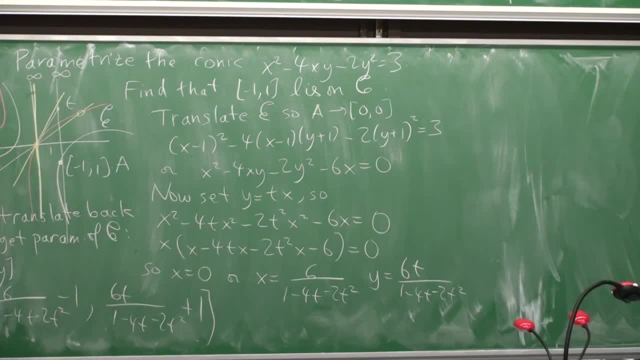 So you're getting the corresponding point on the hyperbola when you set t equal to infinity. What does that mean? Well, it doesn't mean that we need, it's just a projective view. It just means that when t gets large, 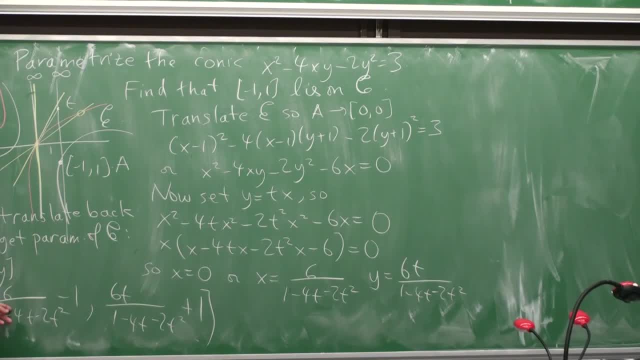 the denominator here will become large and this whole thing goes to zero. And when t is large here, we get zero here. So in that case we're just picking up the original point that we're talking about. So the answer is: it's a good question. 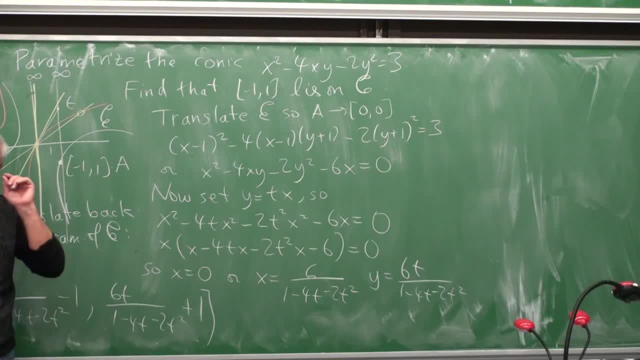 The full parameterization is obtained by thinking about the projective view, where you have to add a point at infinity to the line. Yeah, Don't? you have to make sure that t is not a root of that quadratic equation in the denominator? Not really, because okay. 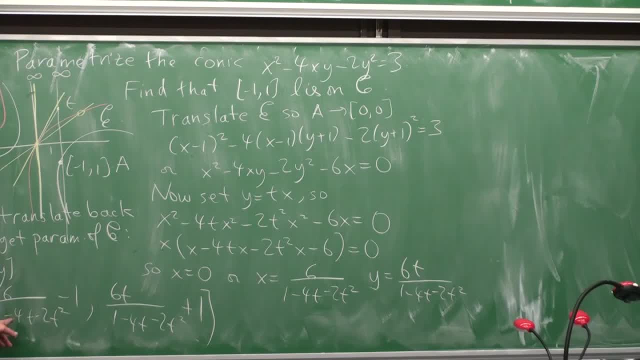 so that's another good question. Okay, what happens if t is? what happens if t is a zero of this, of this, or denominator here? In that case, you would say, well, this blows up. Okay, what does that mean? 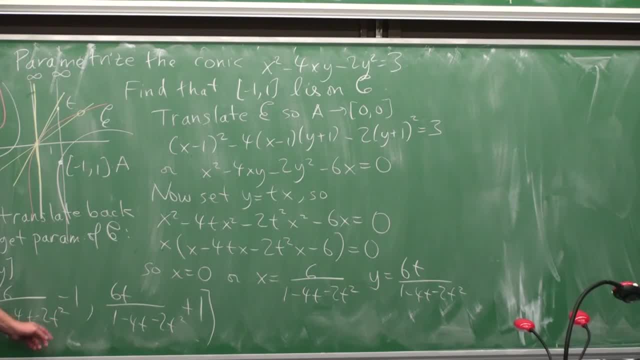 Well what that means. and there will typically be two such values of t. So there will be two directions where it seems, as if we're not, that something strange is happening. To understand that again, you need to go to the projective point of view. 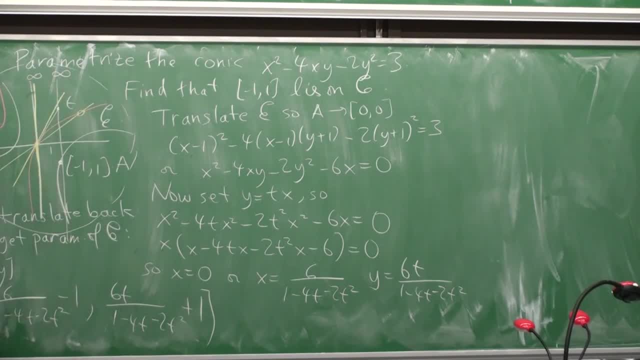 You need to realize that this conic that we're talking about is a hyperbola and it has two points at infinity. Okay, this is a hyperbola, So it has asymptotes. So it has two asymptotes like this: 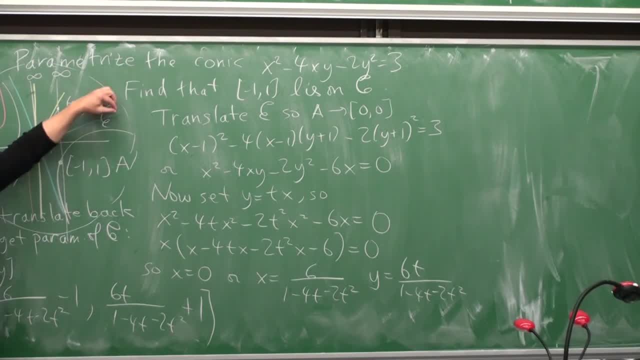 And as the conic gets further and further away, it gets closer and closer to these asymptotes, And where those asymptotes meet the line at infinity, that will be a point that actually the conic goes through, And there will be two such points. 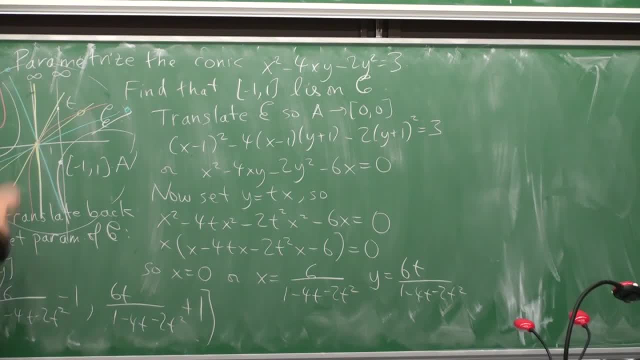 one for each asymptote. So, in other words, the full conic is not just the conic you see in the plane, It also has these two points at infinity. and those are exactly the points that you're picking up when you're looking at the zeros here. 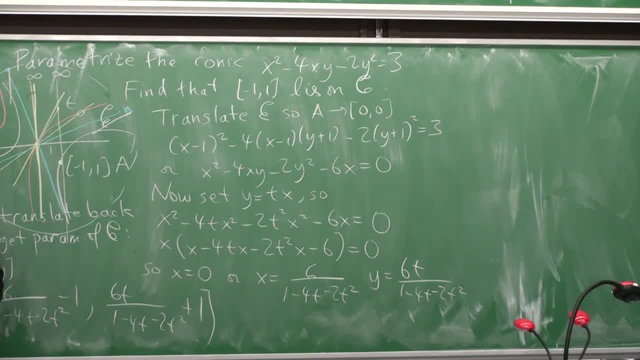 When you get the zero down here, then you're essentially picking up those points at infinity. And if we use projective coordinates instead of affine coordinates, that would all be completely clear. You know, instead of using capital X and capital Y, if we use little x, little y, little z. 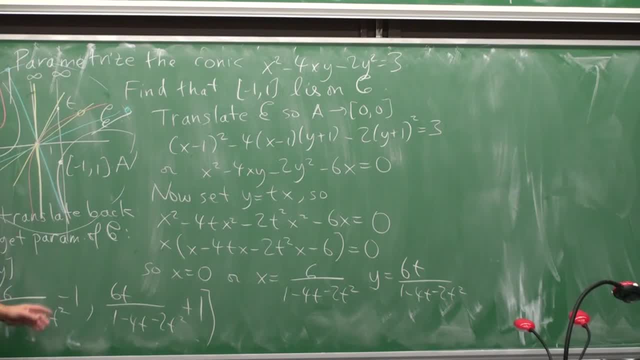 the three coordinates, three homogeneous coordinates, then that would be completely clear. We would see that that those points at infinity being parametrized this way, All right. so let's now go to one of the more challenging questions that I've given you so far. 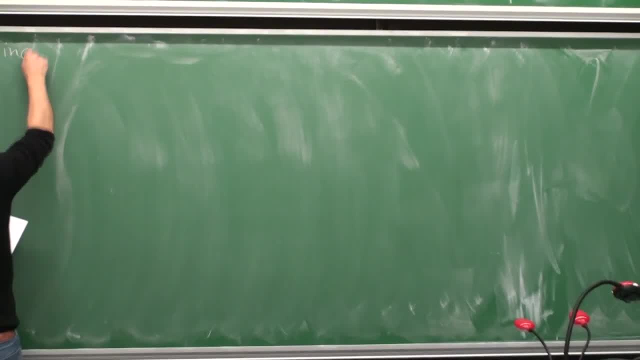 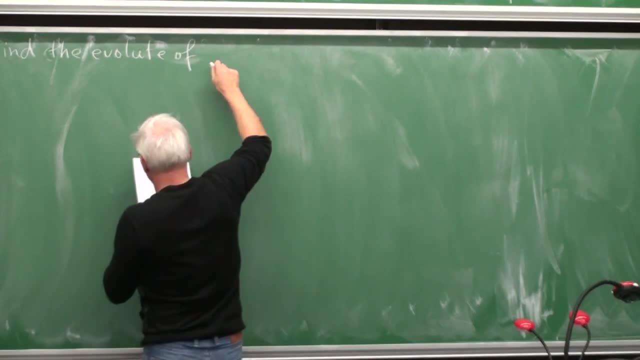 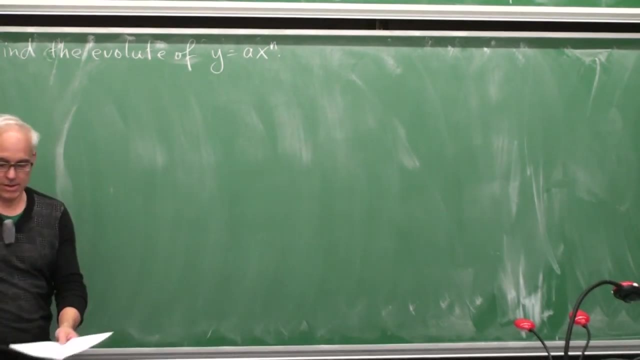 which is find the evolute of the power function. y equals a times x to the n. All right, so we'll do a quick diagram Function, typically something like this, And of course a parametrization is easy enough to cook up. 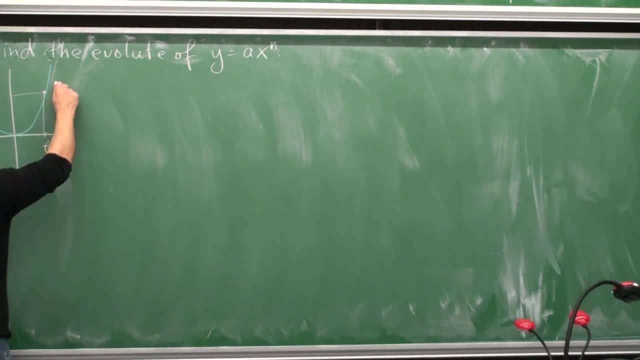 We can say, let that be t, and then that will be the point: t, a, t to the n. So what we'd like to do is we'd like to find, in terms of t, where, where the associated center of curvature is. 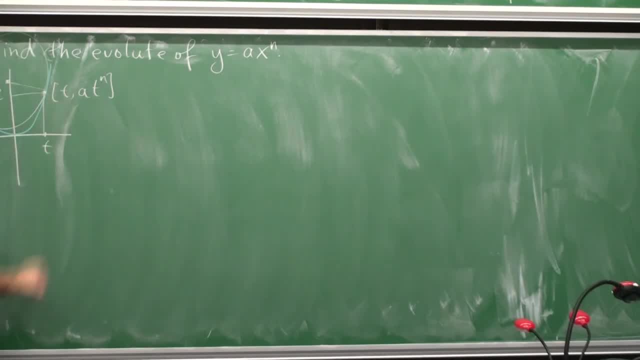 That's the center of the osculating circle that best approximates the curve at that point- Or it's another way of thinking about it- it's the place where adjacent normals meet. From the 17th century point of view, adjacent normals meaning just two normals. 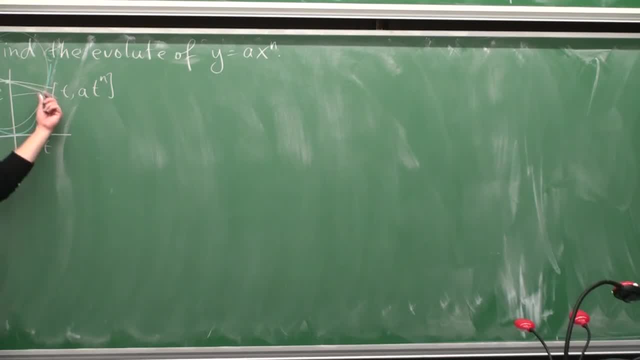 which are very close to each other. They're sort of limiting position as the two points get together. All right, so our strategy is going to be to compute these normals, compute the intersection of two nearby normals and see what the limiting value for this point is. 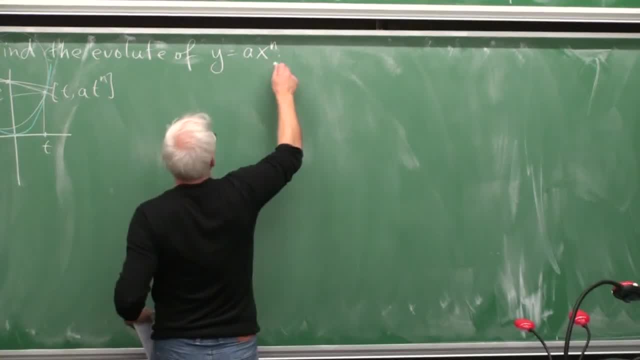 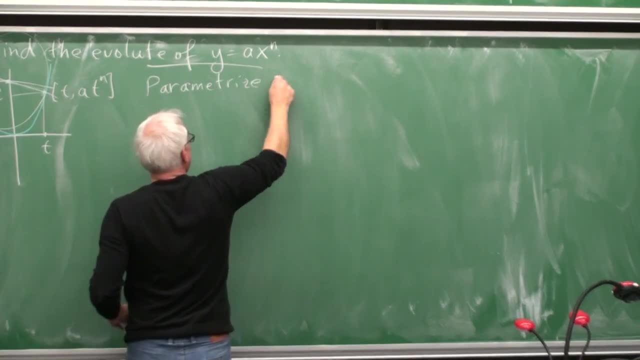 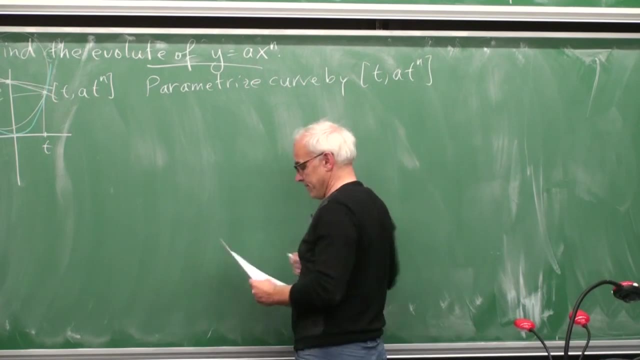 All right. so the first thing that we do is- well, we've said that already, but let's write it down- So parametrize the curve by t, a t to the n. So at this point, what we'd like to do is write down. 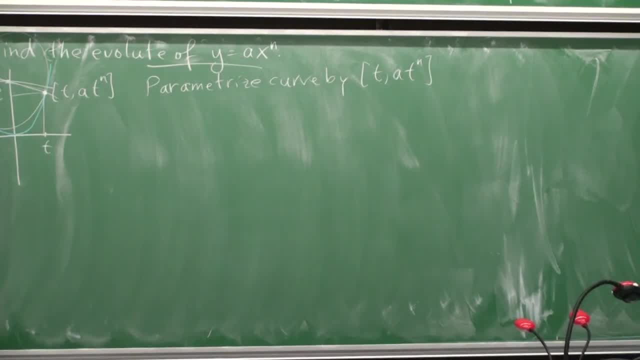 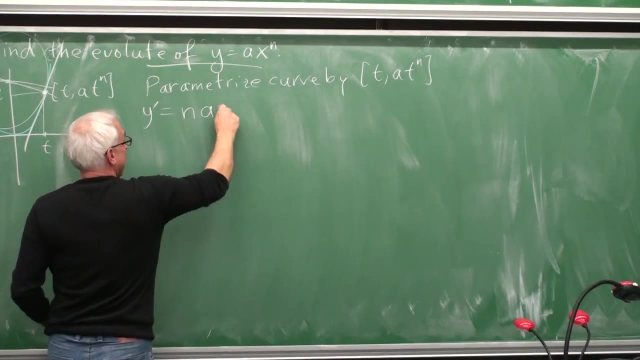 the equation. for the normal, The simplest thing to find out is the derivative, because we know how to differentiate it very quickly And the derivative is giving us the slope of the tangent. Okay, so if we differentiate y, prime equals n a, x. 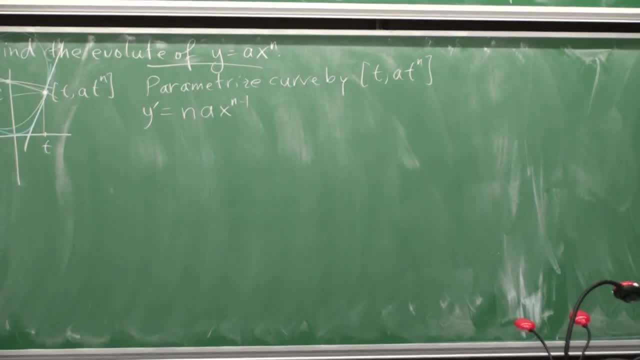 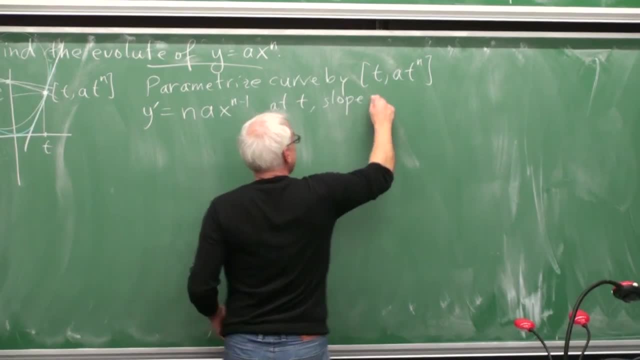 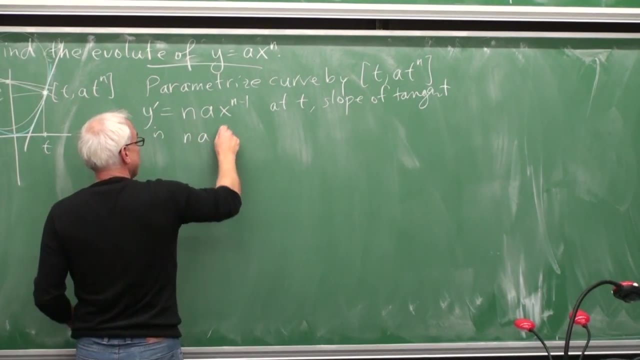 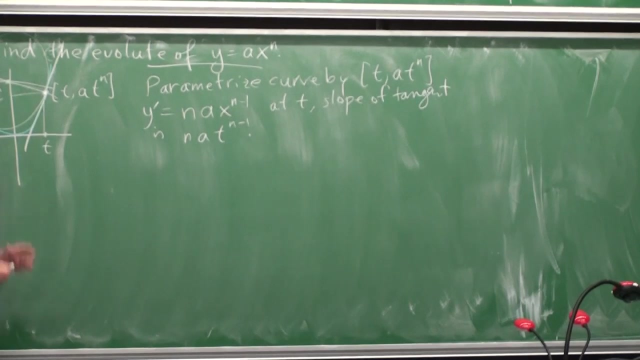 to the n minus 1, that's the derivative, And so at t, at t, the slope of the tangent is n a t to the n minus 1.. That's the slope, And so a direction vector for the tangent. 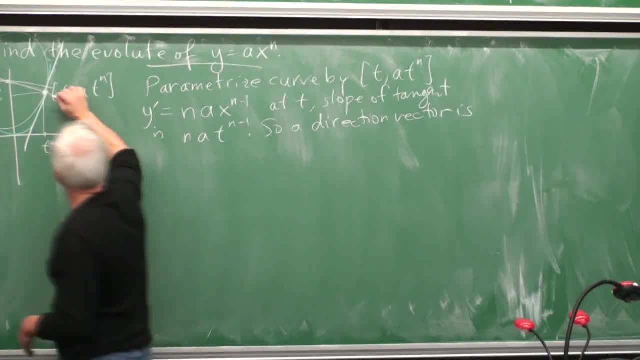 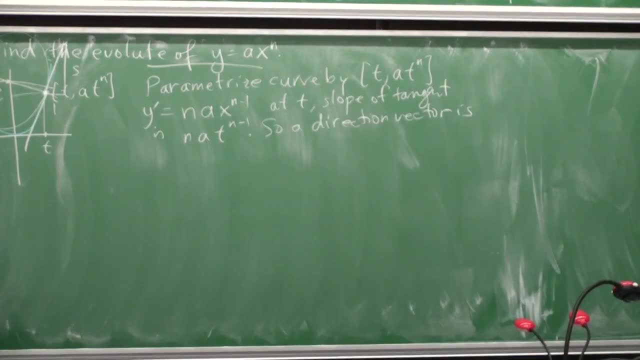 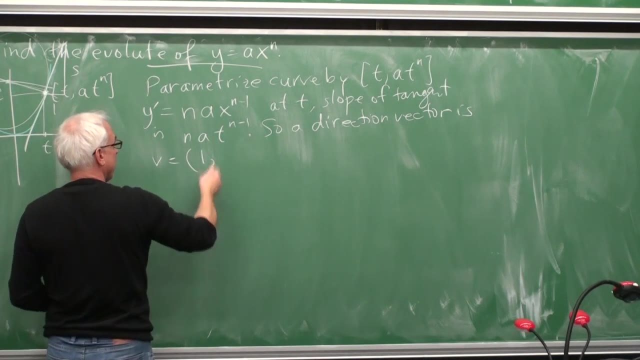 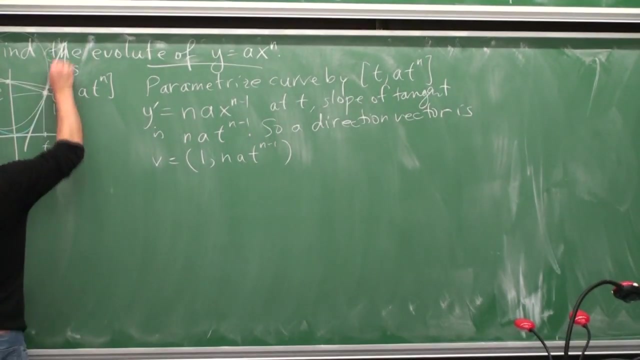 so a direction vector is- think of that- 1.. And the slope, And a direction vector is 1, s Say v equals 1, the slope n a t to the n minus 1.. That's that vector. there that I'm drawing v. 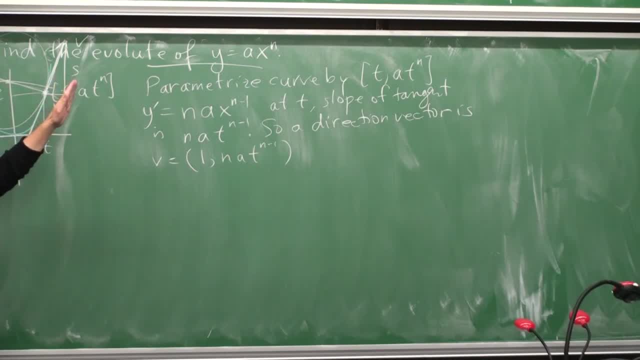 So that's a vector in the direction of the tangent, which is, of course, perpendicular to the normal, And that's the best thing that you want in order to write down the equation of the normal, because you want to write down a line in terms of its normal. 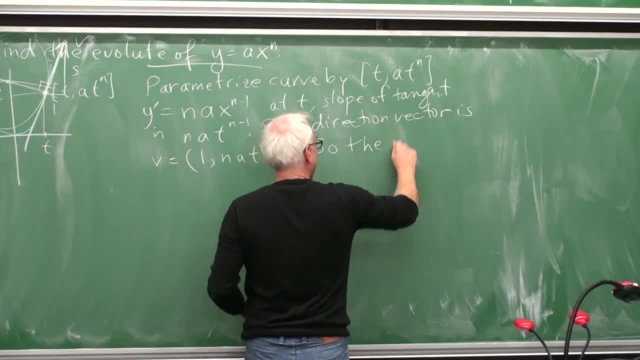 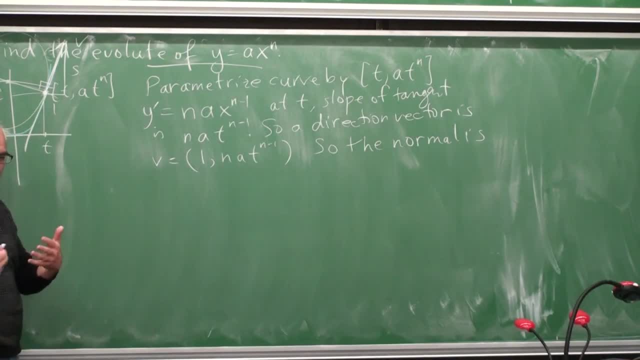 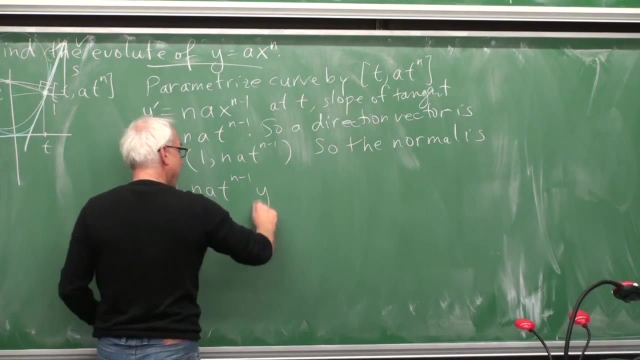 So the normal has equation, or the normal is: well, we're just going to take this vector and take the dot product with x and y. So 1 dot x is x plus this dot y is n a t to the n minus 1 y. 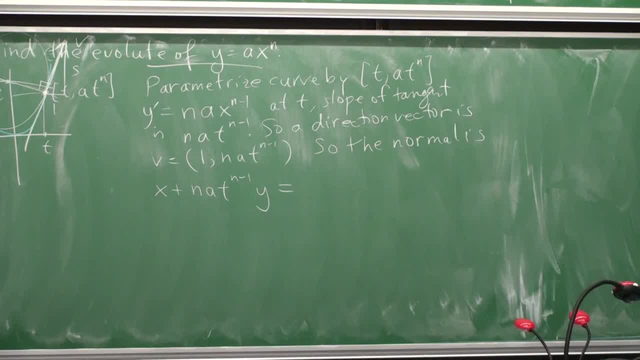 And that's going to be equal to something. And what's it got to be equal? Well, it's got to be a line that goes through the point that we're talking about. So this point has to satisfy the equation of the line. 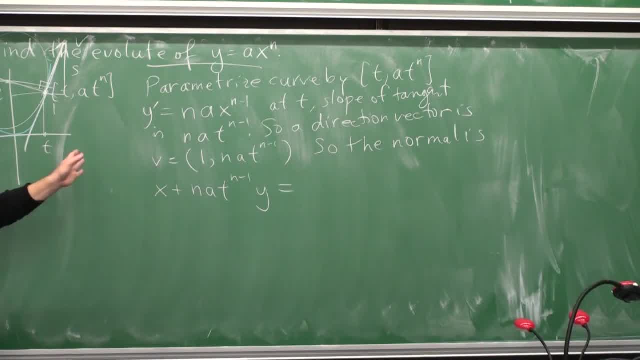 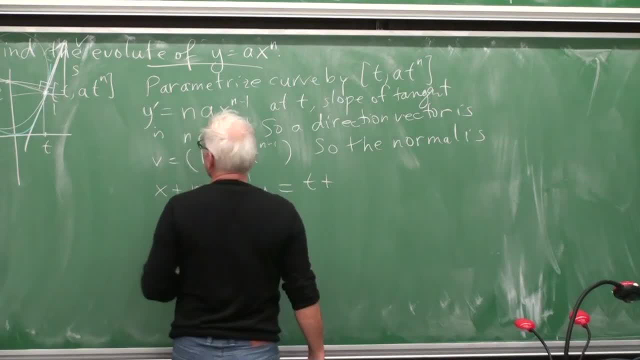 If we plug in x equals t and y equals a to the t to the n, we're going to get what it has to be equal to. So it has to be equal to t, plus I have to replace y with a times t to the n. 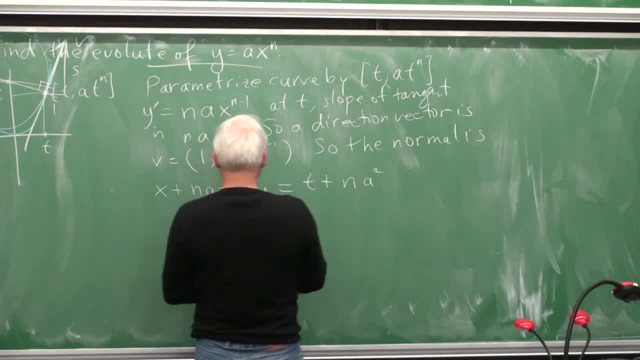 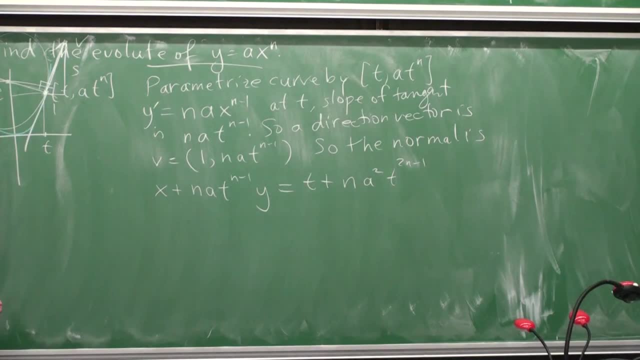 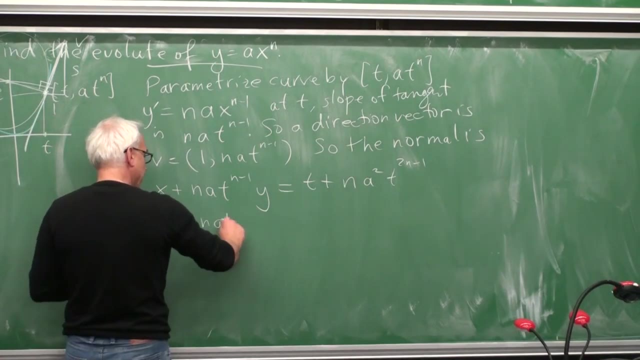 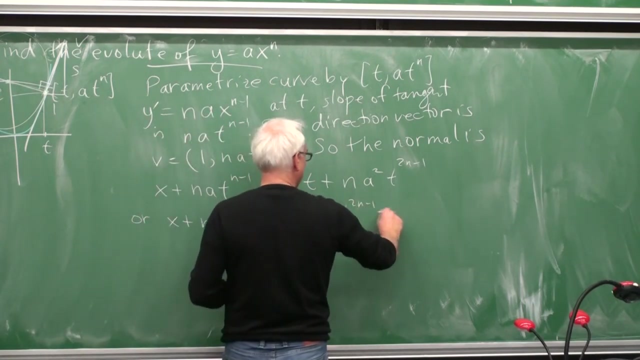 so that'll be n a squared t to the 2n minus 1.. All right, or sometimes, you know, we like to write it with everything on one side. We can do that too. Minus t, minus n. a squared t to the n minus 1 equals 0.. 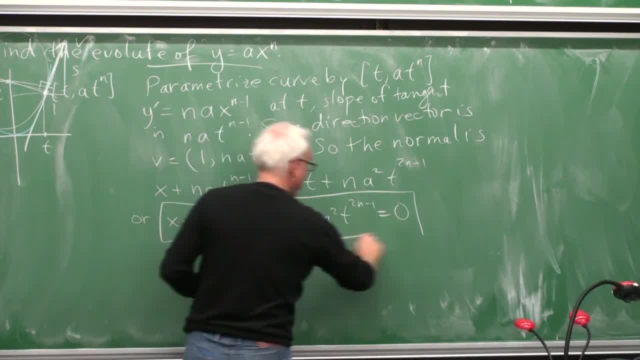 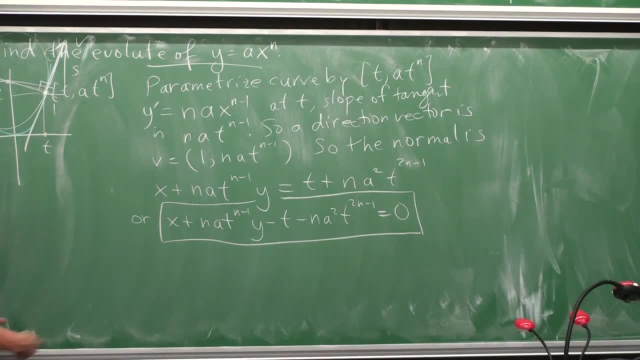 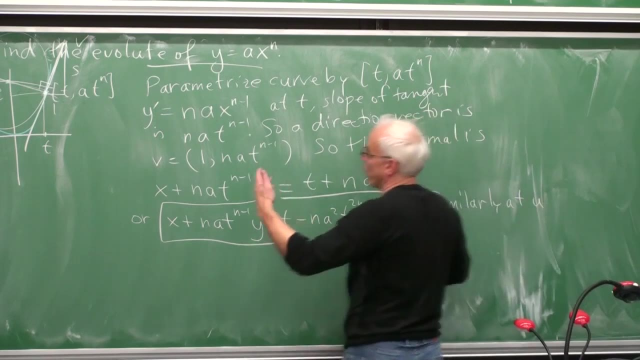 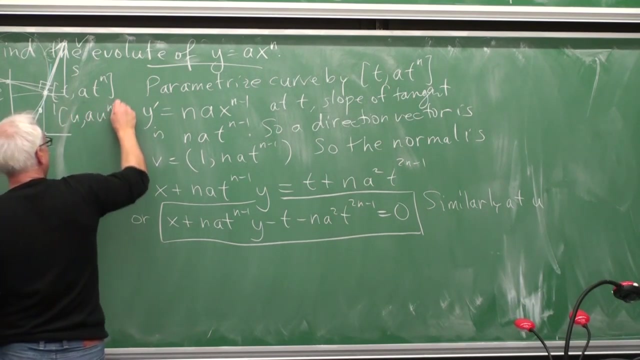 That's an equation of the normal. at the point t, So similarly at point u, at u. so another parameter on the curve, let's say u here, that'll be u and a. u to the n. Similarly, at u, the normal is: 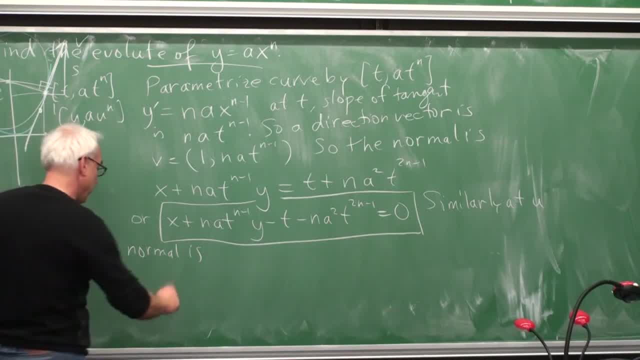 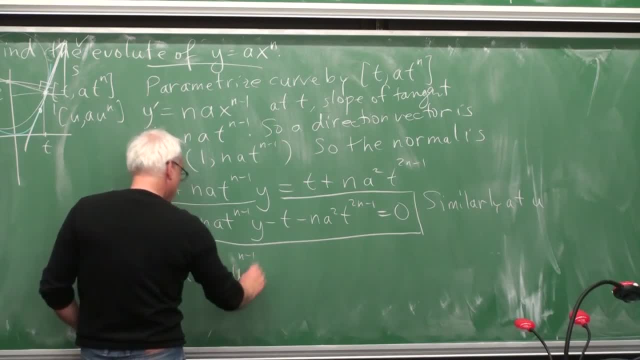 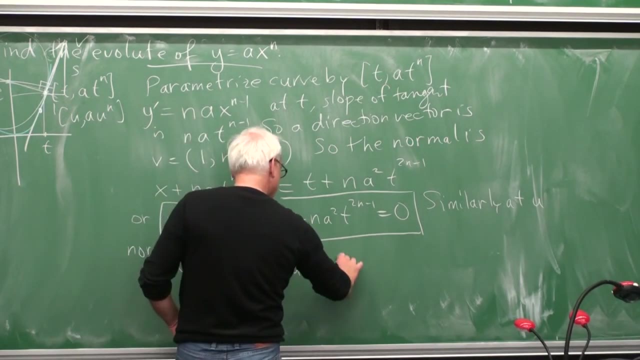 well, it's exactly the same thing with t's replaced with u's, So x plus n a t to the n minus 1,. no, I said t replaced with u, So u to the n minus 1 times y minus u minus n a. squared u to n minus 1 equals 0.. 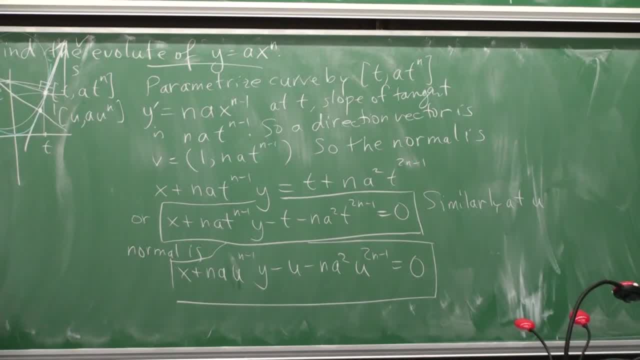 So we have two normals. What we're going to do is we're going to find the common point of intersection and then let u approach t and see where that common point of intersection drifts towards. All right, so how do we solve the intersection of these two lines? 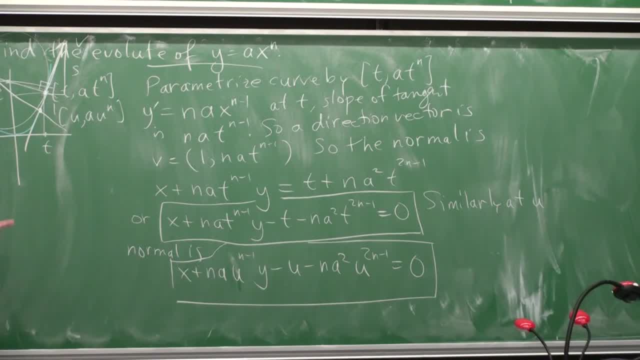 Well, we just have to. you know, these are just two linear equations We have to solve for x and y, two equations in x and y We have to solve. Okay, it's probably simplest just to subtract these equations, because there's an nx here and an x here. 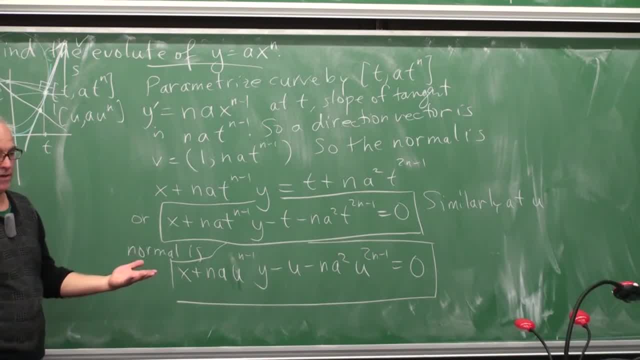 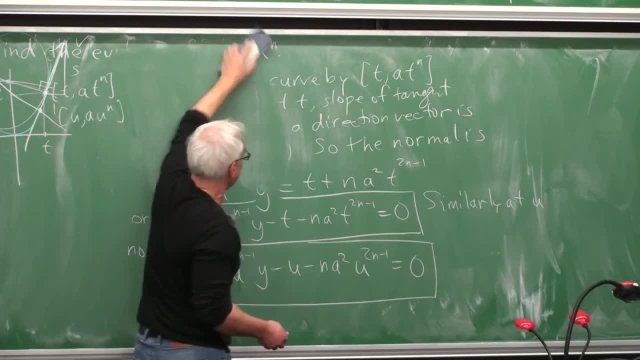 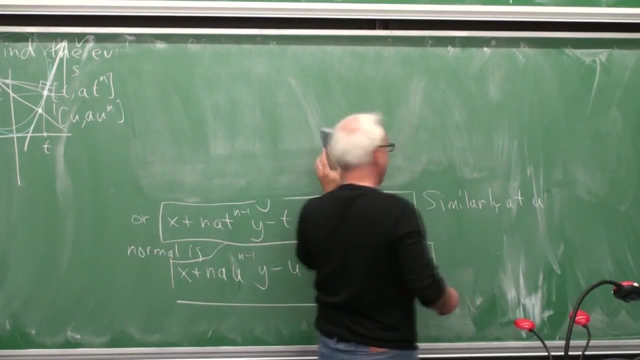 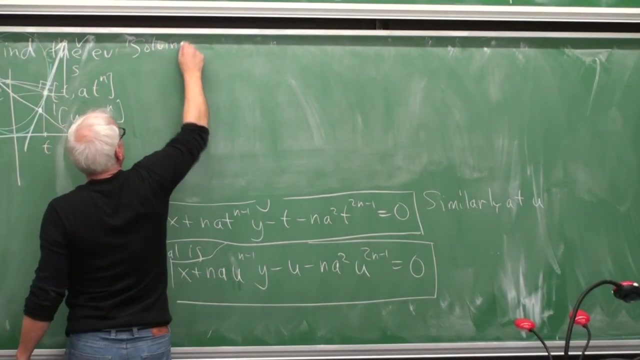 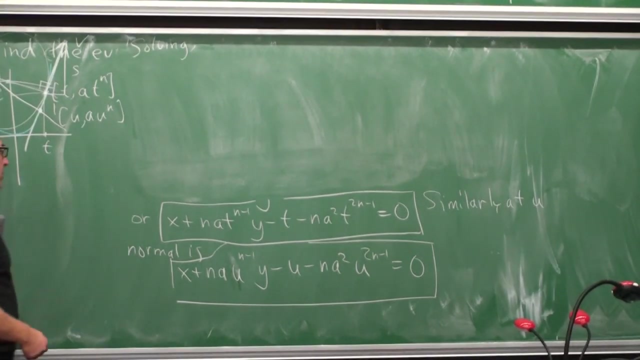 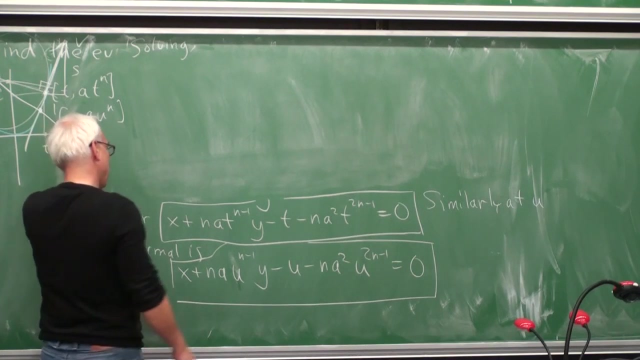 So if we subtract, the x will be gone immediately and we'll just have a single equation in y. That's very simple. So I'll leave them there and go up here. All right, so solving, Solving. Well, what's the best, okay? 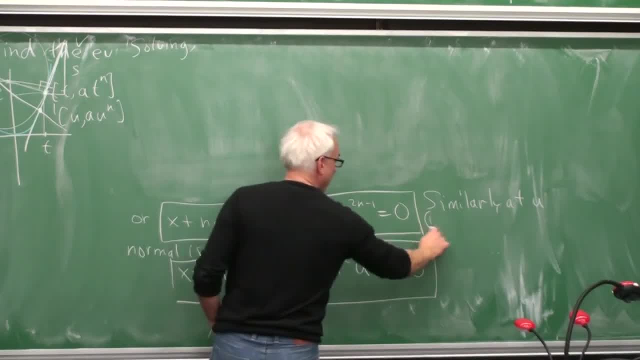 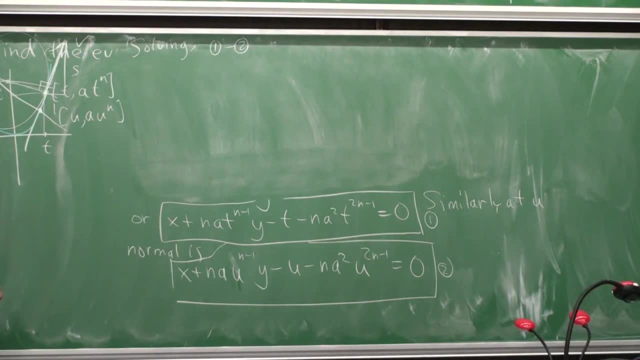 I'll just take the difference. How's that? Okay, I'll take equation 1, equation 2.. So I'll take equation 1 minus equation 2.. What's that do for us? The x's will cancel. We'll have an n. 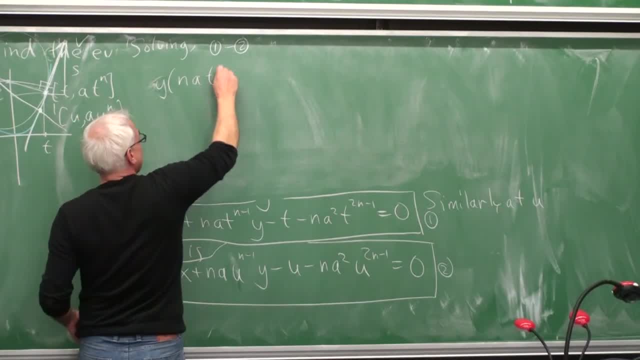 Well, we'll have y times n a t to the n minus 1 on this side, and then we'll have y times n a t to the n minus 1 on this side, minus n a u to the n minus 1 on that side. 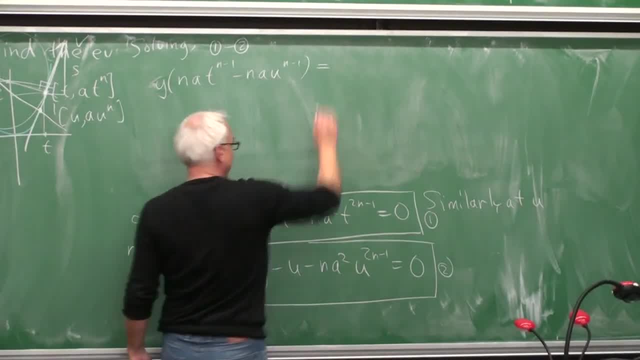 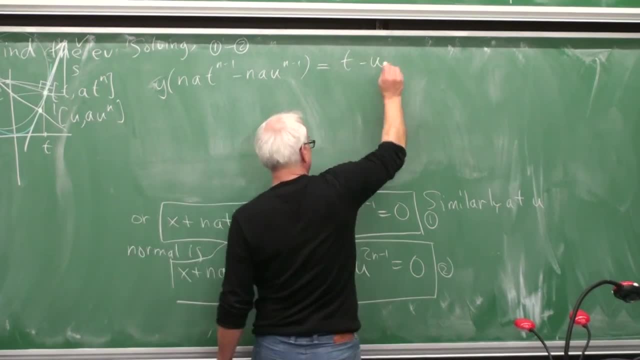 And then probably we should bring everything else to the other side. So equals. so if we bring this stuff here on the other side, we'll have a t and then there'll be a u, and so it'll be t minus u. 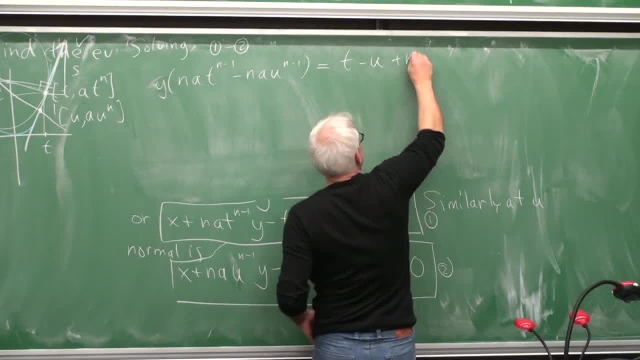 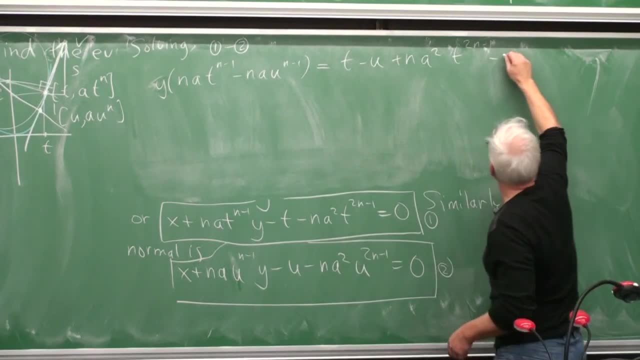 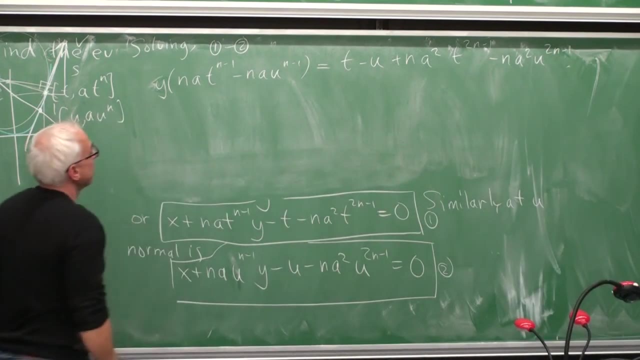 And then we have this: n a squared t, so plus n a squared t to the 2n minus 1, and then there'll be a minus. similarly n a squared u 2 to the n minus 1.. So I guess we can just solve for y by just dividing by this. 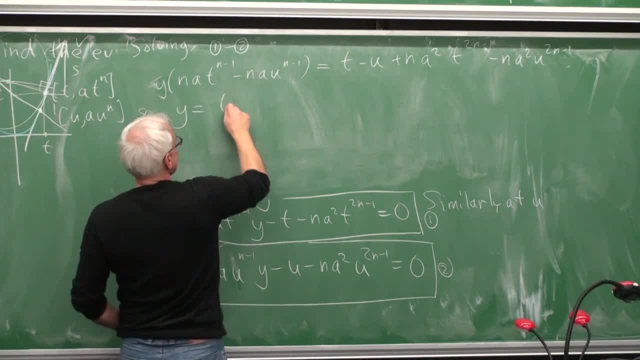 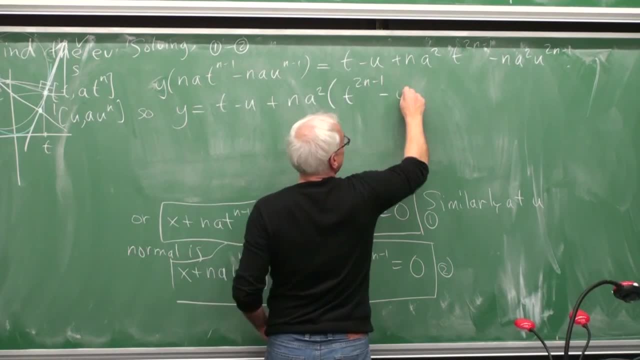 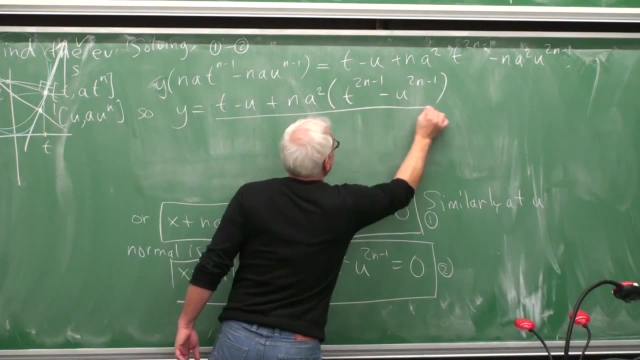 so y equals- and we'll try to factor things- so there's a t minus u and then there's an n a squared times t to the 2n minus 1 minus u to the 2n minus 1.. Divided by the coefficient of y, here 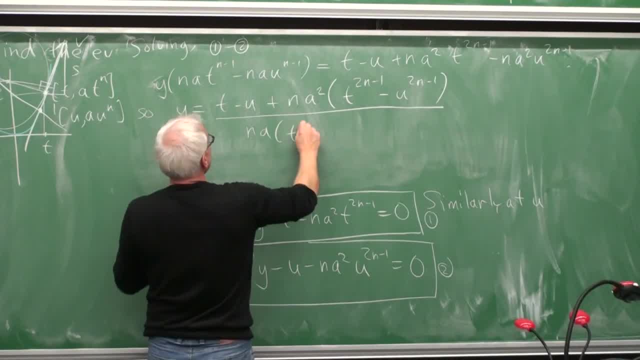 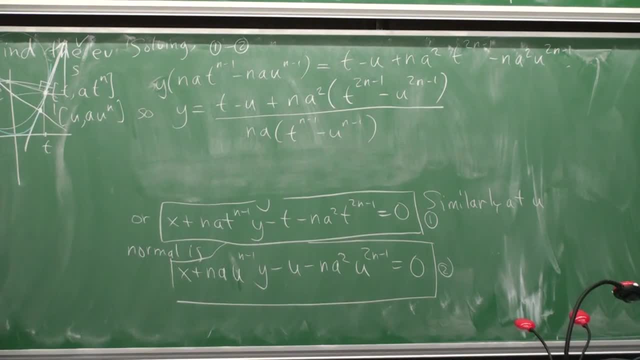 there's an n a. that's a common factor- and there's a t to the n minus 1, minus u to the n minus 1.. Alright, so it's easy to make a little mistake, so let's just check that we haven't done that. 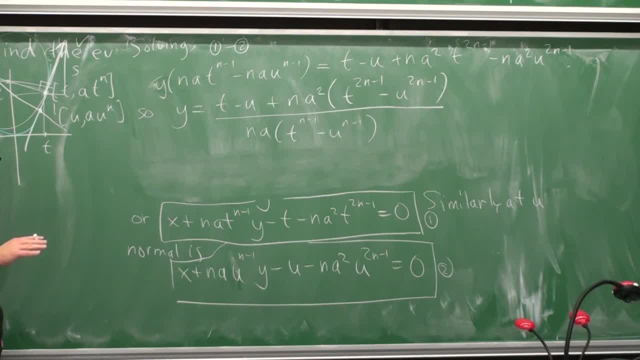 Okay, it's very good to go slowly and to check that you've done every step right, because you make a little mistake, then you mess up your entire calculation, then you have to find it later and it causes you all kinds of extra work. 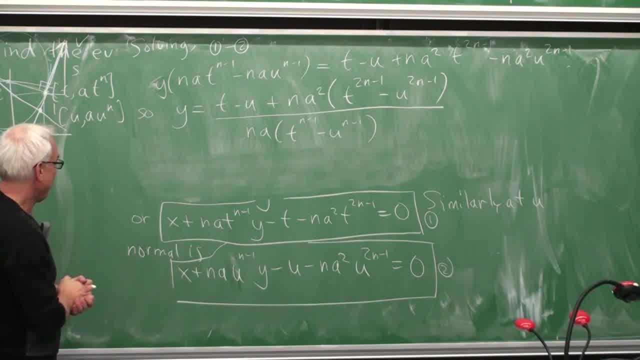 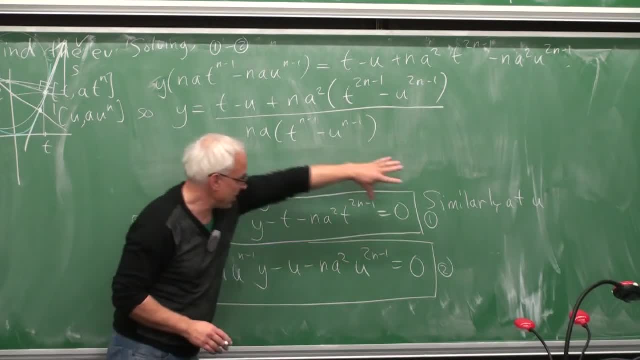 So have we done that right? So we've taken this equation minus this equation. the x's have cancelled this minus this gave us that, and then we took this to the other side and we had to subtract this to the other side. 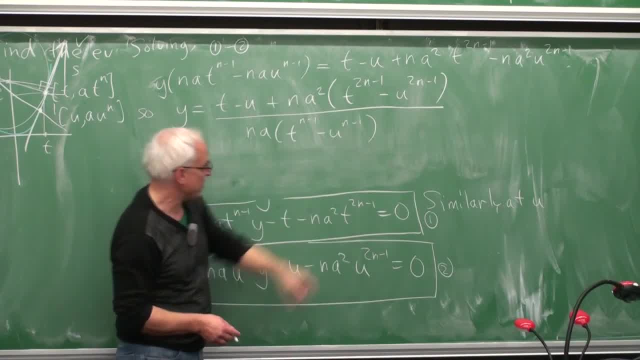 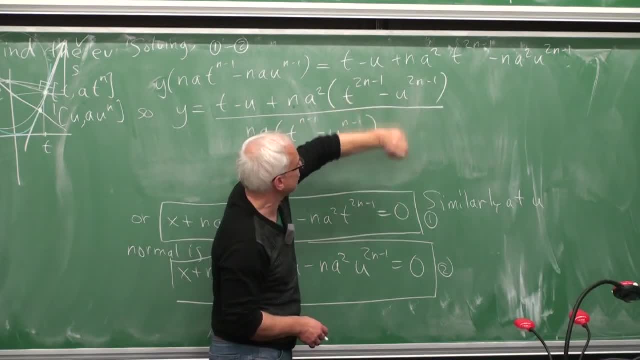 So t minus u, and this was with a plus sign, and then this one was with a minus sign, And then we took a factor of n a squared out of there and we had a t to the 2n minus 1, minus u to the 2n minus 1,. 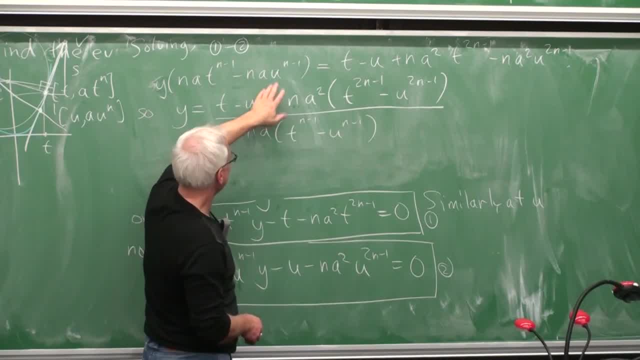 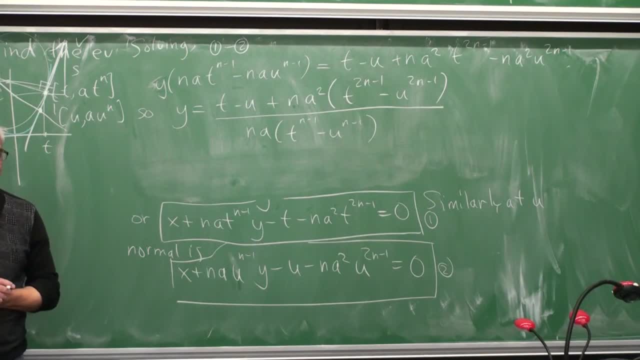 and down here we factored n a t to the n minus 1, u to the n minus 1.. Okay, that looks about reasonable, All right. now we have to ask what happens as u approaches t. Well, obviously there's a bit of a problem. 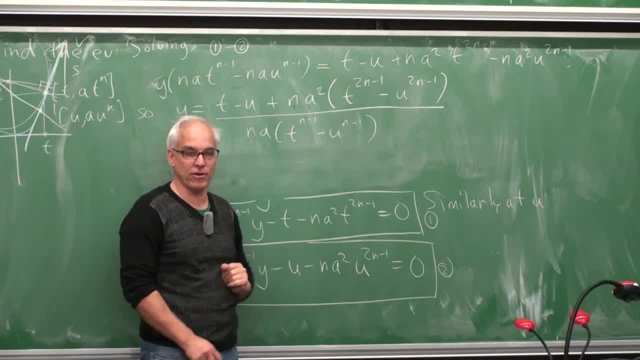 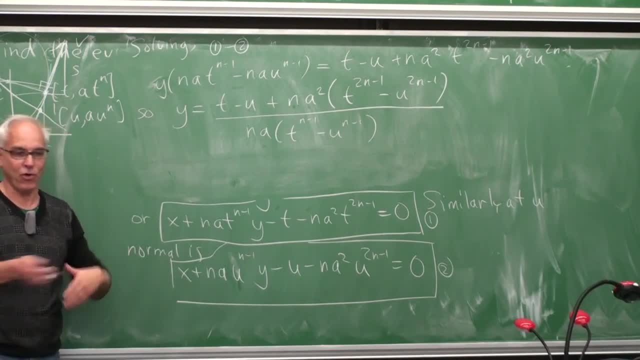 because everything goes to 0. This goes to 0, that goes to 0, that goes to 0. Now, if you have done calculus, you know that this is not such a problem. There's something called L'Hopital's rule. 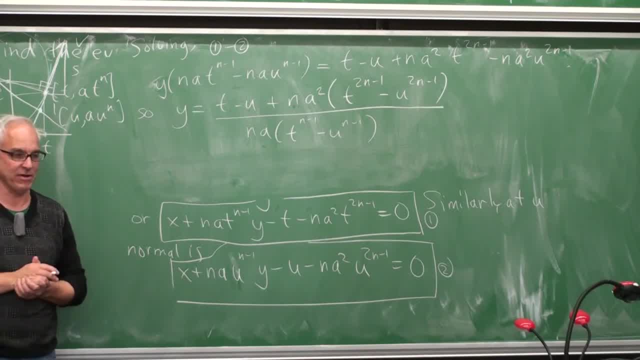 and we could differentiate things appropriately and get some kind of limit. But it's also useful to think a little bit more elementarily and say: well, how could we do this if we didn't know calculus and L'Hopital's rule? 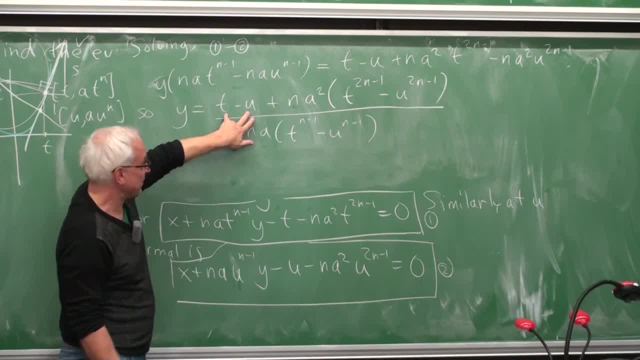 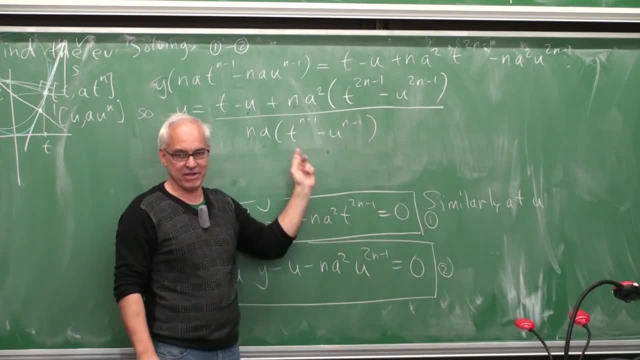 Well, what we notice is there's a factor of t minus u here, and there's really factors of t minus u here and here. The problem of this- everything going to 0- is because of these factors of t minus u that are actually around. 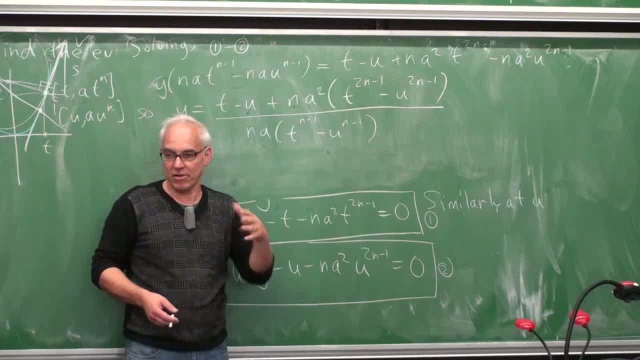 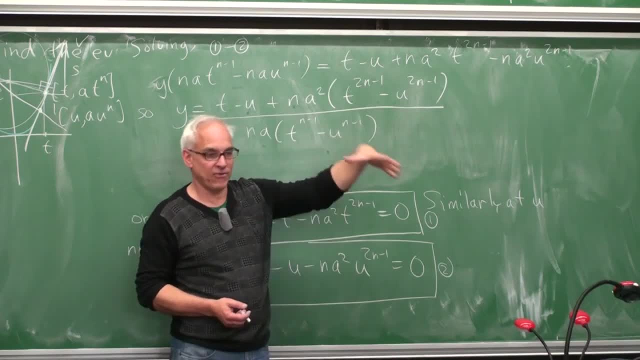 So why don't we just identify what those factors are and then cancel them at the top and the bottom and get rid of them? Okay, That requires us to know that this thing factors as t minus u times something else. So we need an algebraic identity. 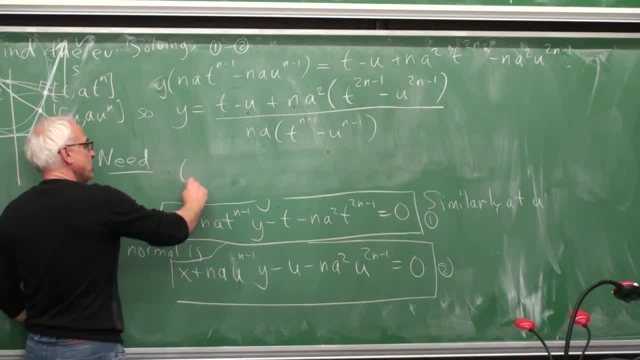 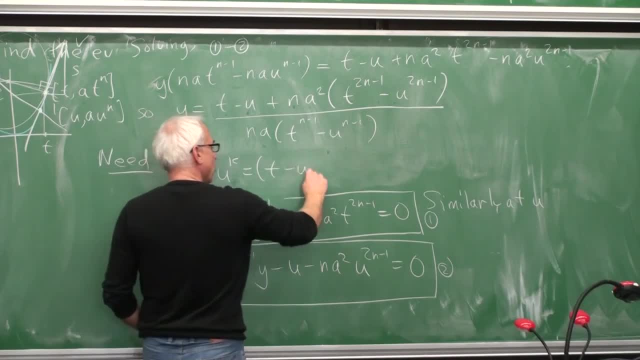 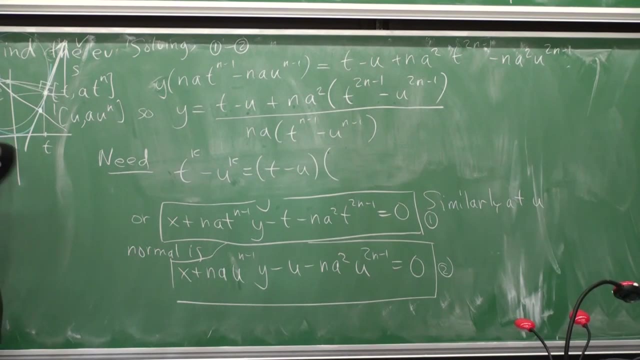 We need to know that. let me just say it a little bit more generally: that t to the say k minus u to the k equals t minus u, times something It factors, And this is the kind of thing that should be known by all undergraduates. 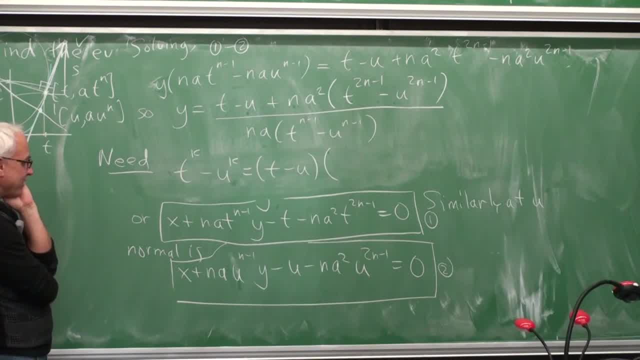 but it perhaps isn't. It is, It is Good. I'm glad to hear that. Okay, so how do we extract the factor? Well, we just sort of do it term by term. We need a t to the k here. 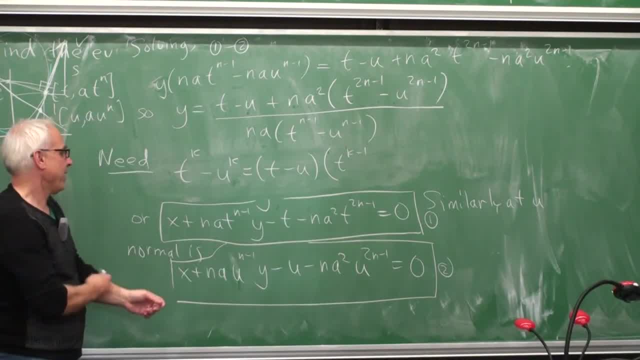 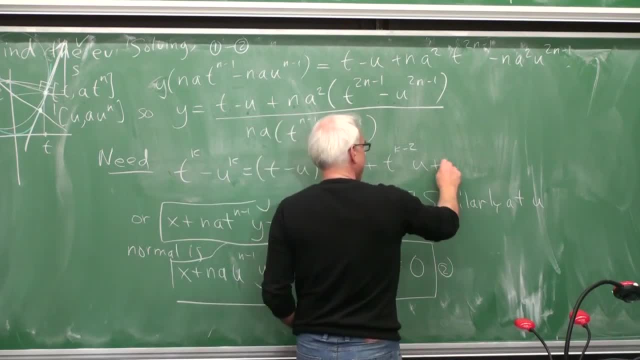 so this had better be t to the k minus 1.. And then the next one's going to be plus t to the k minus 2 times u. And then we keep on going. The powers of t decrease, the powers of u increase. 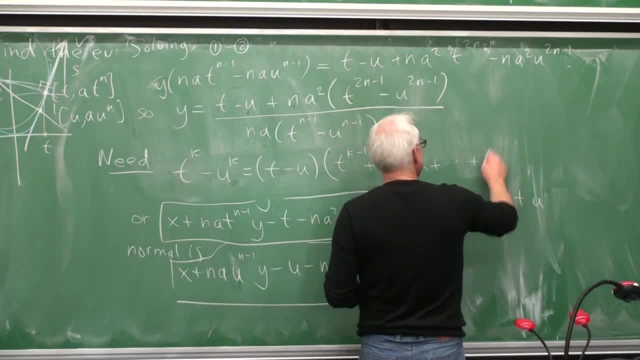 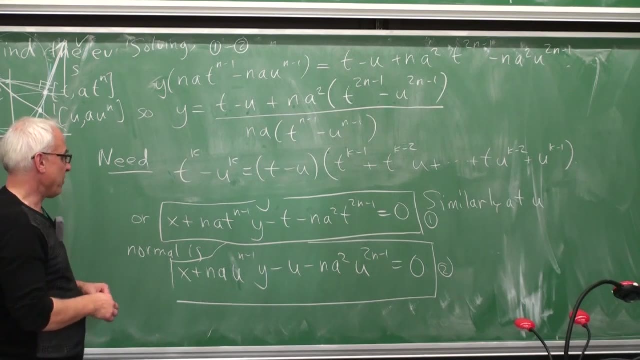 until the second last one will be t times u to the k minus 2, and the very last one will be u to the k minus 1.. This is not really such an unfamiliar formula. It's really just the geometric series formula in disguise. 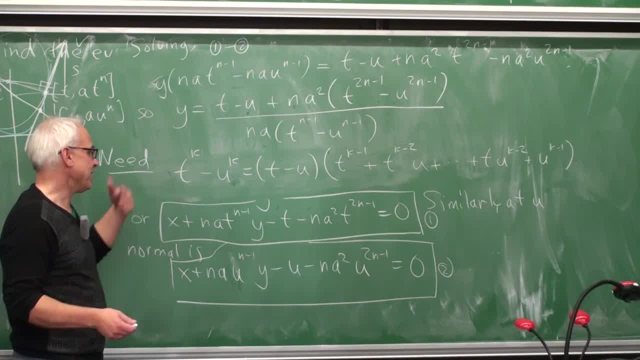 Okay, if you think what happens if, say, t equals 1, if t equals 1, this is just the geometric series formula. It's really the formula 1 minus u to the k over 1 minus u equals 1 plus u plus u, squared. 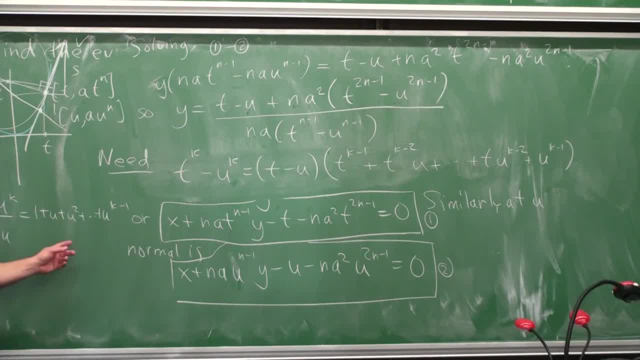 all the way up to u, to the k minus 1.. And, conversely, if you remember this one and you want this one, it's just a question of replacing u with a over b or l over m, or something like that, and then you can extract that one. 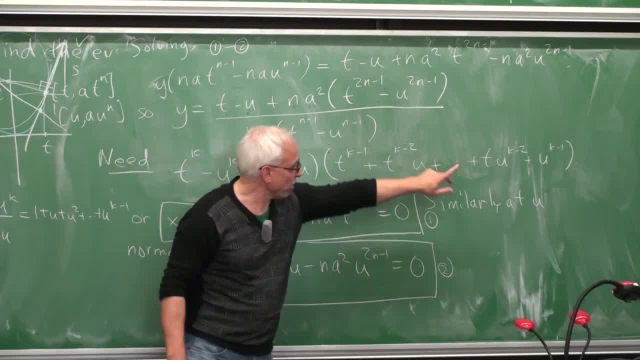 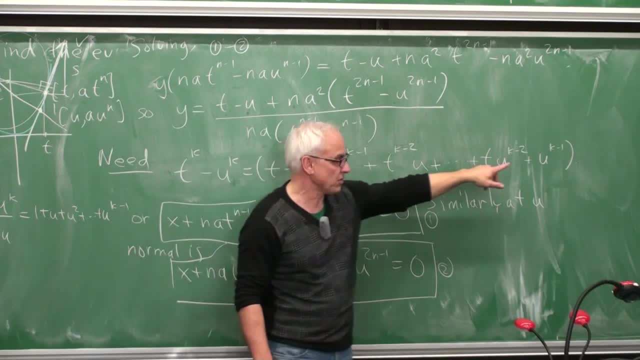 Okay, so that's good. So one more thing to remark here. how many terms are there here? So there's a. if we're thinking about powers of u, we're going from u to the 0 all the way up to u, to the k minus 1.. 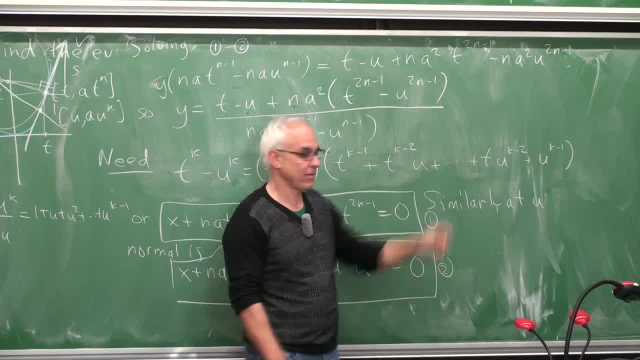 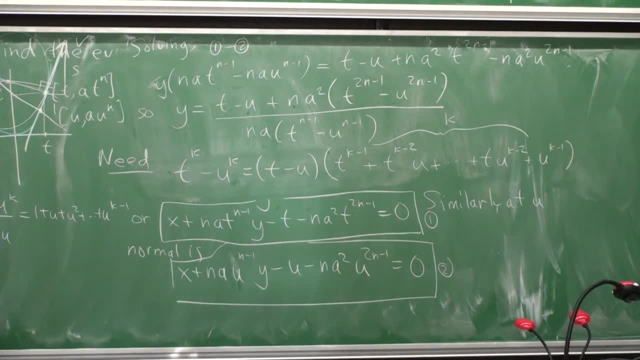 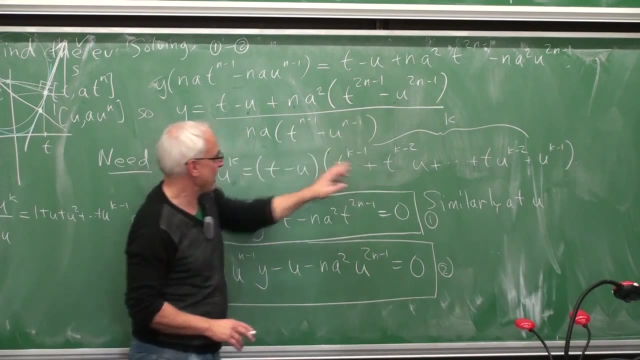 So they're all together k terms. That's going to be important for us in a second. All right, do we buy that? All right, so now, having that at our disposal, we can replace this thing with something like this. We can replace the thing down here: 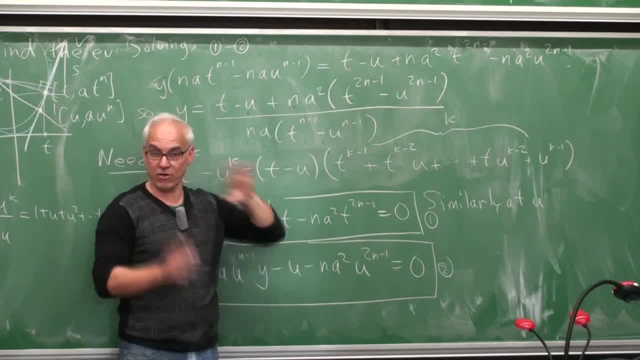 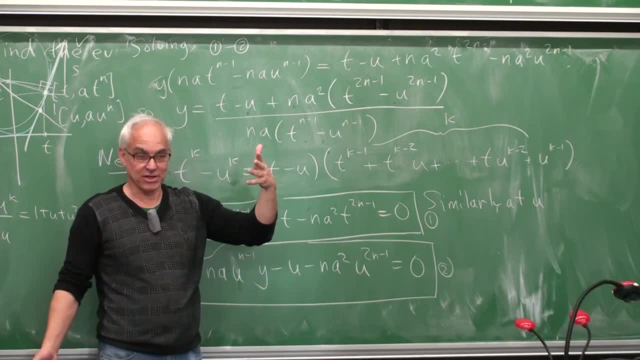 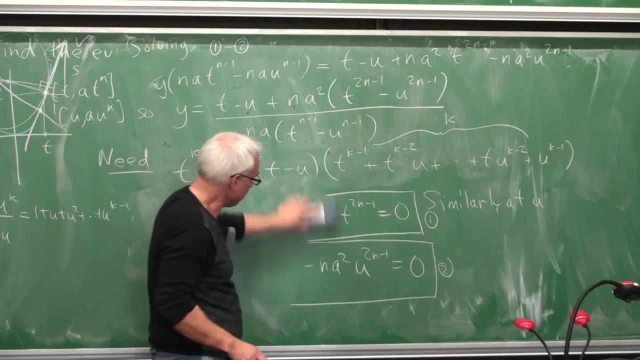 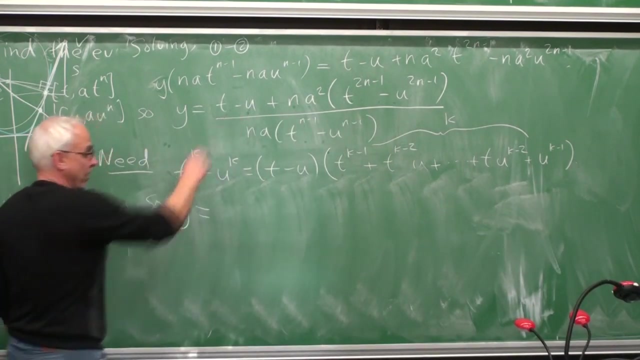 with something like this, and then there'll be this common factor of t minus u everywhere that we can just drop before we take the limit. That'll make it much easier to take the limit. All right, so let's do that. So let's just rewrite this thing. 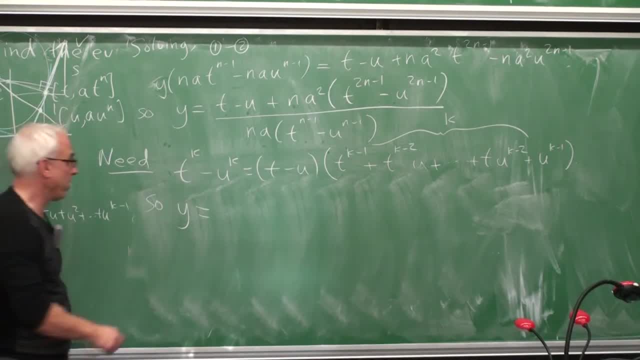 and I'm going to cancel that t minus u that's going to appear everywhere. So I'm going to have on the top 1 plus n a squared Now instead of this thing. I had to replace it with something like this, but I have to remember that the power here is 2n minus 1,. 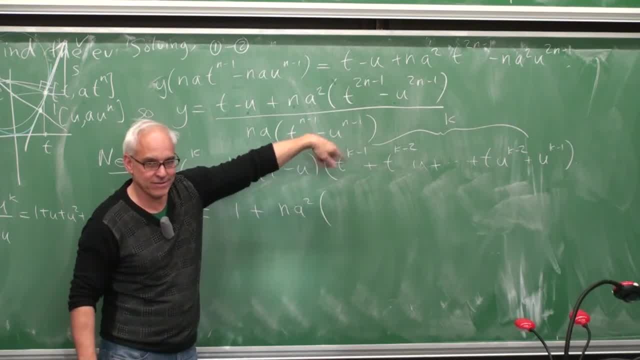 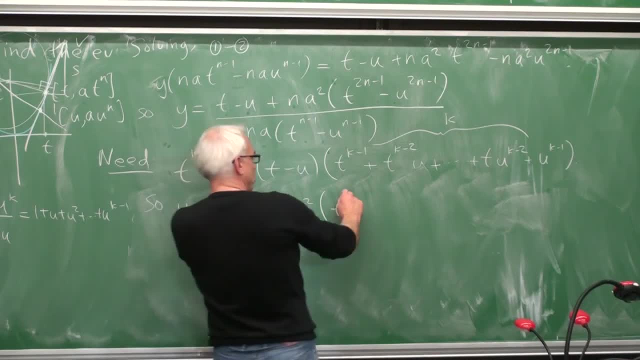 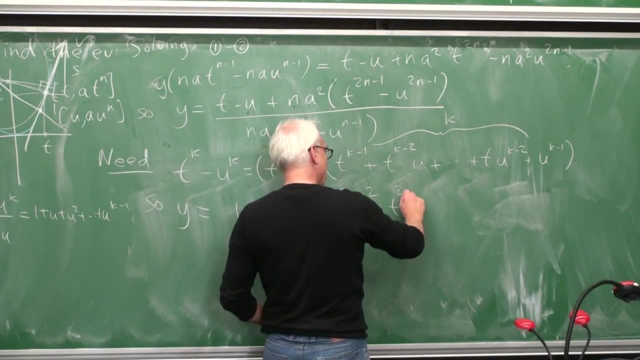 so I have to write the appropriate series here. So I have to start with t to the 2n minus 2,, 2n minus 2, and decrease in powers of t- 2n minus 1 times u, and then to go all the way up to the last one. 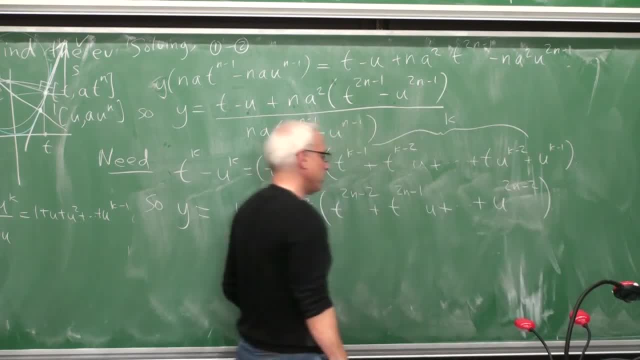 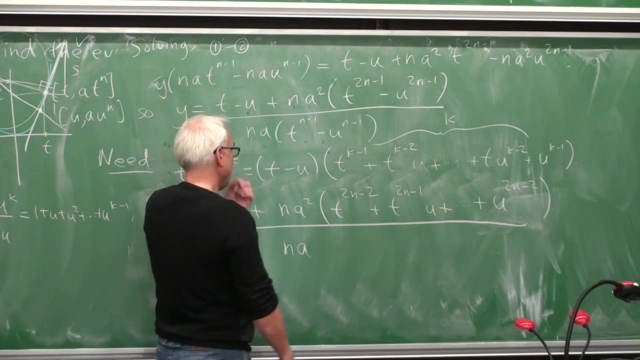 u to the 2n minus 2.. And on the bottom, we had n times a same kind of story Down here. Oh, thank you. yes, 2n minus 2, that's right, This should be 2n minus 3.. 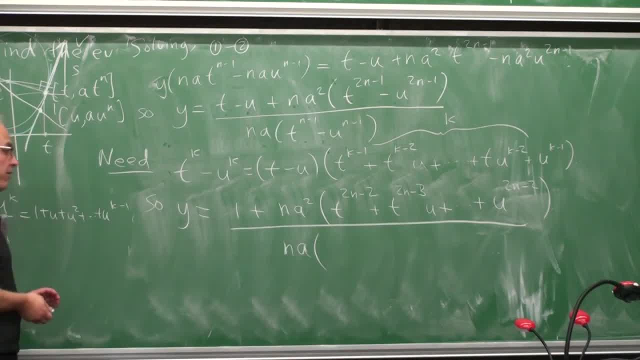 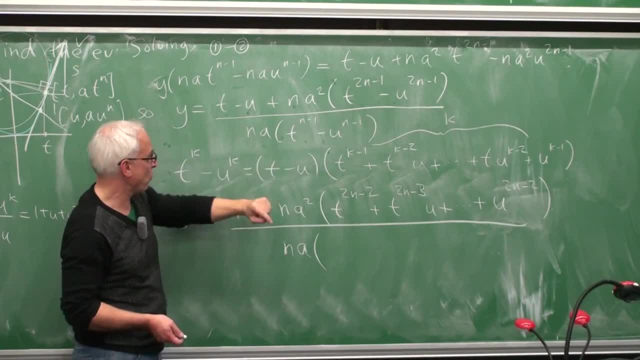 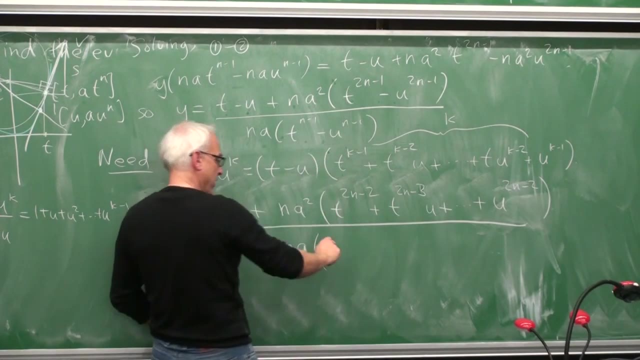 The powers of t are going down and the powers of u are going up. thanks, Okay, we're doing the same kind of thing over here. same expression. Now we're starting with n minus 1 instead of k, So the first term that we'll get will be n minus 1 minus 1,. 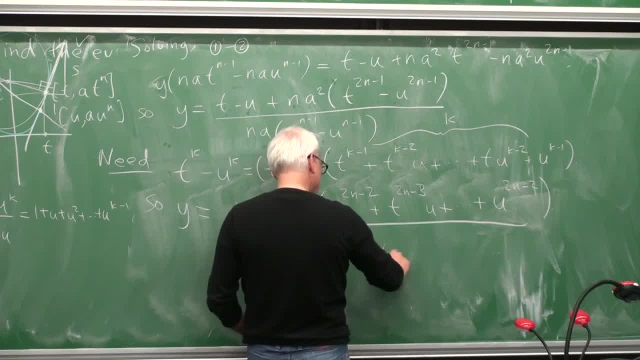 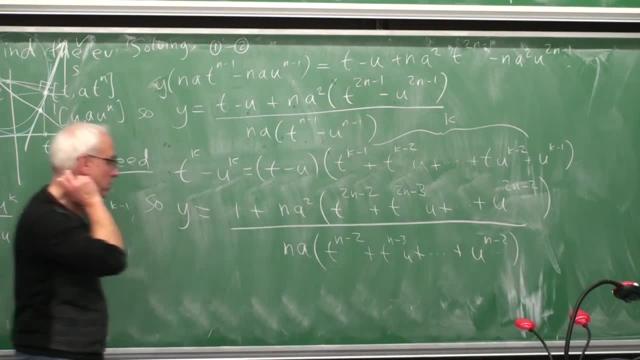 which I guess is n minus 2.. And then the t's go down t to the n minus 3 times u, and the u's go up until finally we get u to the n minus 2.. All right, now we can let t approach u. 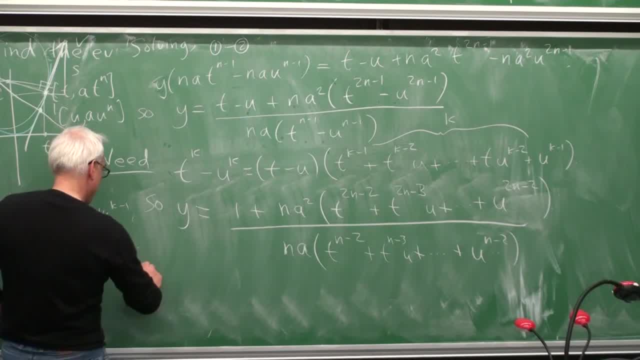 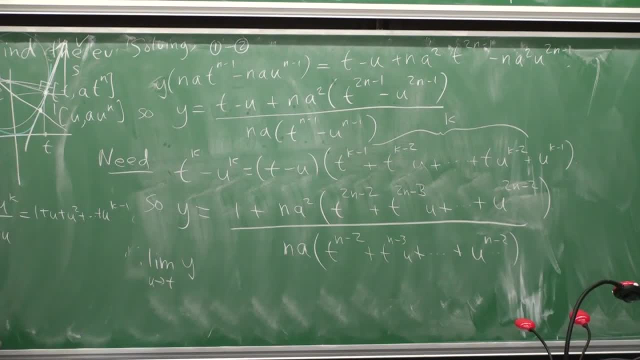 And we can say what we get. So now, the limit, therefore the limit of y, as say u, approaches t, we'll do everything in terms of t. What's going to happen? So, all over, we're just going to set all the u's equal to t's. 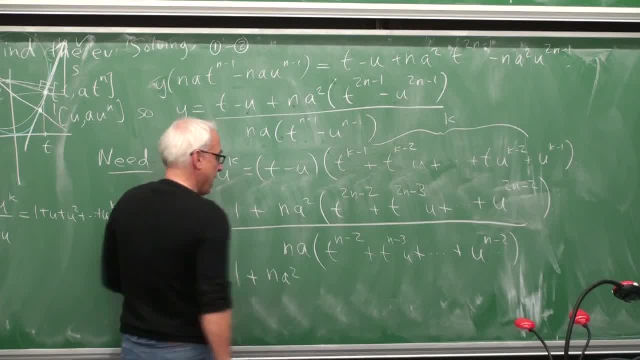 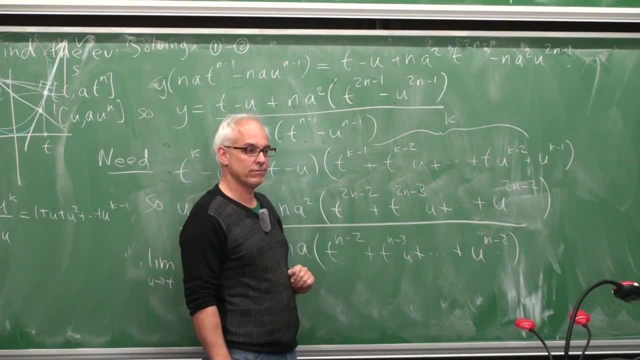 So we get 1 plus n, a squared. what's going to happen here? All these terms are going to be exactly the same. They're all going to be t to the 2n minus 2, because we're setting u equal to t. 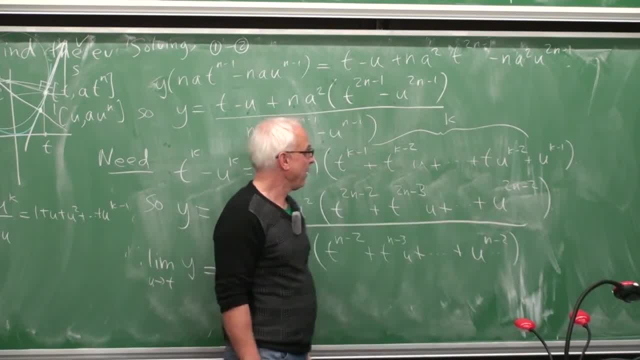 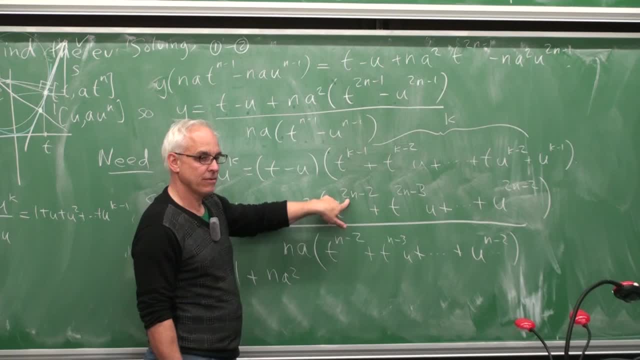 So the only question is, how many of them are there? Okay, and we said that there is sort of one more than the first power here. All right, if it starts with k minus 1, then they're all together k terms. So they're all together here: 2n minus 1 terms. 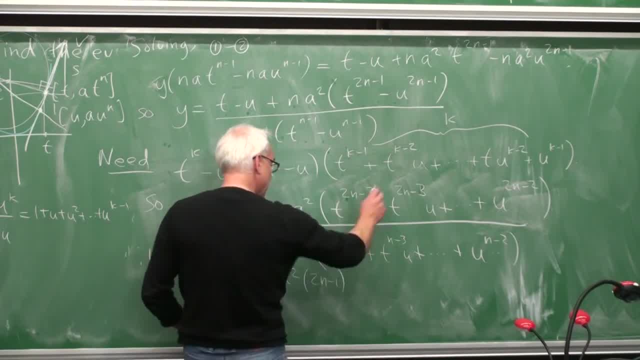 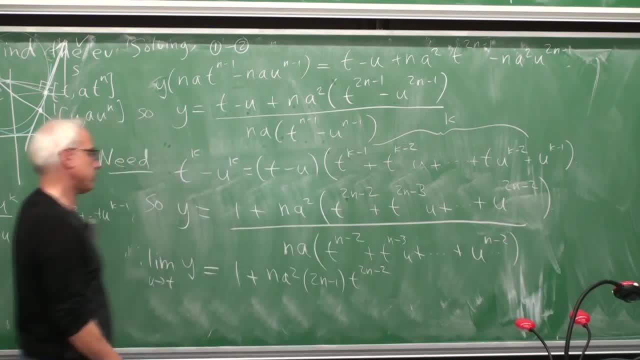 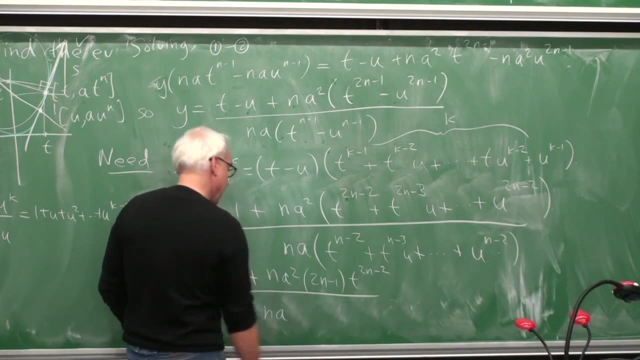 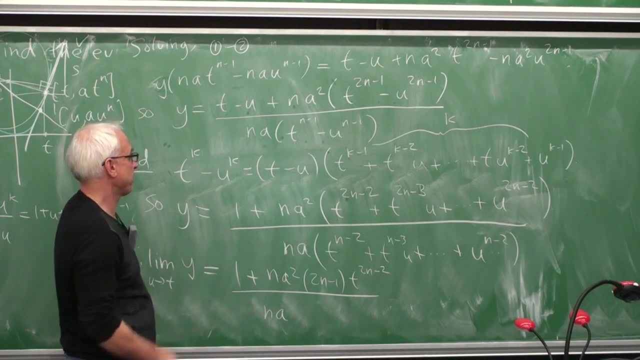 So we have to factor 2n minus 1 here, and each of the terms is actually t, to the 2n minus 2.. It's in the numerator And the denominator is a similar kind of story n times a. How many terms do we have here? 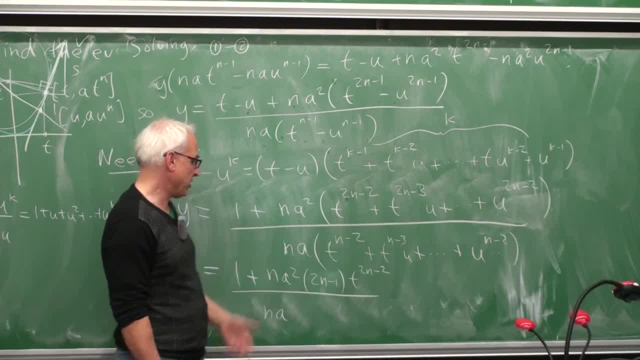 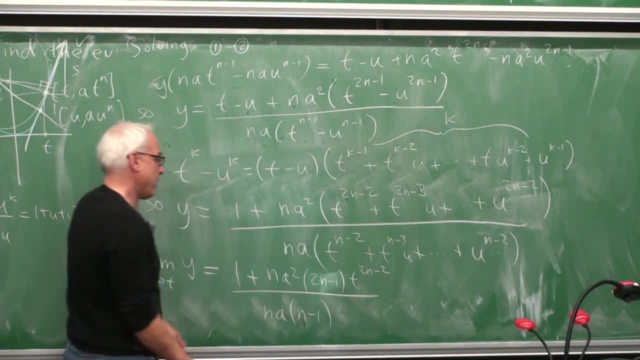 So we have to take this first thing and add 1.. So there's n minus 2 here, so we have to add 1 to that. so n minus 1, n minus 1 there, And the common terms are all t to the n minus 2.. 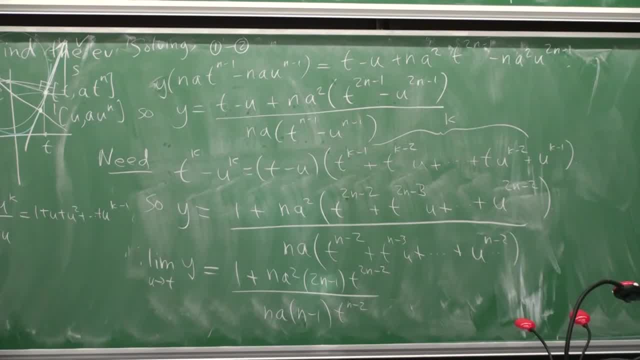 All right, that's what y is. That's an expression for y in terms of t. That also involves a, of course, and it also involves n. Okay, so what do we need more? Well, we still need x, of course. 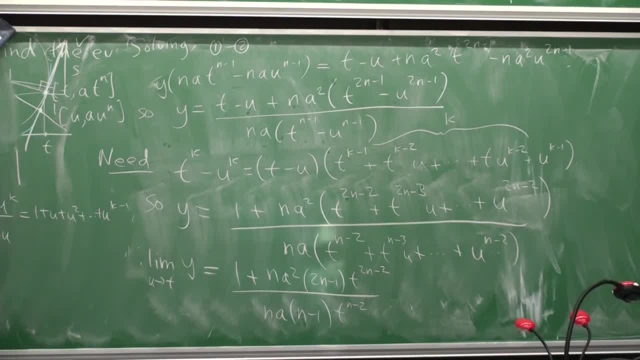 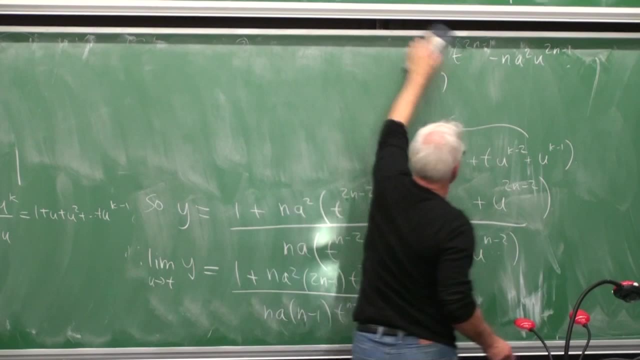 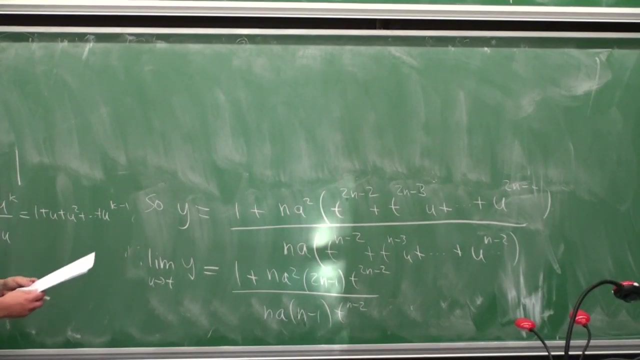 And how are we going to get x? Well, we had a relation between x and y because they lie on these tangent lines, on these normal lines. So I've rubbed it off, but we can perhaps resuscitate it. What was the relation? 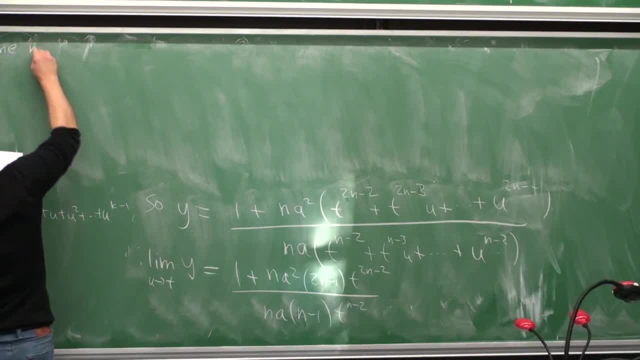 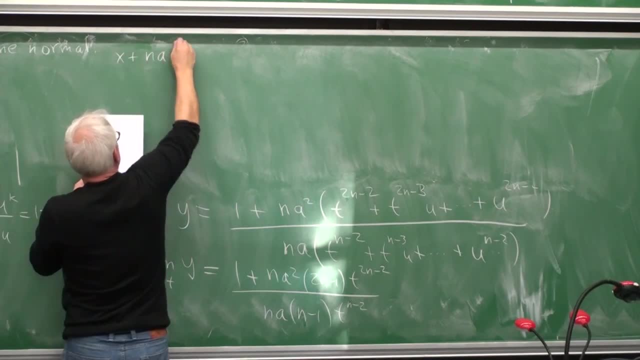 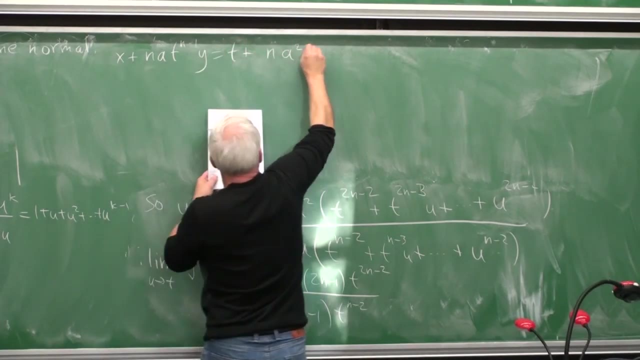 So one of the normals, I guess the first one was x plus n a t to the n minus 1 times y equals t plus n a squared t to the 2n minus 1.. So therefore, if we know x, if we know y, 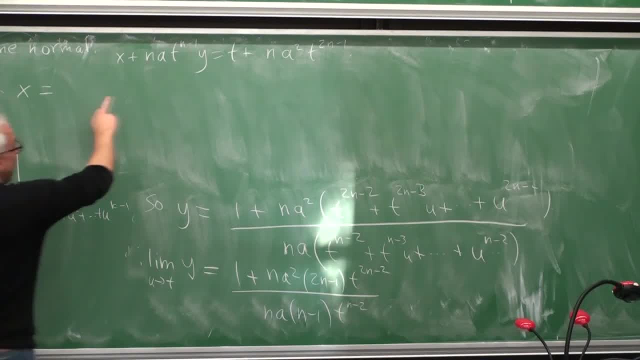 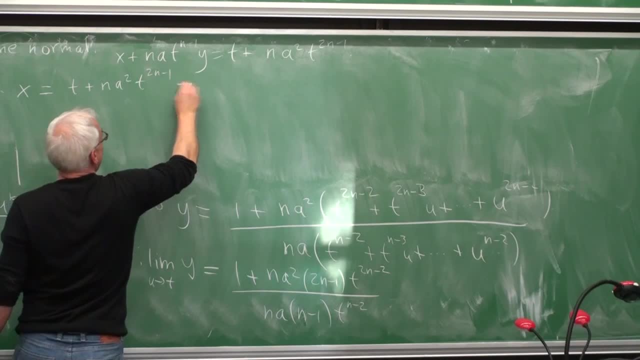 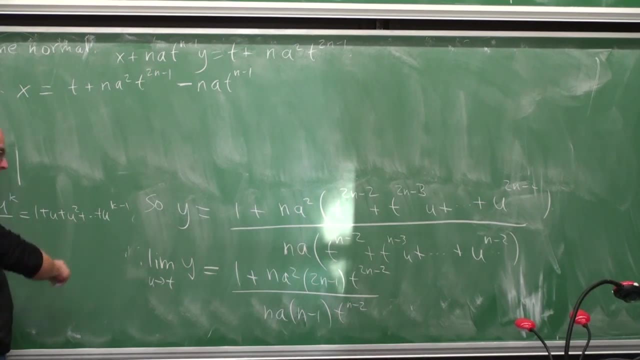 we know x, We can solve for x. We'll take: x equals t plus n. a squared t to the 2n minus 1 minus n. a t to the n minus 1.. t to the n minus 1 times this value of y. 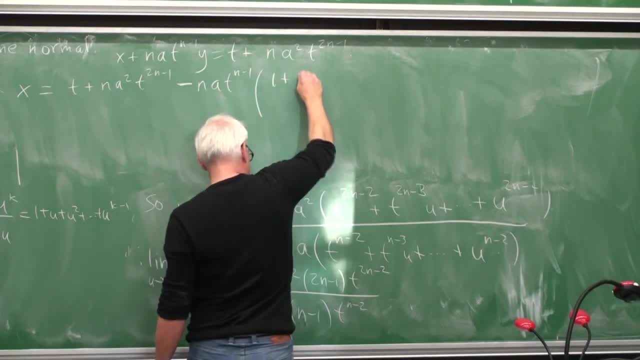 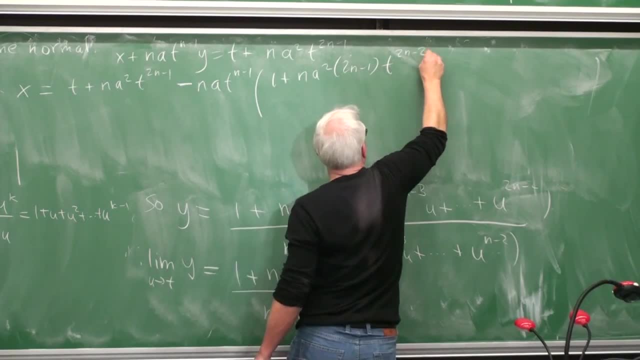 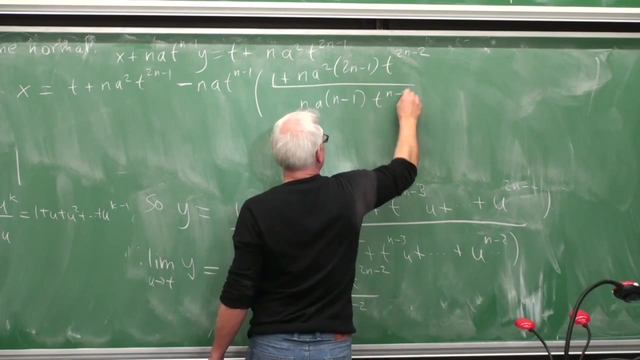 And that is 1 plus n a squared times 2n minus 1 t to the 2n minus 2, all over n a n minus 1 t to the n minus 2.. And again we better check that we haven't made. 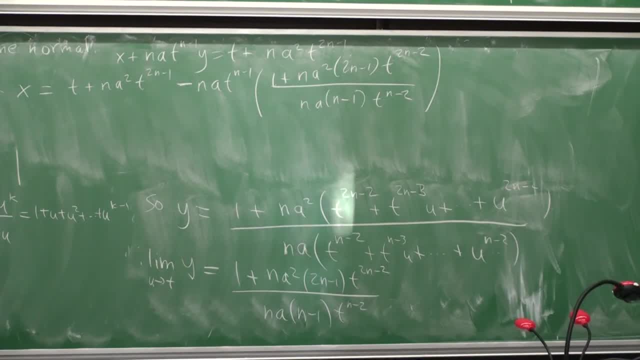 a transcribing error. I guess that looks right. I've copied y there And here. I've just copied n a t, squared t then and subtracted n a t to the n minus 1.. All right, So we have to simplify this, of course. 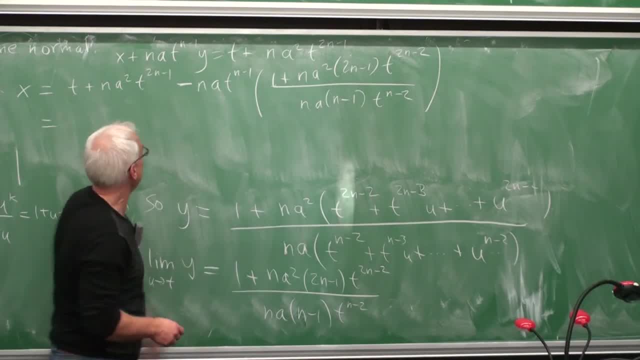 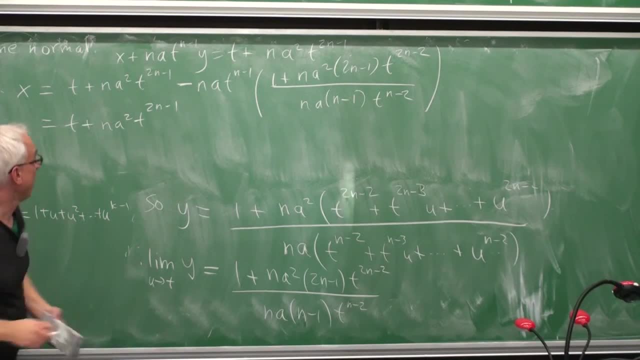 There'll be a bit of cancellation here, because there's an n a, there's a power of t, So we'll get t plus n a squared t to the 2n minus 1.. We're going to remember that this is y all right. 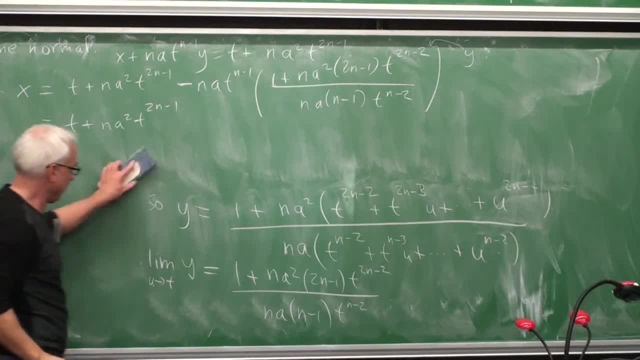 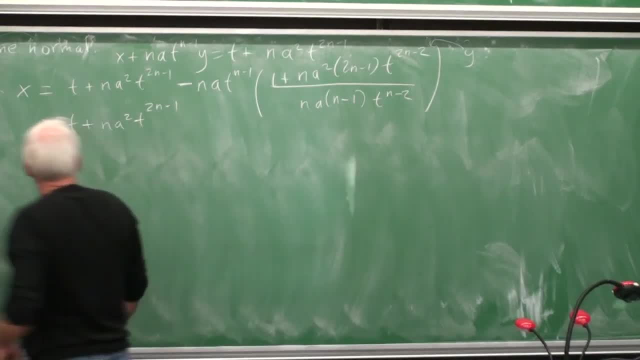 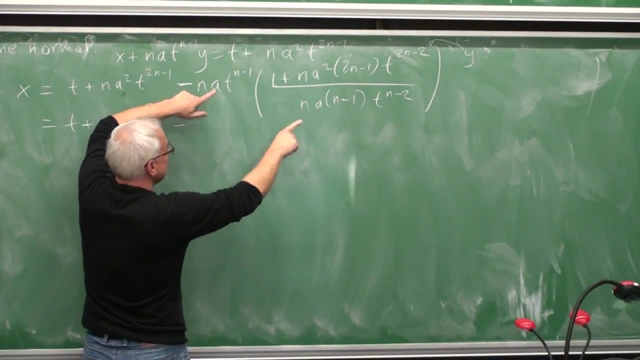 This is y here. I'm going to rub all this out to give us some space. OK, we have repeated that and now I have to subtract n. a cancels The t to the n minus 1s cancel. There'll be one more up here, so there'll be a t factor left. 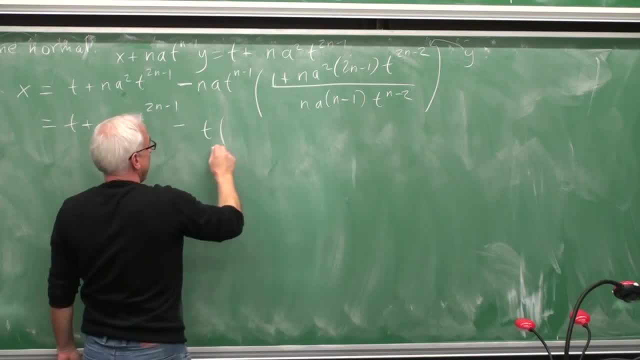 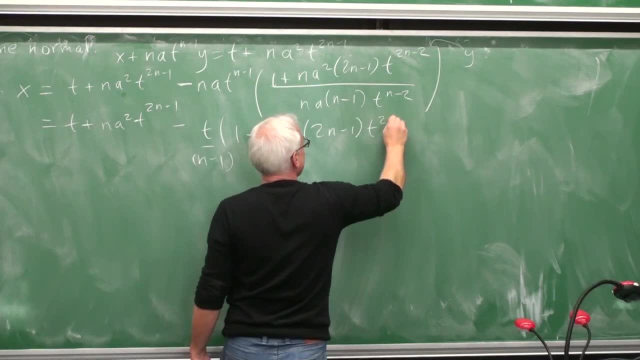 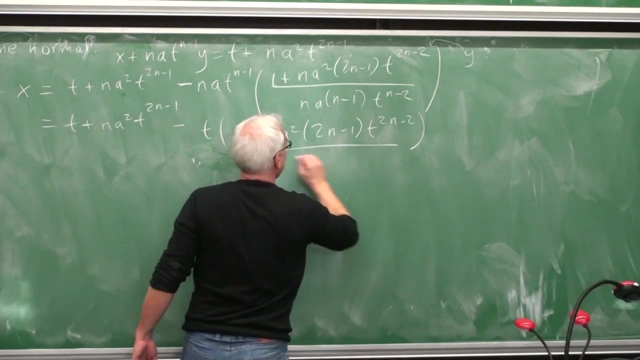 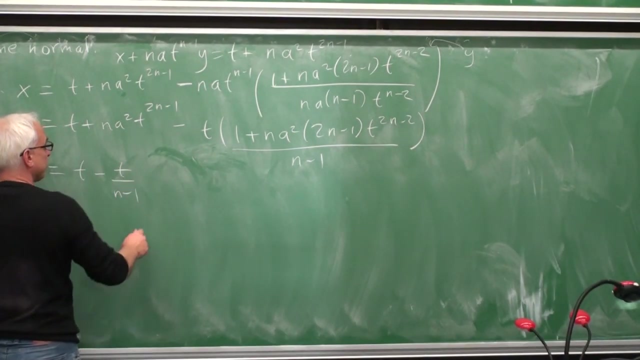 There'll be an n minus 1 on the bottom and a 1 plus n, a squared 2n minus 1 t to the 2n minus 2.. Maybe I could put that all over n minus 1.. OK, so I'm getting t minus t over n minus 1.. 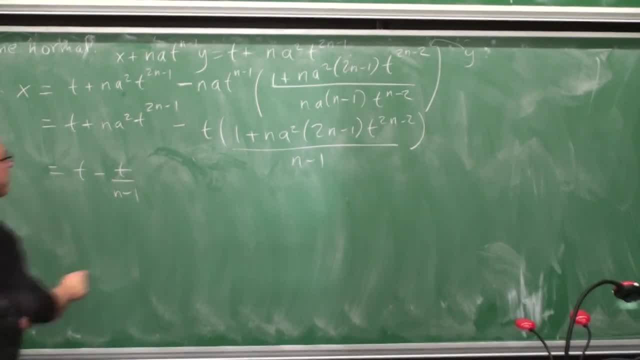 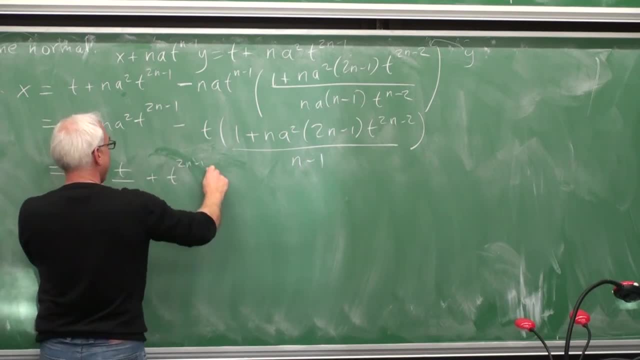 So the first term, And then There'll be a certain number of, actually 2 to the n minus 1.. t to the 2n minus 1, times n, times a squared times 1. from here I'm just taking that factor out. 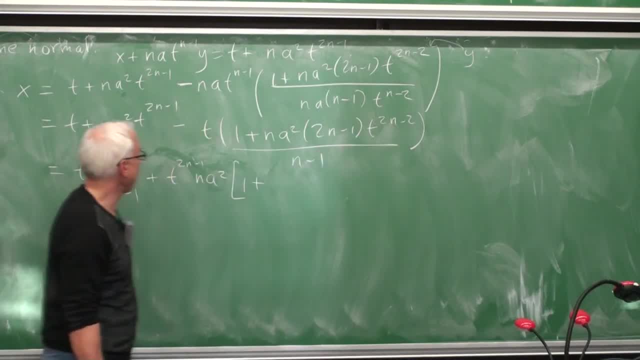 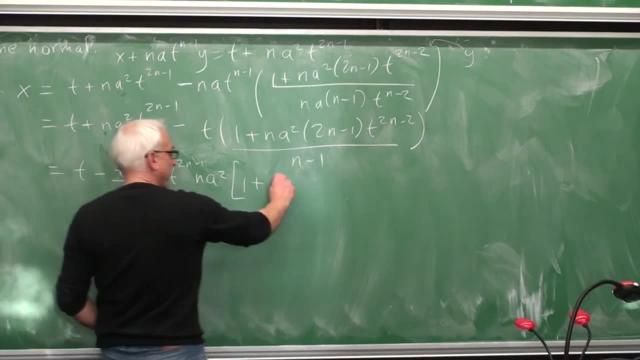 And when I multiply this t here, I'm going to get 2 to the n minus 1.. That's the same power of t. There's an n a squared. I'm going to pull that out. I think I have 2n minus 1 left. 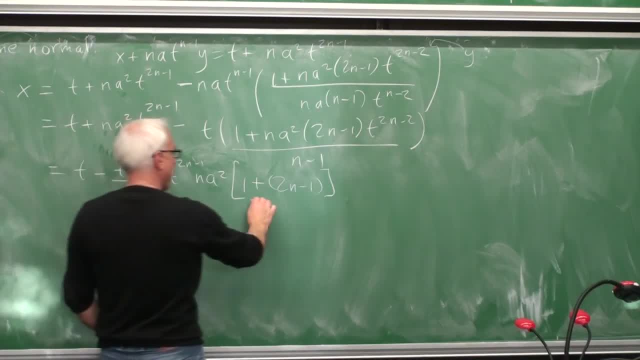 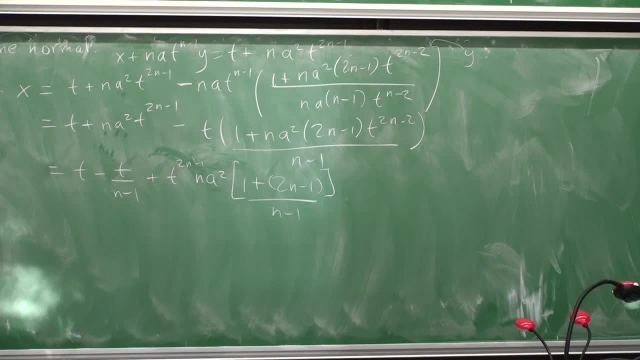 All divided by n minus 1.. Did you buy that n a squared t to the 2n minus 1.. I've multiplied the t times that 1 already and brought that out. Now it's just t times this. So 2 to the n minus t to the 2n minus 1 is exactly the same thing as this one here. 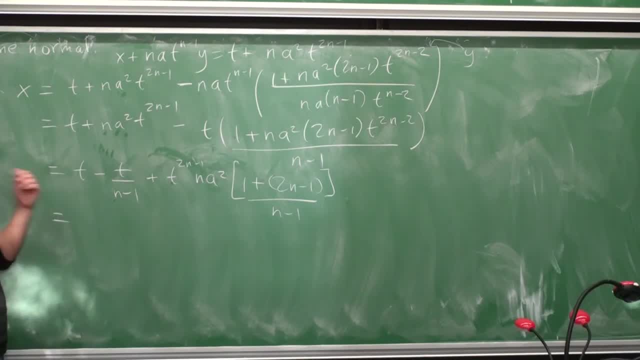 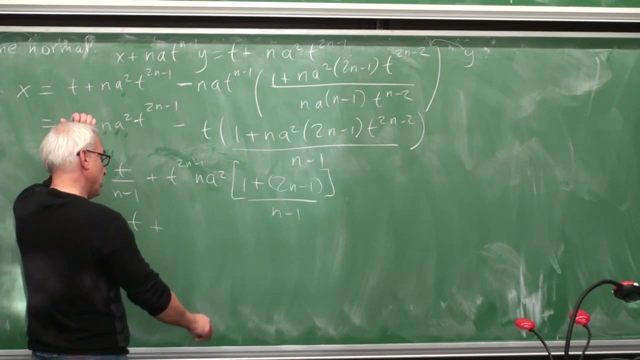 OK, looks reasonable, OK. so what is this now? This here is n minus 1 minus 1.. So that's n minus 2 all over, n minus 1 times t, And this is plus. 1 minus 1 is 0.. 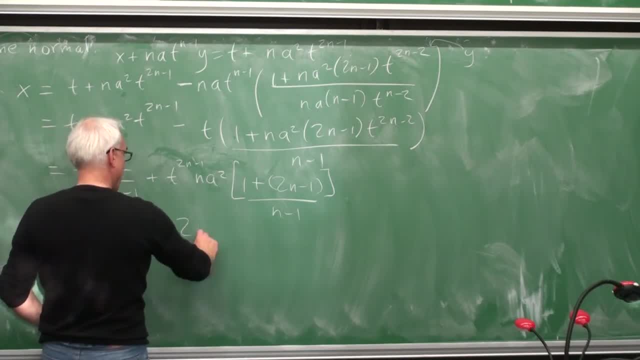 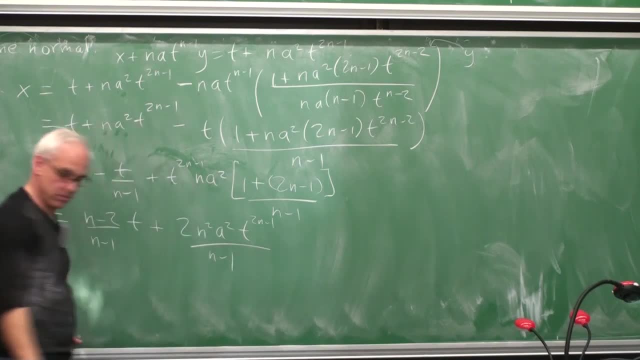 2n is another n here. 2n squared a squared t to the 2n minus 1. all over n minus 1.. No, no, no, I made a mistake. I made a mistake. What did I make a mistake? 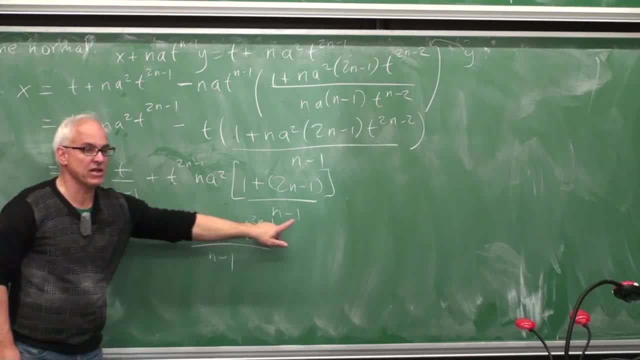 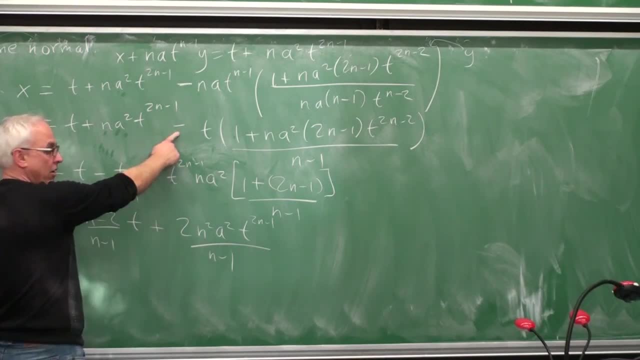 When I put everything over the common factor, there was an n minus 1 down here And there's also a minus sign here, isn't there? Oh, my goodness, Very important to check things. Don't trust yourself. first time around. Third time around, OK. 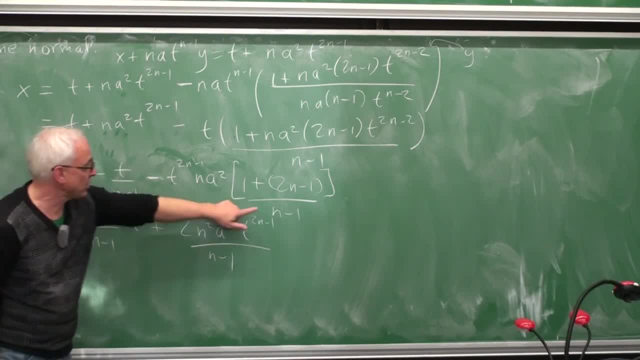 So there's a minus sign that I forgot. What else did I do? When I take everything over a common denominator, there's an n minus 1. that's under here, So I need to multiply this thing by n minus 1 as well. 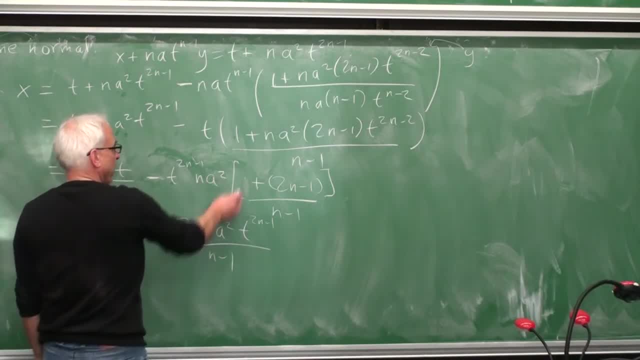 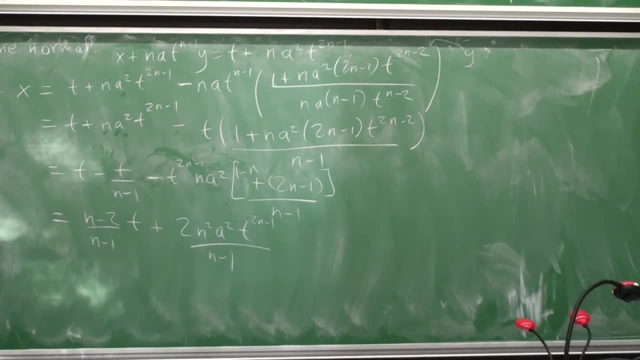 So instead of having a 1 here, there should have been an n minus 1.. But with a minus sign it's actually 1 minus n. Should have been a 1 minus n there, And that means that that 1 and that 1 minus 1 cancel. 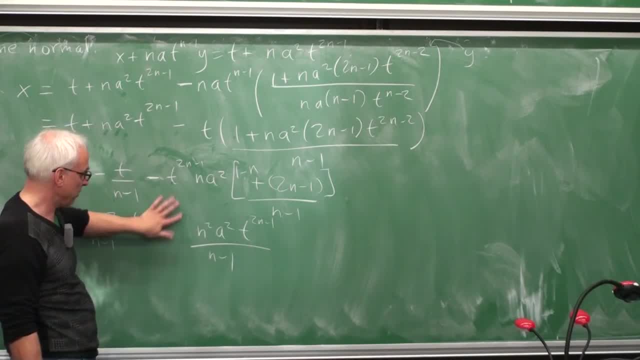 And that 2n and the minus n just give me a single n. There's no 2 here And there should be a minus sign. So we have n minus 2 over n minus 1 times t minus n, squared a squared t to the 2n minus 1 over n minus 1.. 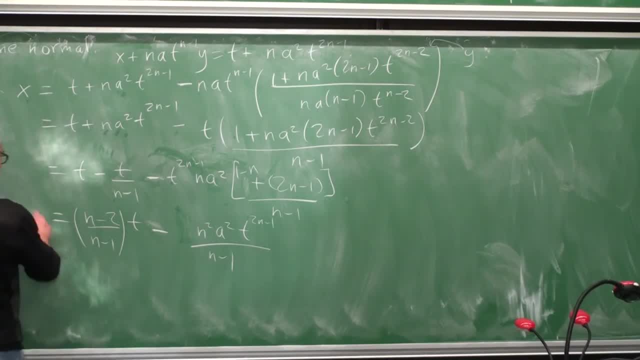 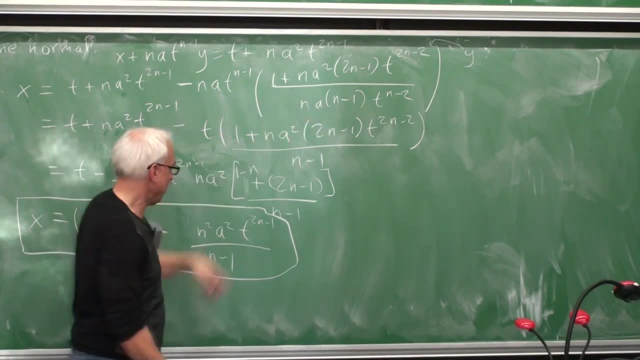 And all of that is equal to the x coefficient, So I might put that in a box And y we already have. I think y was exactly this thing here, So I'll put it over here. y equals 1 plus n minus 1.. 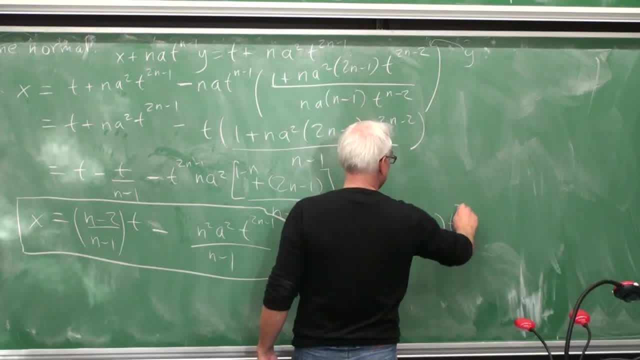 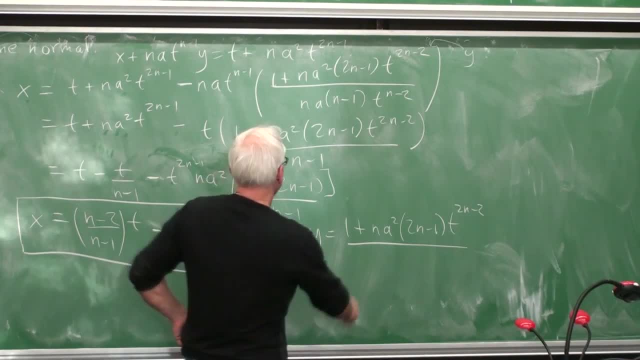 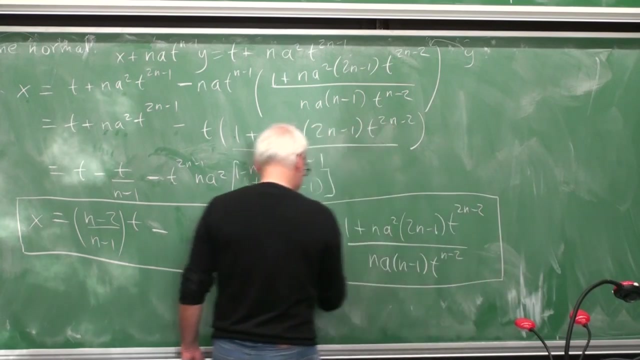 a squared 2n minus 1 t to the 2n minus 2. all over, That was all y, wasn't it? n times a times n minus 1 t to the n minus 2.. All right, Something of a heroic calculation. 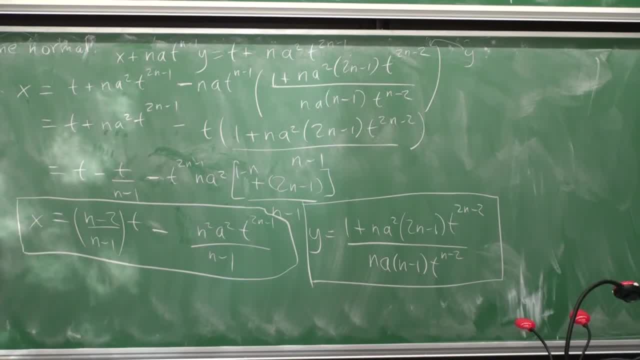 But- And it's easy, of course, to go wrong- All right, So you have to go slowly, Write neatly. Writing neatly is important, Giving yourself lots of room, Be patient. It actually doesn't take that long if you just go systematically, slowly, step by step. 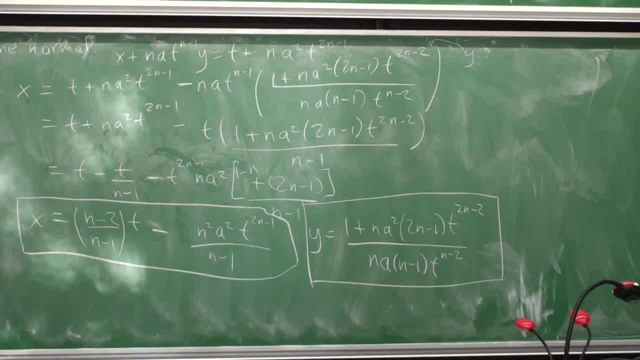 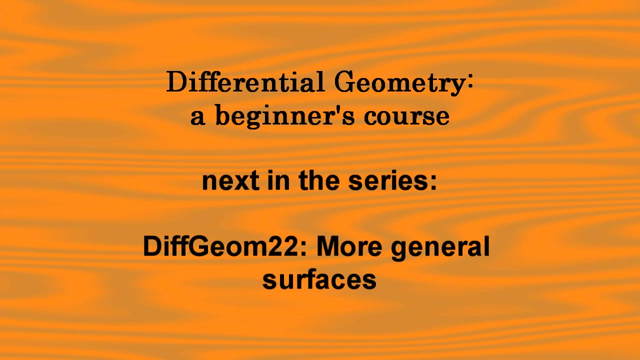